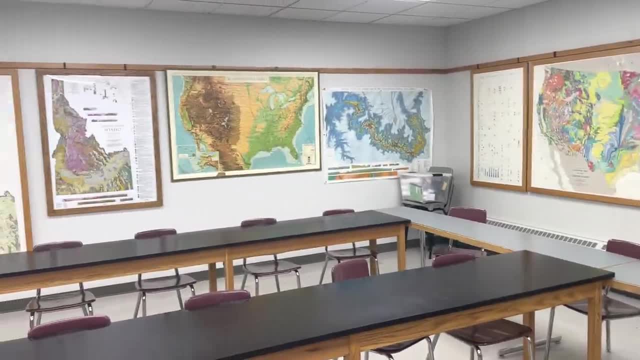 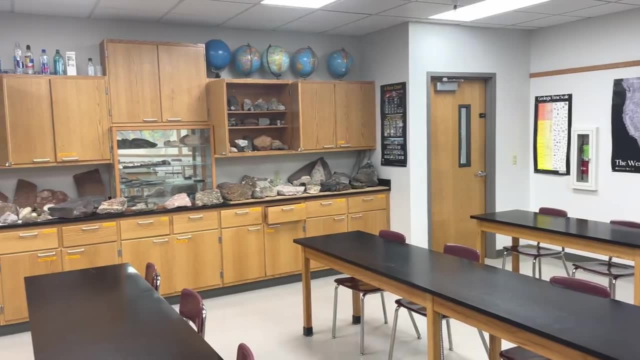 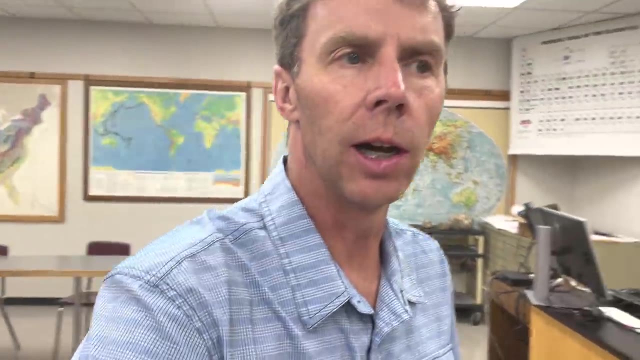 All right, friends. we are back here in the Evergreen building at the College of Southern Idaho, in my classroom here in Twin Falls cabinet full of rocks there- And we're gonna launch our new video on rocks and rock types- Still not sure what. 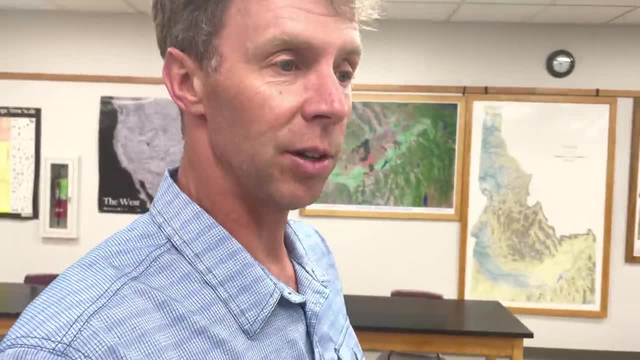 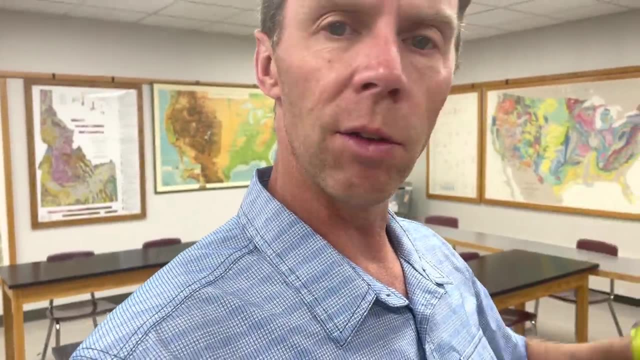 I'm gonna call it, but I'll come up with something, maybe creative, maybe just very pretty basic. But I thought we'd first kind of get into the rock cycle. an overview of the three major types of rocks. Some of you know this in detail. 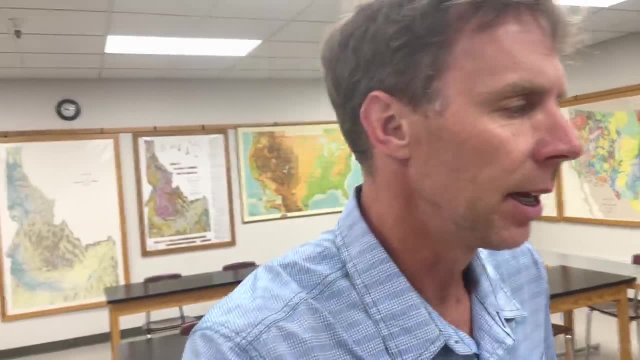 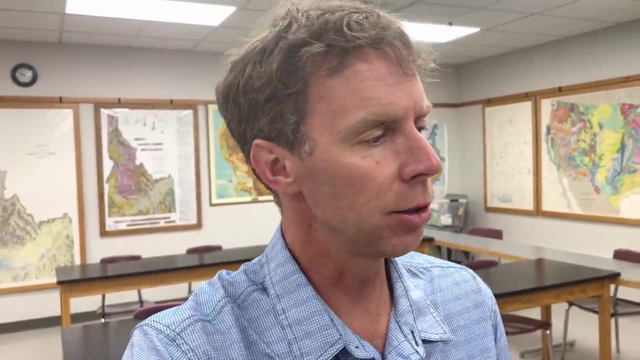 for others, you might be new. I'm gonna kind of cover this at a sort of an introductory level, but hopefully a very useful level. So I'm sure there's some of you that know way more about rocks than I do. They're gonna want more out of it. 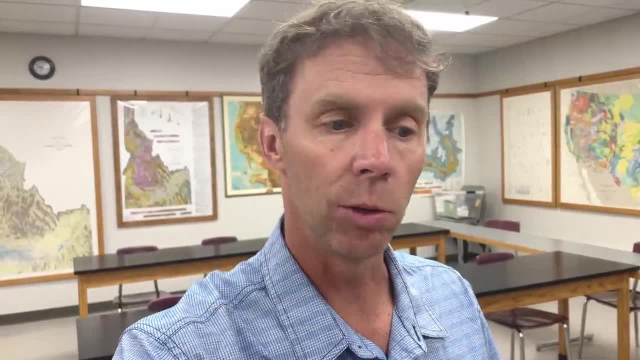 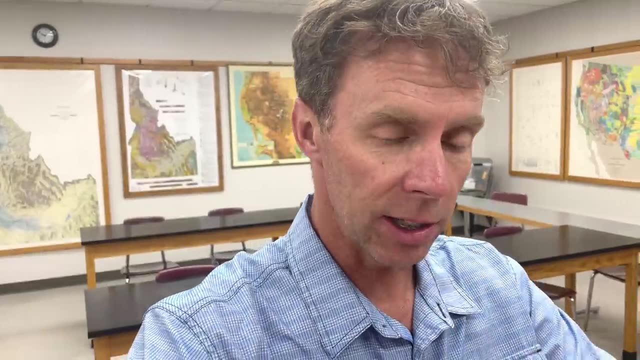 but I'm hoping to hit the majority of you with the content and the depth and depth that I cover these things. So we're gonna talk a little bit about the rock cycle. I've got some samples I want to show to you and then, I think, my idea. 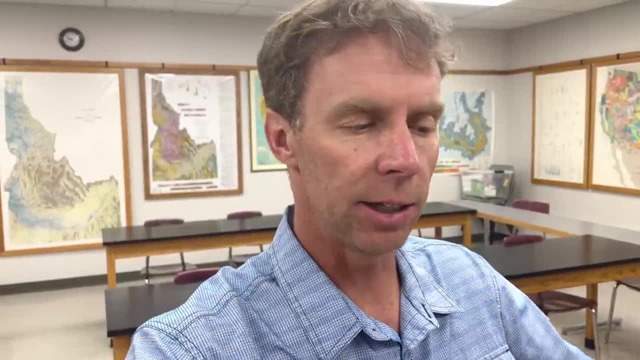 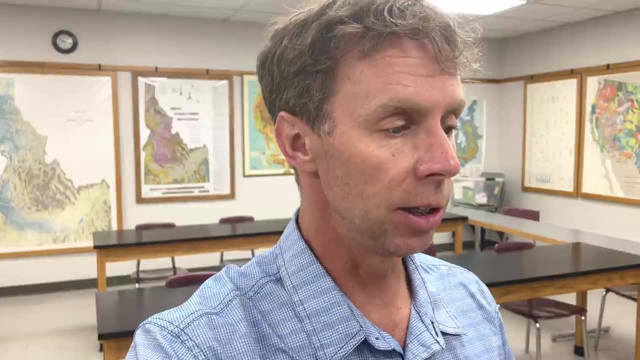 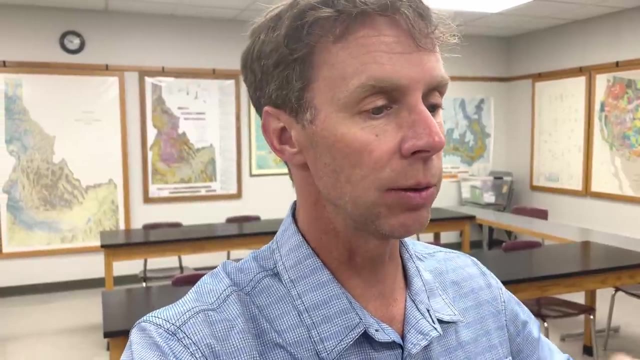 is to launch into each group of rocks, like the igneous rocks, and cover maybe just one rock, maybe several, to kind of give you some skills and some information, show you lots of different examples. And then the idea again is that as you're going out on your adventures and you're looking at rocks, you're able 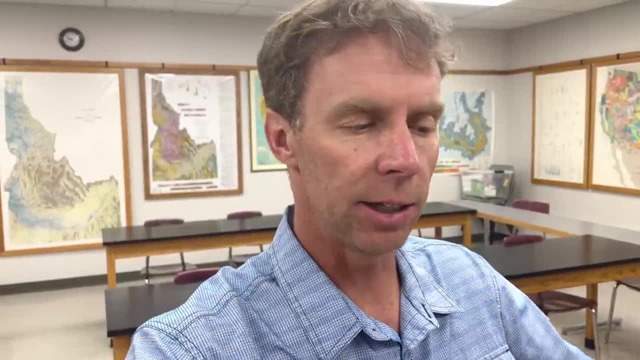 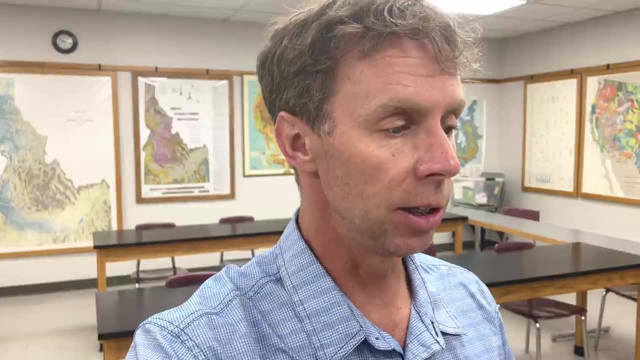 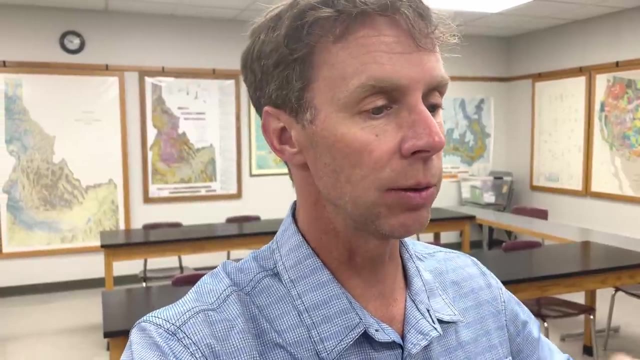 is to launch into each group of rocks, like the igneous rocks, and cover maybe just one rock, maybe several, to kind of give you some skills and some information, show you lots of different examples. And then the idea again is that as you're going out on your adventures and you're looking at rocks, you're able 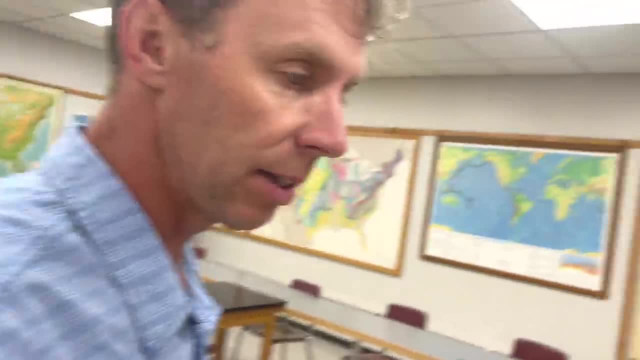 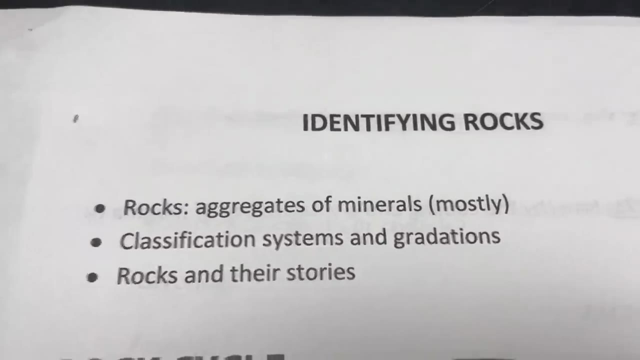 to figure them out a little bit better and make better identifications. So what we have here is identifying rocks- This is what we're gonna kind of start with here- and realize that rocks are just just aggregates of minerals. right, Just putting a bunch of minerals together. 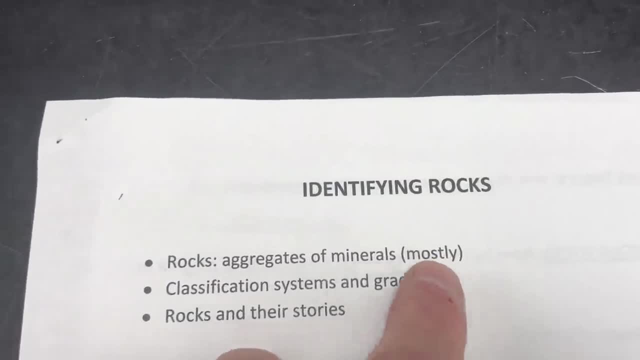 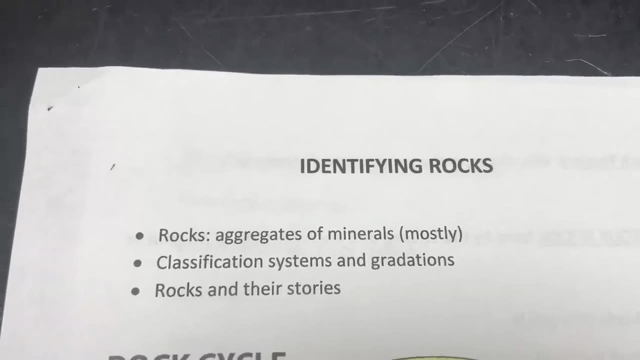 That's what a rock is, And I pull over here mostly because we do have a couple of rocks that sort of defy this description, and one in particular would be something like obsidian, which is actually made out of no minerals, because the elements are are not organized into rocks. So I'm gonna start off with the 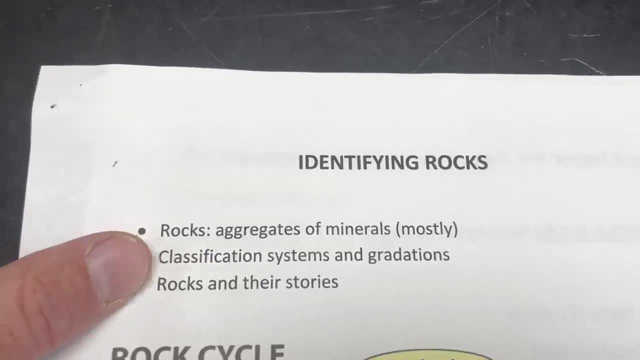 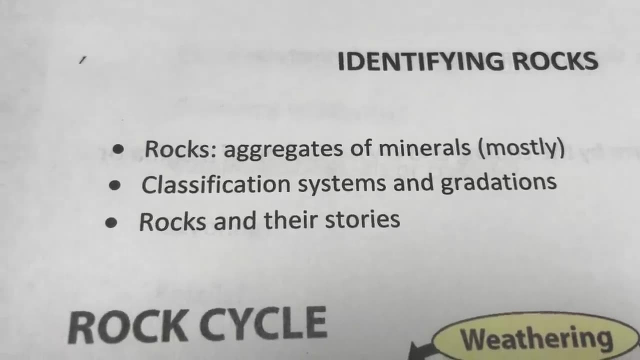 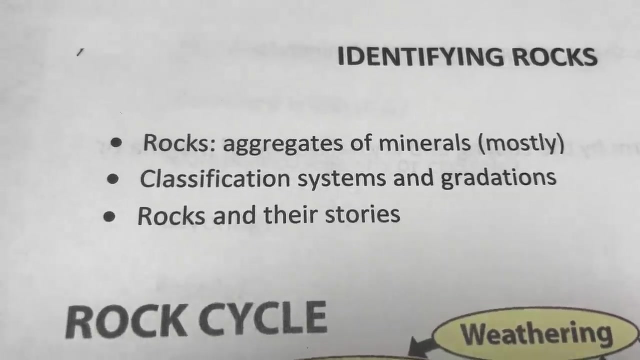 specific mineral crystals. Realize as we go through the classification systems here, the classification systems are just. it's just the way humans make sense of things, right? So we have how many types of music are out there, right? There's country, there's punk rock, there's bluegrass, there's, you know, jazz, all. 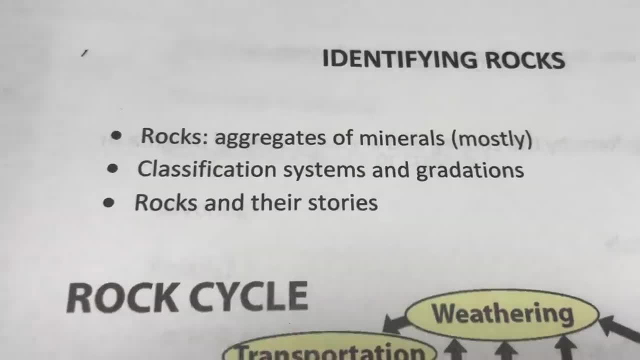 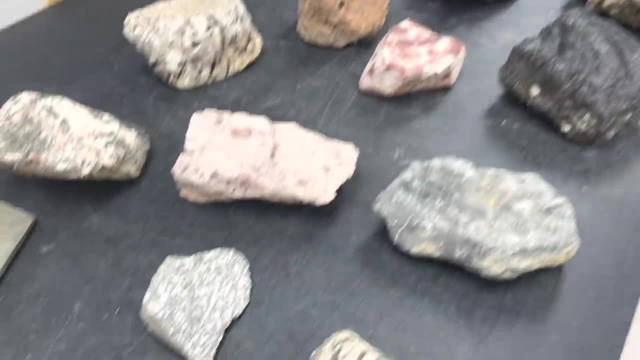 sorts of types of music, And this is just nothing more than our way of making sense of all the crazy rocks that exist out there in nature, And we'll kind of get to some of these here in a minute. So this is just our way humans like to have. 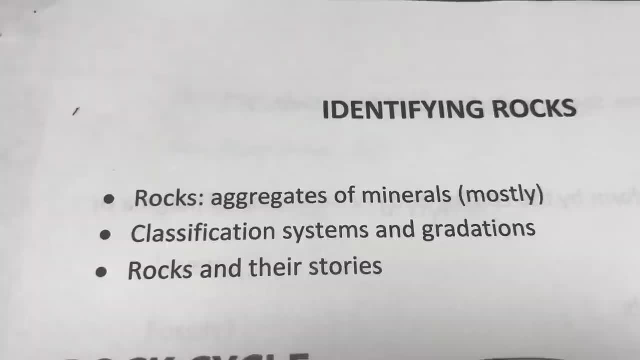 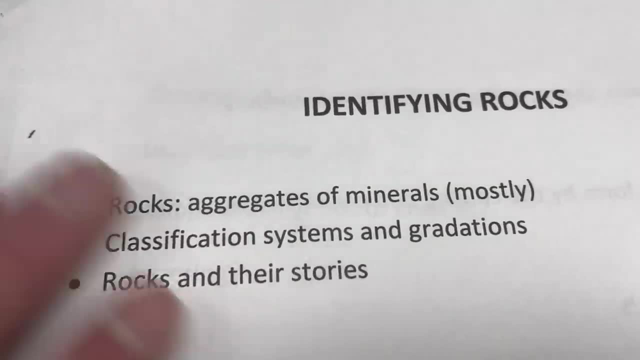 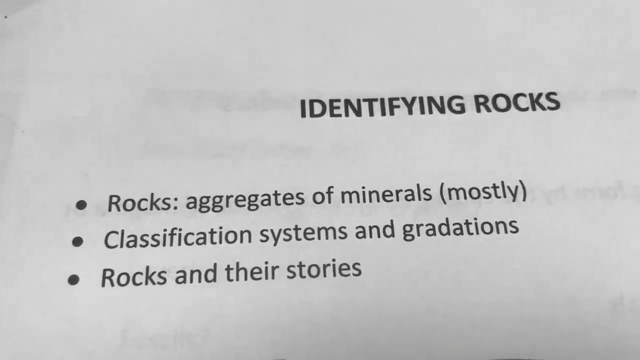 things classified. It helps us make sense of our world and some of the chaos and craziness and complexities that are out there, So realize that all classification systems are somewhat arbitrary and that they're also they're not perfect, right. So the way we classify rocks works pretty well, but it's not perfect. There's probably other. 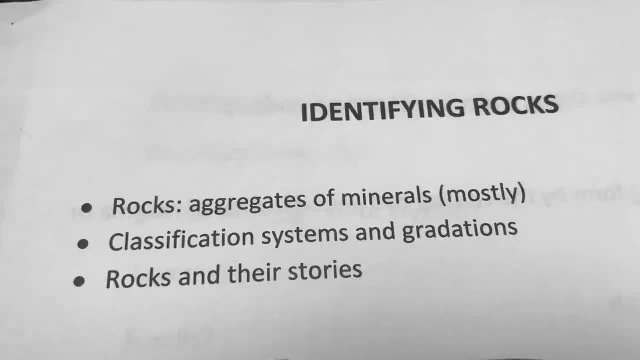 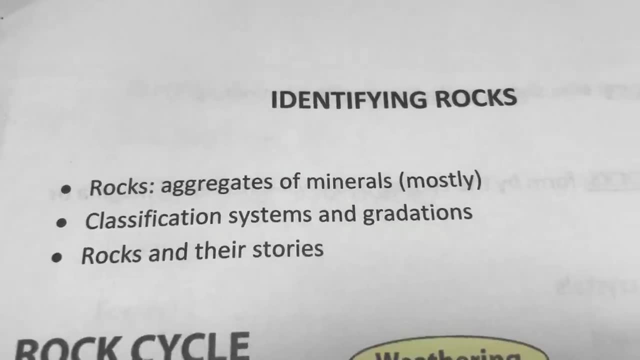 ways you might organize rocks. but this is pretty much stood the test of time so far and it seems to be a pretty good starting place to sort of organize rocks and provide some sort of organizational scheme. Realize that there's gradations as well. So if we 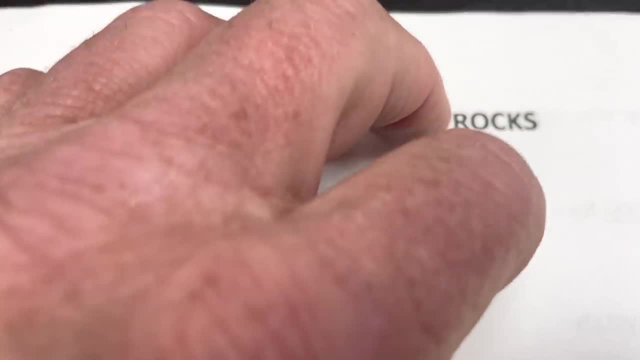 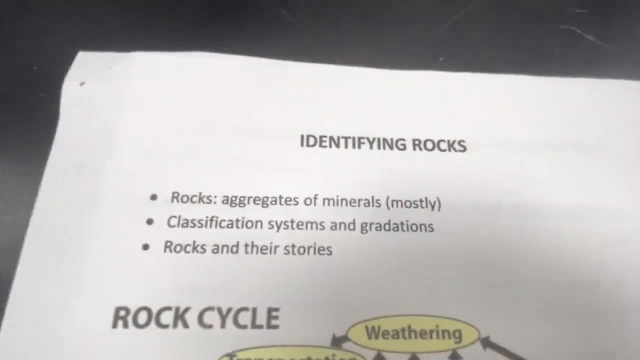 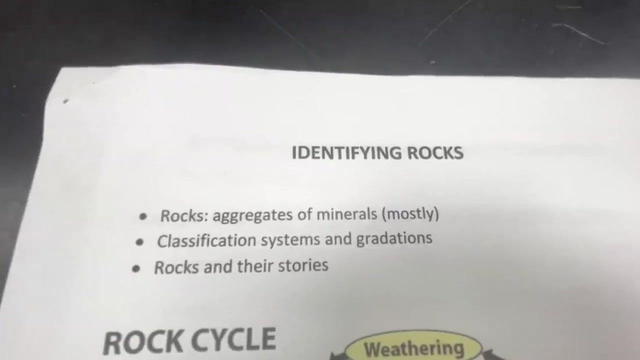 look at a rock like granite and then maybe another rock like diorite, realize that there's rocks that kind of fit in between there, And so there's always going to be something that might fit in between two unique rocks, And so the gradations are very possible. And then a big theme: 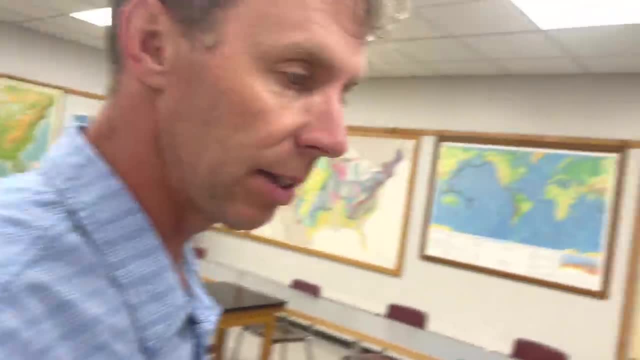 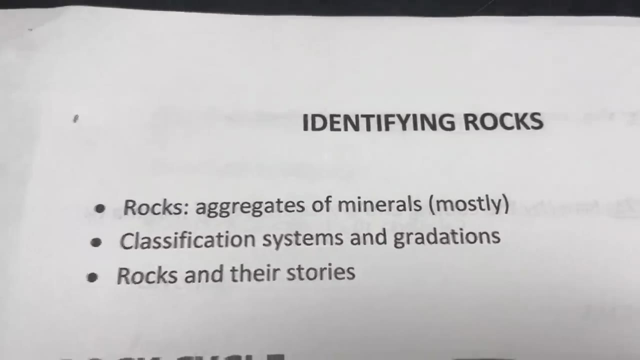 to figure them out a little bit better and make better identifications. So what we have here is so identifying rocks- this is what we're gonna kind of start with here- and realize that rocks are just just aggregates of minerals, right, Just putting a bunch of minerals together. 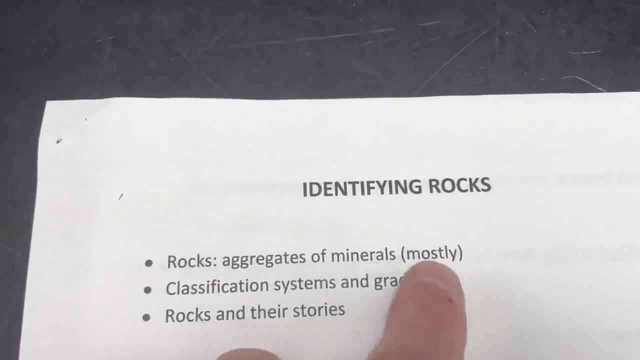 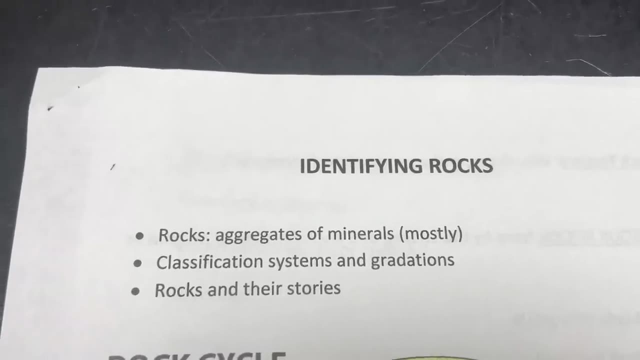 that's what a rock is, And I put over here mostly because we do have a couple of rocks that sort of defy this description, and one in particular would be something like obsidian, which is actually made out of no minerals, because the elements are are not organized into the rock cycle. So that's kind of what I'm going to talk about. 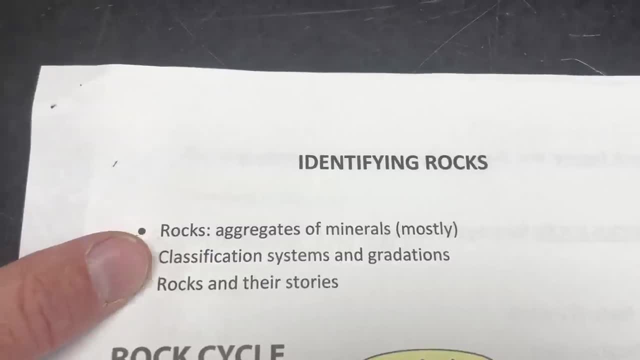 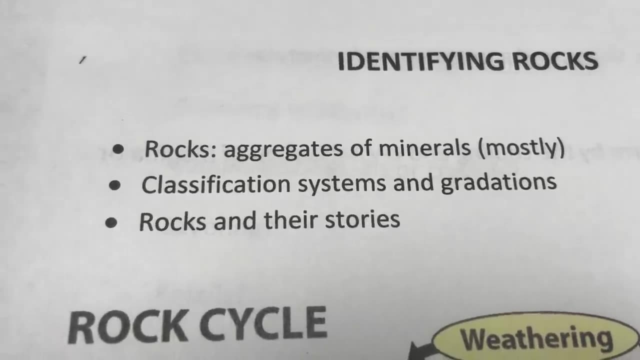 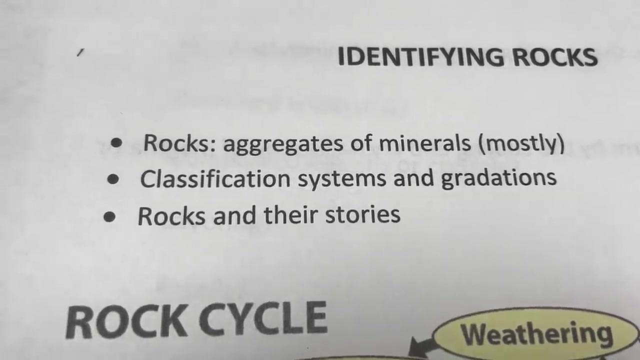 Realize as we go through the classification systems here. the classification systems are just. it's just the way humans make sense of things, right? So we have. how many types of music are out there? right, There's country, there's punk rock, there's bluegrass, there's, you know, jazz, all sorts of. 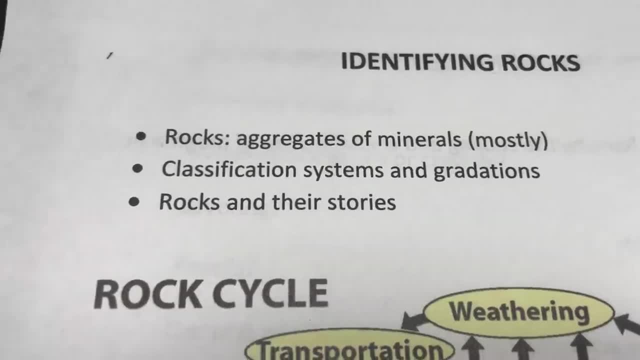 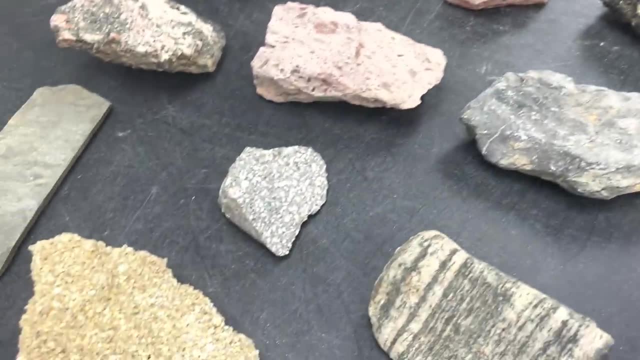 types of music, and this is just nothing more than our way of making sense of all the crazy rocks that exist out there in nature, And we'll kind of get to some of these here in a minute. So this is just our way humans like to have things. 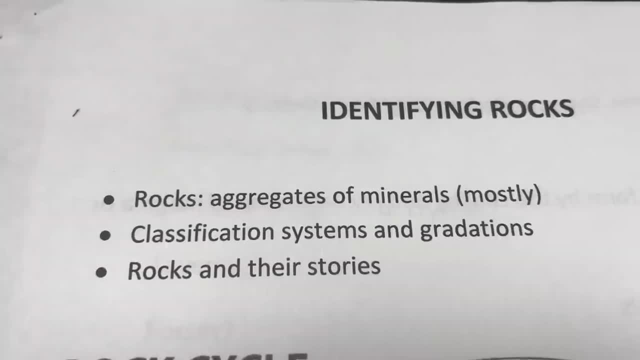 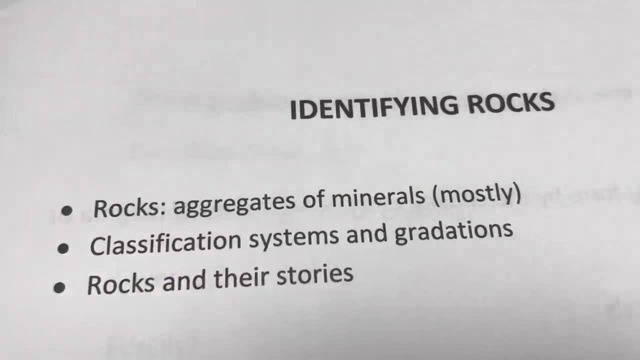 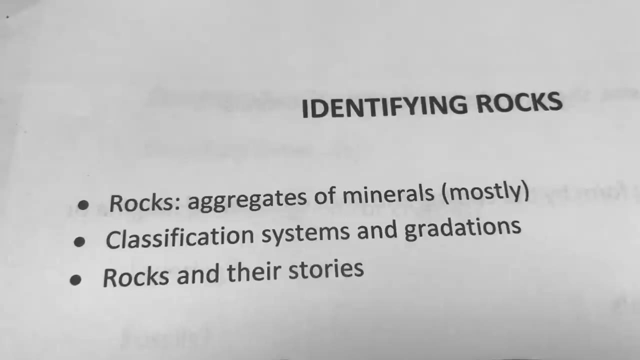 classified. It helps us make sense of our world and some of the chaos and craziness and complexities that are out there, So realize that all classification systems are somewhat arbitrary and that they're also they're not perfect, right. So the way we classify rocks works pretty well, but it's not perfect. There's probably other. 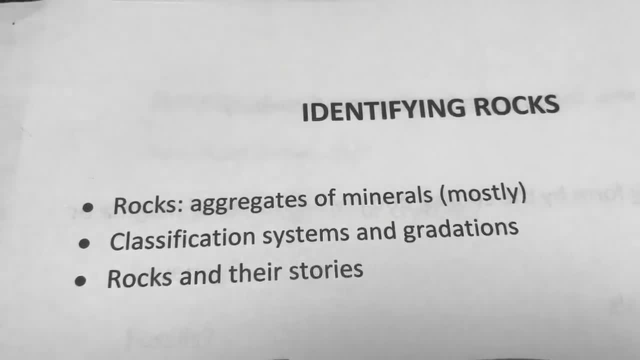 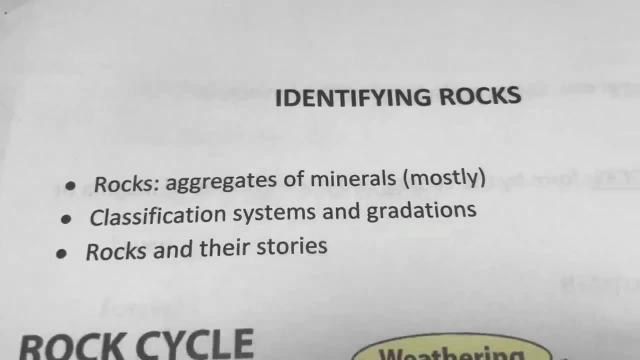 ways you might organize rocks. but this is pretty much stood the test of time so far and it seems to be a pretty good starting place to sort of organize rocks and provide some sort of organizational scheme. Realize that there's gradations as well. So if we look at a rock, 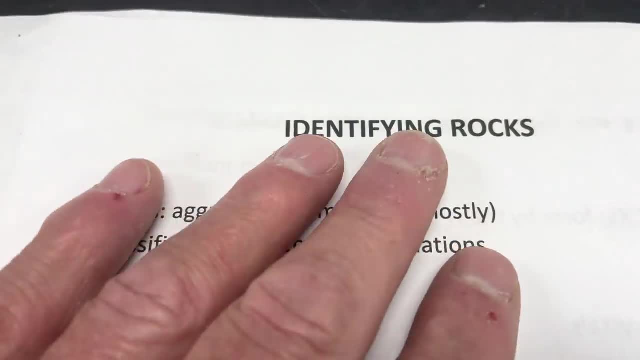 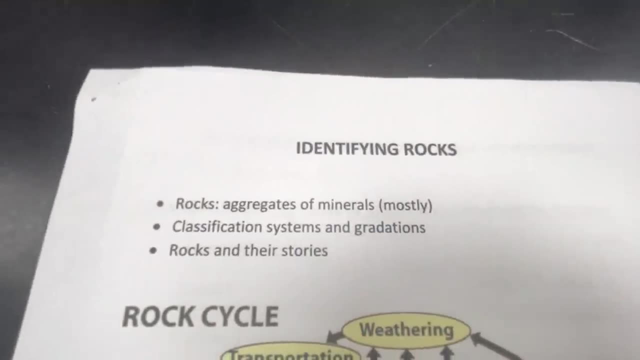 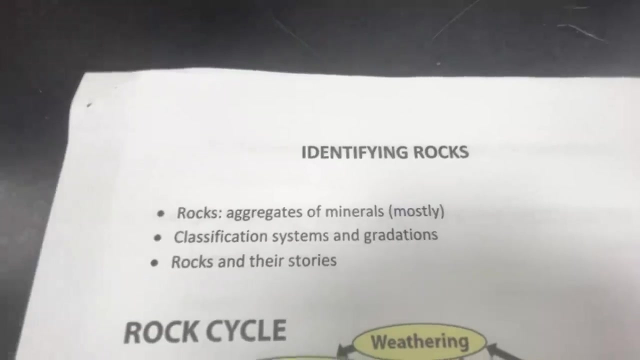 like granite, and then maybe another rock like diorite, realize that there's rocks that kind of fit in between there, And so there's always going to be something that might fit in between two unique rocks, And so the gradations are very possible. And then, a big theme that I 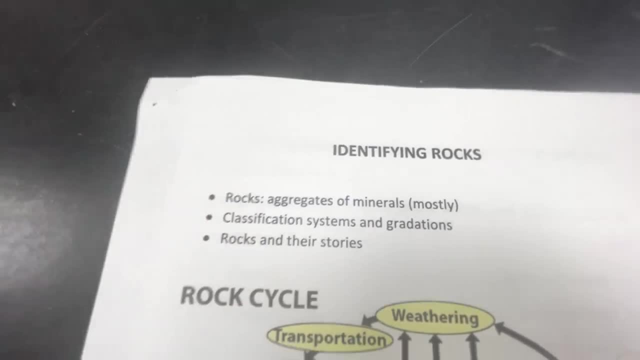 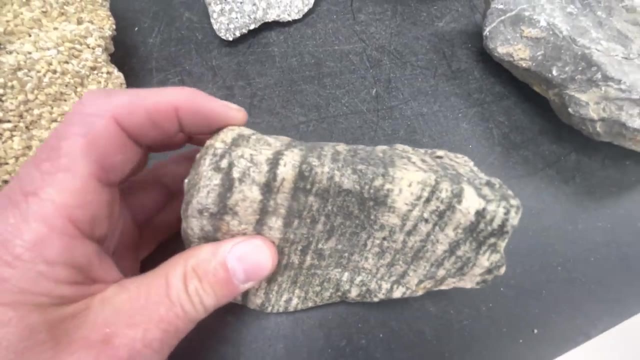 want to cover with this series is not just identifying the rocks. I think it's great to look at a rock like this and know that it's a metamorphic rock called nice, And if you can run around your town and out on your hiking trails. 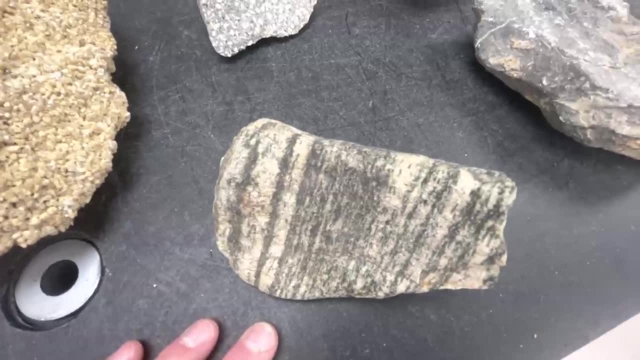 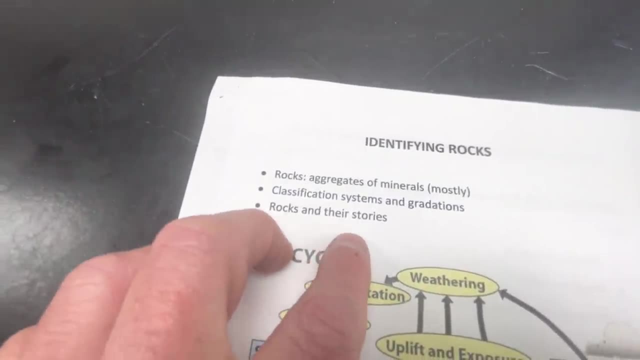 and be the smart person on the trail that can identify all the rocks. I think that's great, But for me and when I teach with my students, I'm really more interested in the stories. Can you, can you not only come up with the name, but can you really tell us what? what's happened to the? 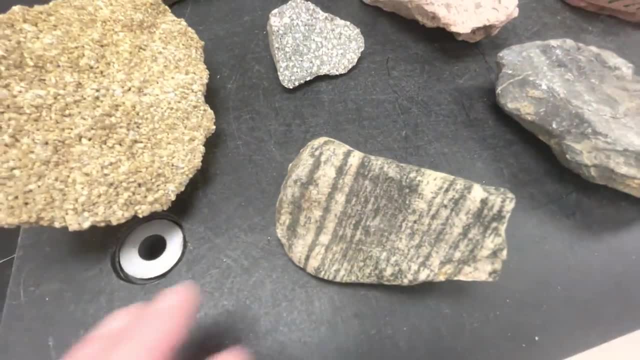 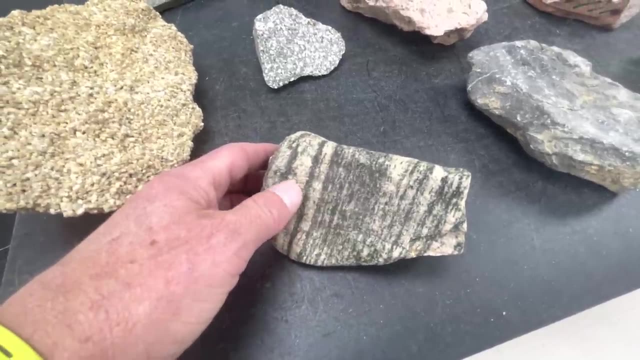 rock. What's actually formed these lines here in this metamorphic nice? What's the story of this rock? What conditions, what environment did it form in? And to me, that's where the real power is is interpreting the stories. And I tell my students all the time that you know you're. 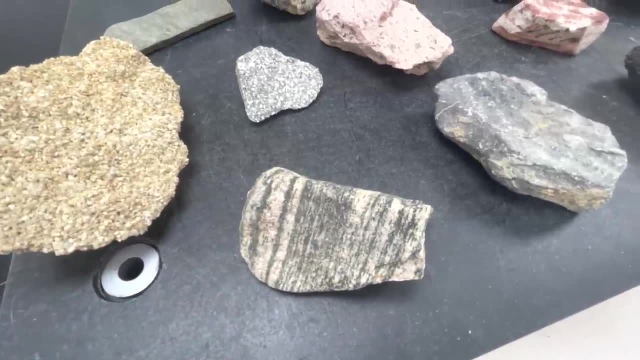 probably going to forget a lot of the names of the rocks. I'd rather have you be able to explain it. I'd rather have you tell someone in 10,, 20 years when you're on a camping trip: oh, this rock. 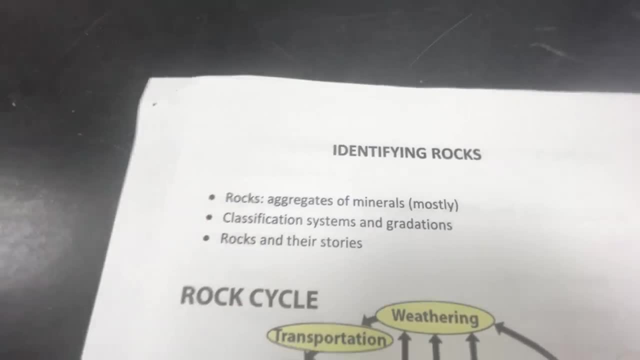 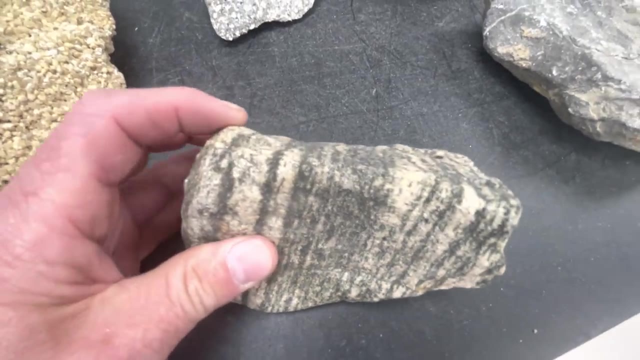 I want to cover with this series is not just identifying the rocks. I think it's great to look at a rock like this and know that it's a metamorphic rock called nice, And if you can run around your town and out on your hiking trails and be the smart person on the trail. 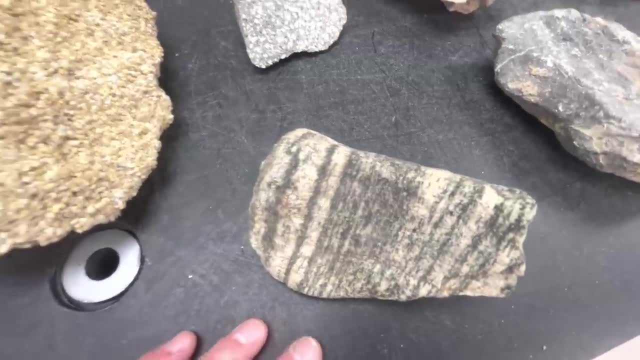 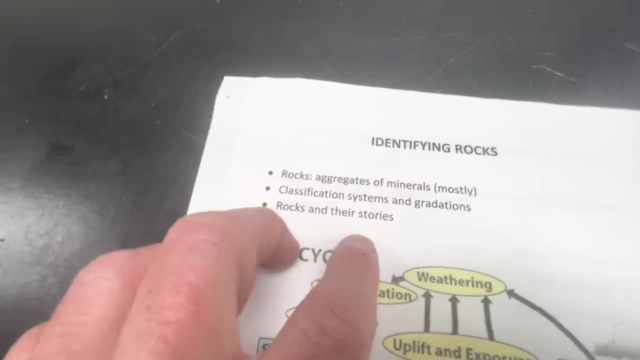 that can identify all the rocks. I think that's great, But for me and when I teach with my students, I'm really more interested in the stories. Can you not only come up with the name, but can you really tell us what's happened to this rock? Can you tell us what's happened to this rock? 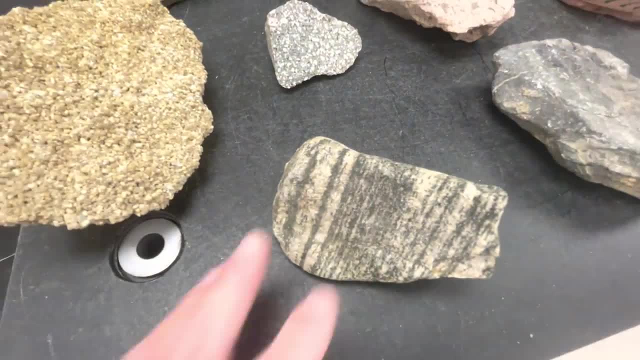 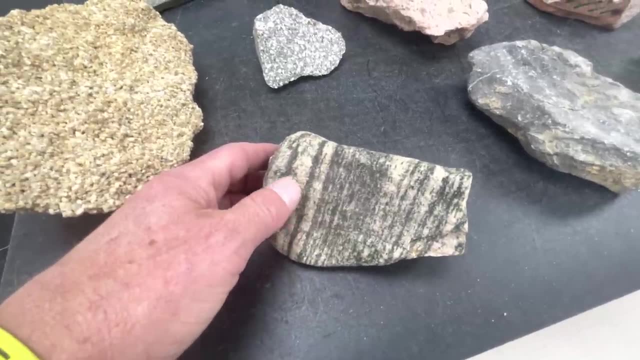 What's actually formed these lines here, in this metamorphic nice? What's the story of this rock? What conditions, what environment did it form in? And to me, that's where the real power is is interpreting the stories, And I tell my students all the time that you know. 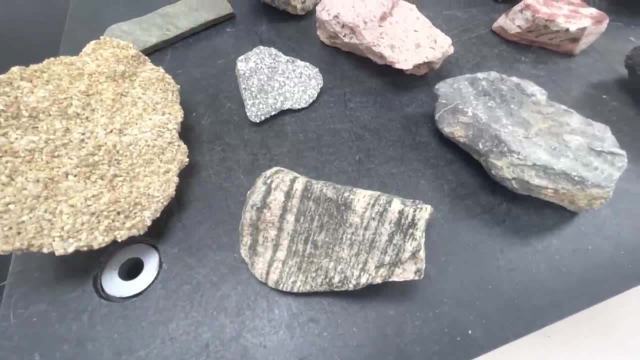 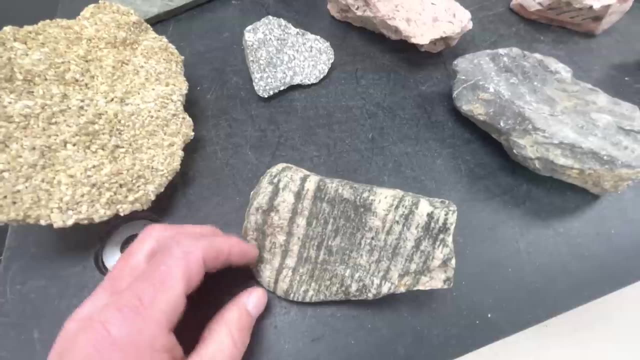 you're probably going to forget a lot of the names of the rocks. I'd rather have you be able to explain it. I'd rather have you tell someone in 10,, 20 years when you're on a camping trip: oh, this rock, I think it's a metamorphic rock. I can't remember the name, but I think it has. 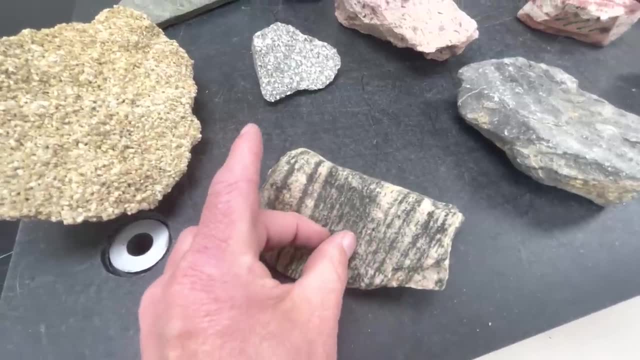 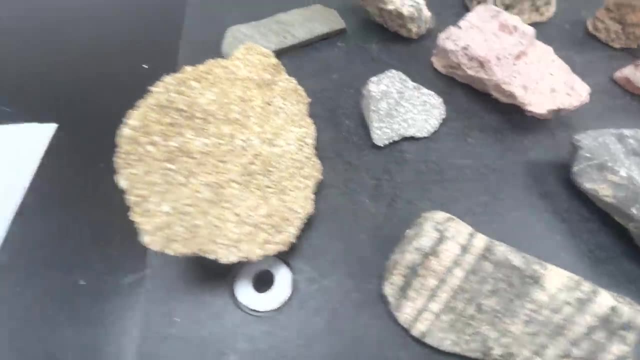 these lines in it because it was squeezed in this direction. Very high temperatures and pressures caused it to deform, And that's why the minerals are aligned in this manner. To me, I think that's much more powerful than just regurgitating a name. but that's just me. Let's look at the rock cycle. 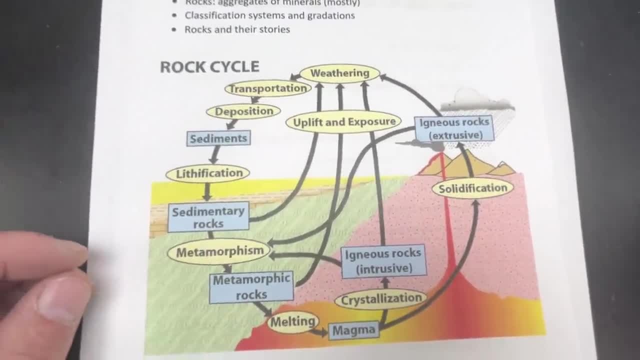 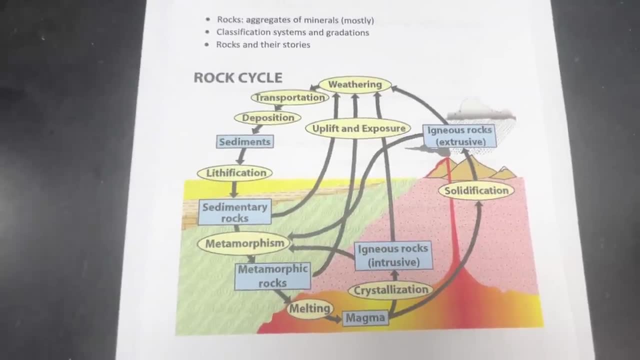 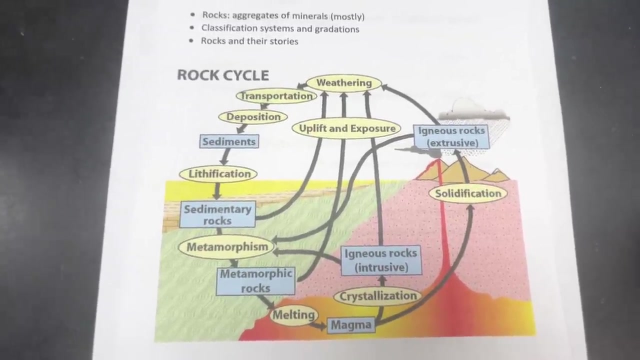 Again, this is something you've probably seen before, but just to make sure we're all on the same page. So this is just a nice diagram and a handy way to think about rocks, because rocks are transient entities. They're changing location Over time. they're changing the environment in which they reside in over time. So if we start, 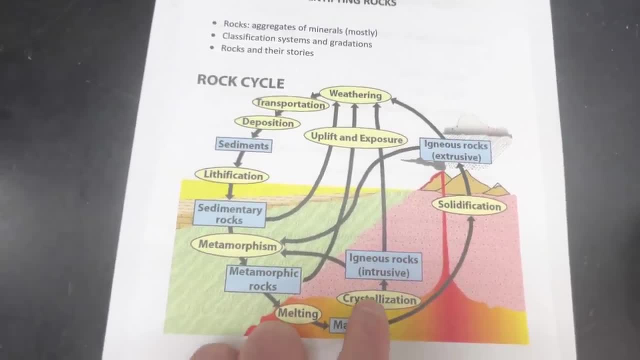 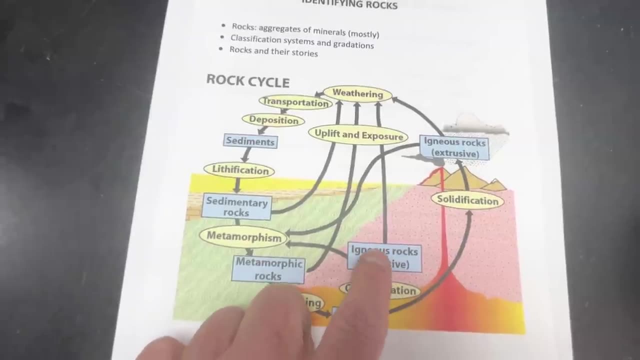 with something like magma and it crystallizes. the crystalizes underground, below the earth's surface. that's what we call an intrusive igneous rock. So this is magma cooling and crystallizing slowly under the earth's surface. This might be something like granite. That's one possible rock. 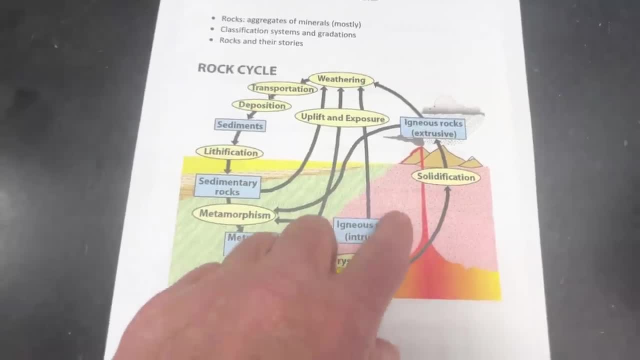 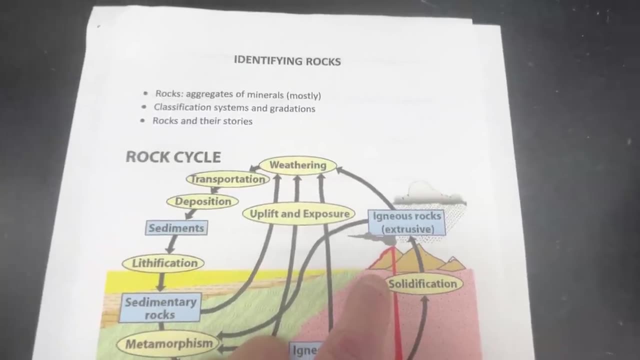 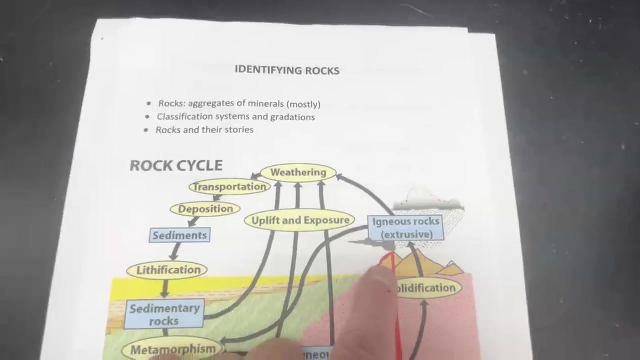 that would result from magma crystallizing. Magmas, though, might make their way all the way to the surface. expelled to the surface through some type of volcanic eruption, It might be explosive. It might be less explosive, but that would be an extrusive igneous rock. But when that lava or ash, 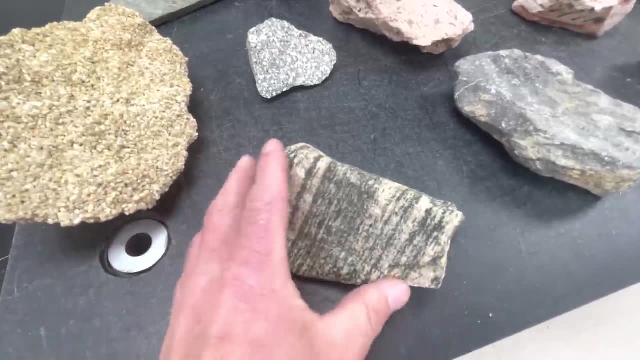 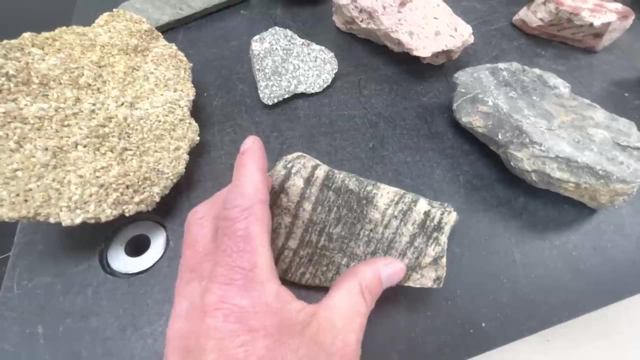 I think it's a metamorphic rock- I can't remember the name, but I think it has the lines in it- because it was squeezed in this direction. Very high temperatures and pressures caused it to deform, And that's why the minerals are aligned in this manner. To me, I think that's. 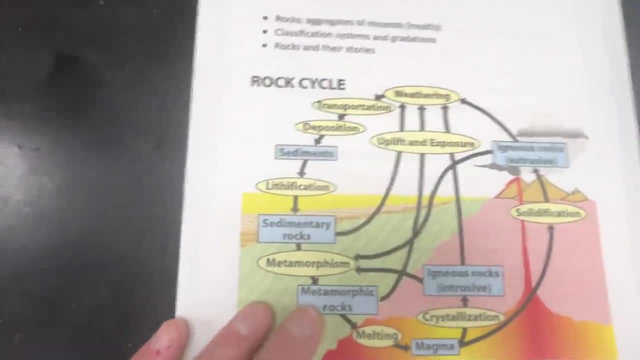 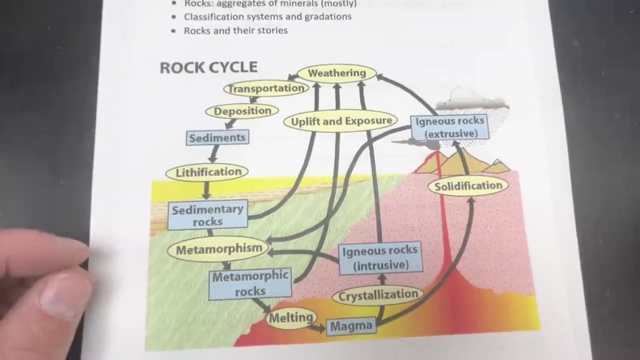 much more powerful than just regurgitating a name. but that's just me. Let's look at the rock cycle Again. this is something you've probably seen before, but just to make sure we're all on the same page. So this is just a nice diagram and a handy way to think about rocks, because rocks are. 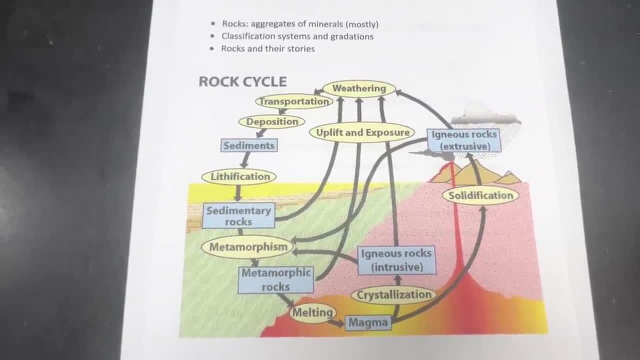 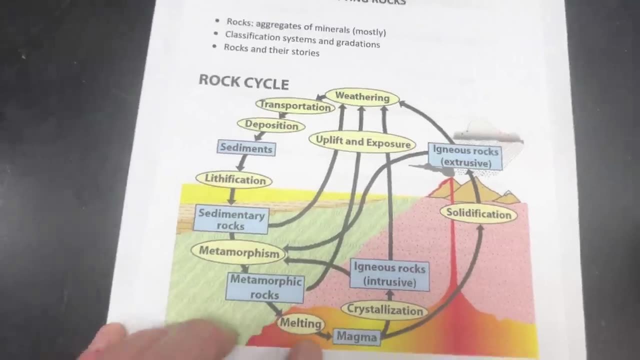 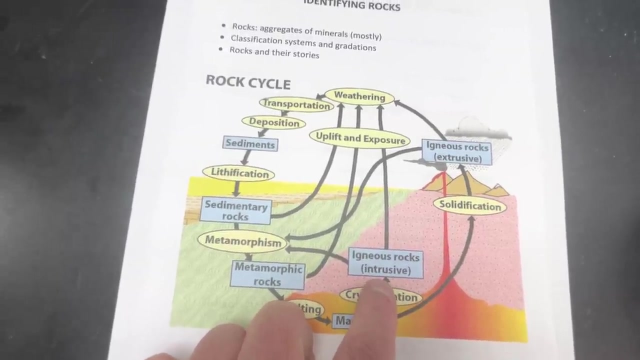 transient entities. They're changing location Over time. they're changing the environment in which they reside in over time. So if we start with something like magma and it crystallizes, the crystallizes underground, below the earth's surface. that's what we call an intrusive igneous rock. So this is magma cooling. 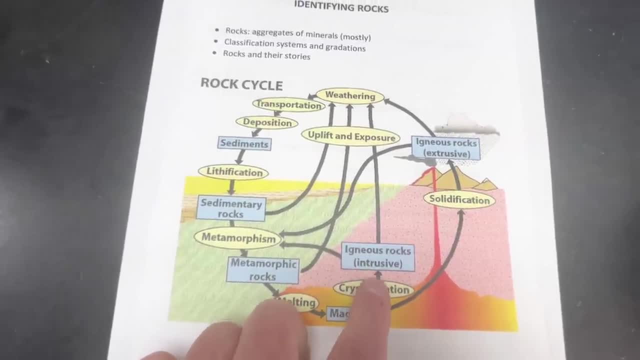 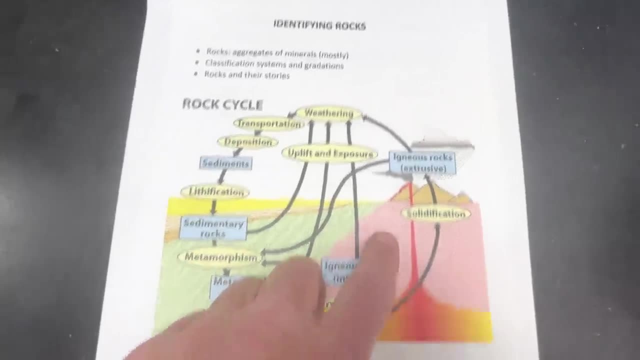 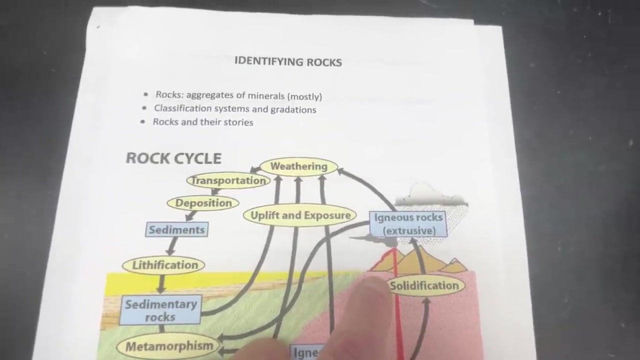 and crystallizing slowly under the earth's surface. This might be something like granite, That's one possible rock that would result from magma. crystallizing. Magmas, though, might make their way all the way to the surface, where they are expelled to the surface through some type of volcanic eruption. It might be explosive. 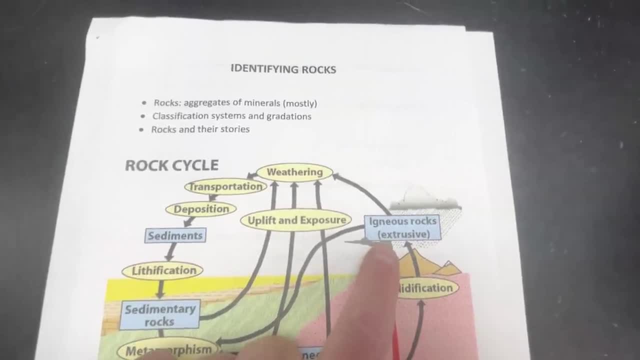 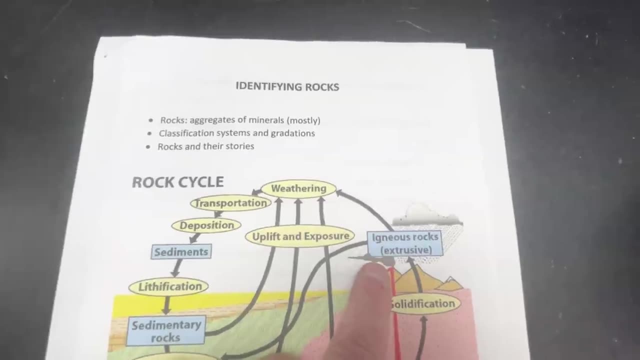 it might be less explosive, but that would be an extrusive igneous rock. But when that lava or ash or whatever the volcanic material is, cools and crystallizes, that will form an igneous rock at the surface. So we have igneous rocks in two different environments. we'll obviously spend 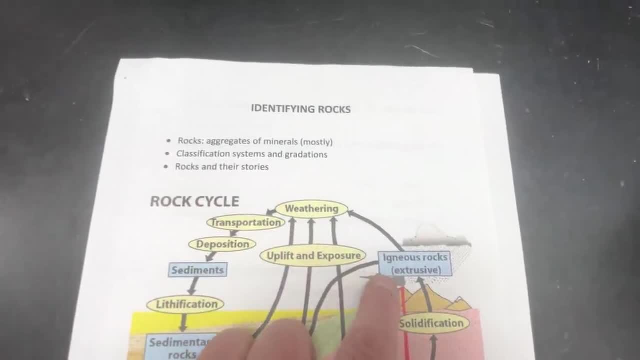 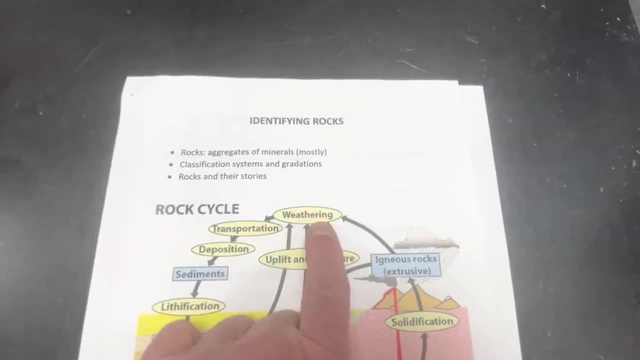 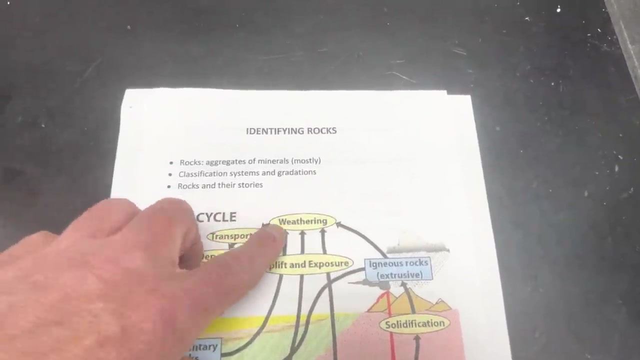 some time on those. Once we have any rock at the surface, be it igneous or any other type of rock, it's exposed to weathering. the wind, the, the glaciers, the wave, action in the, in the ocean streams- all sorts of different processes conspire to break the rock into smaller pieces. that's what weathering is: breaking the rock. 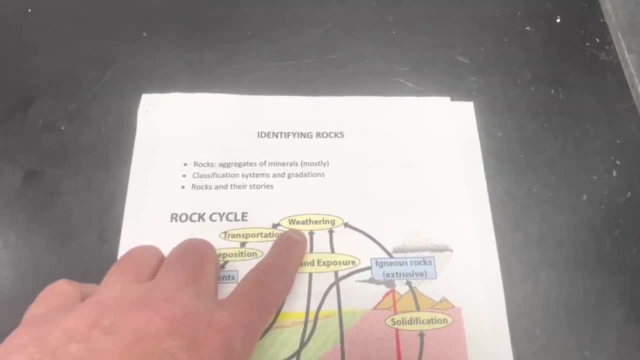 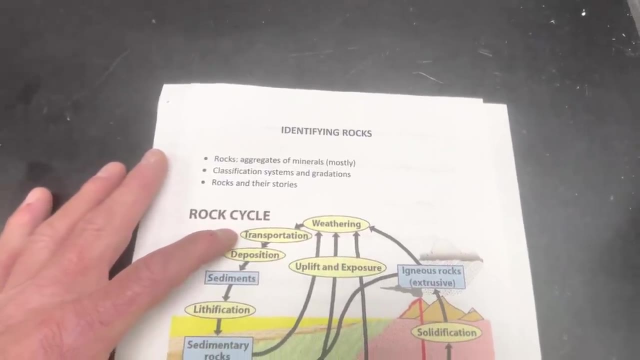 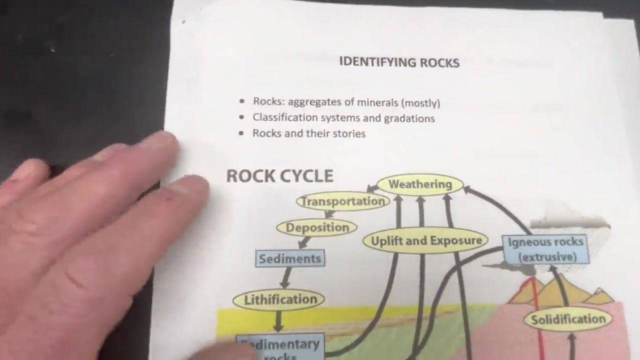 into pieces. once the pieces are small enough that they can be effectively moved, we call that just transportation. sometimes we also call this erosion, when we're actually moving the particles. eventually you run out of energy to move the particles and so those particles come to rest somewhere and that's known as deposition. so we're depositing layers of weathered rock in some 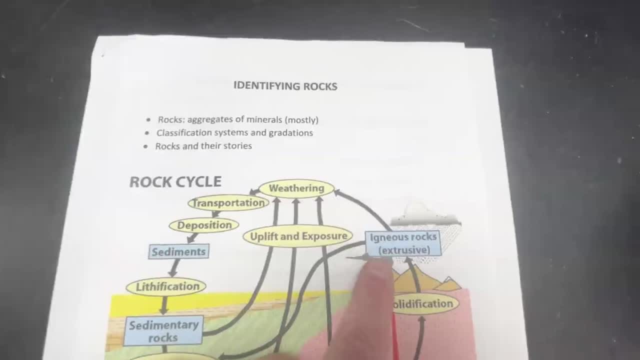 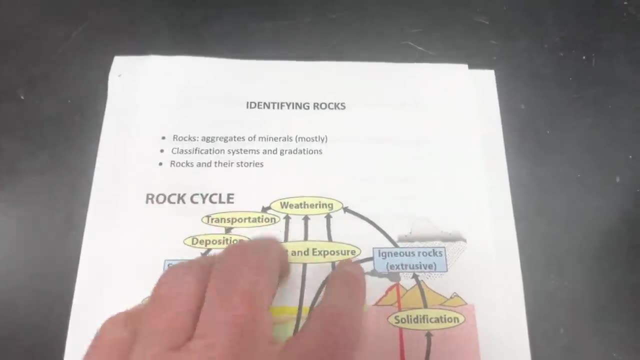 or whatever the volcanic material is, cools and crystallizes, that will form an igneous rock at the surface. So we have igneous rocks in two different environments. We'll obviously spend some time on those. Once we have any rock at the surface, be it igneous or any other type of rock, 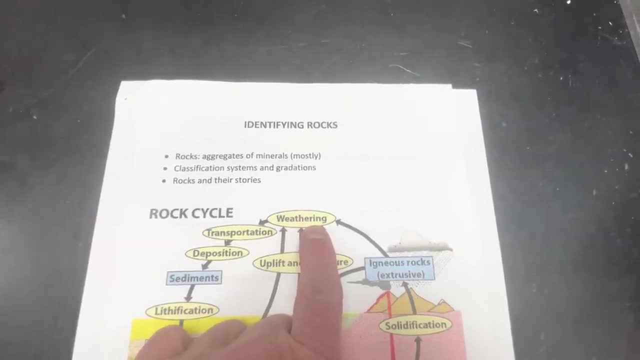 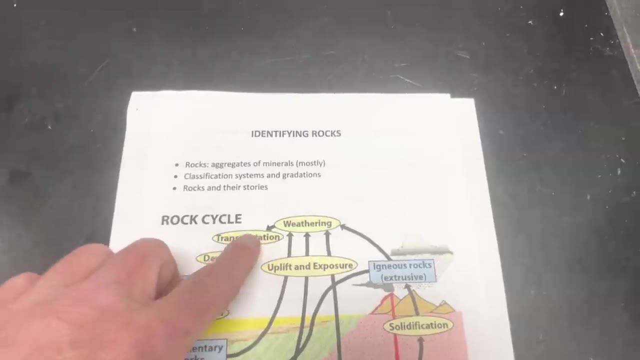 at the bottom of the ocean that will blow up. As you can see, we have very, very small rocks as we enter the ocean, But we also do have very, very small particles at the bottom of the ocean that will move and then go down into the ocean, and we have very, very small surfaces. So we want to 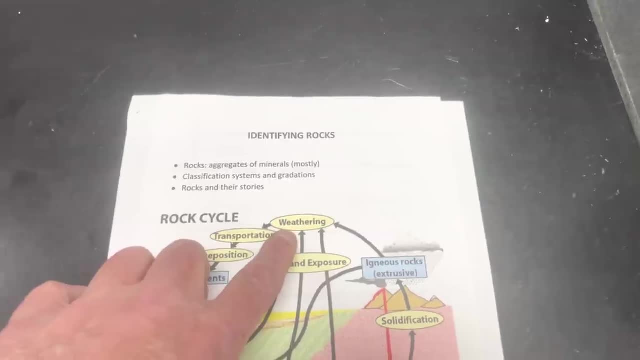 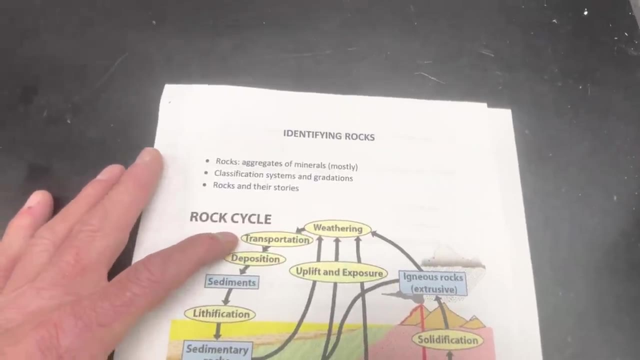 have very, very small particles, because if they move it will be very difficult to collect. But as we go through this a little bit more, we're going to draw a line between the rocks, the ocean rocks, the magma and the crystalization igneous rock. So this is really a very, very 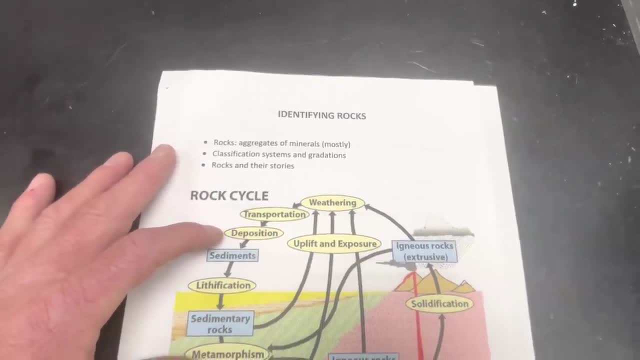 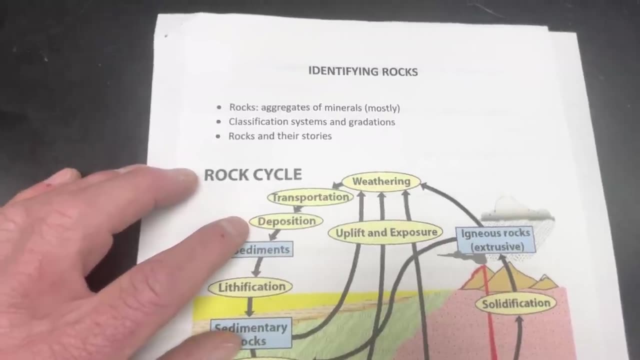 tight line between the rocks and the wind. So while we're trying to write that now, this is a very come to rest somewhere and that's known as deposition. so we're depositing layers of weathered rock in some environment and those become sediments. those 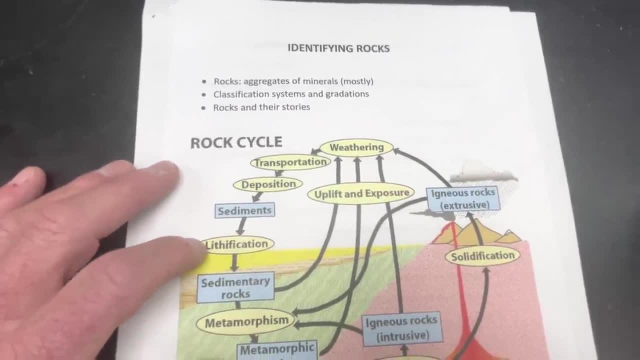 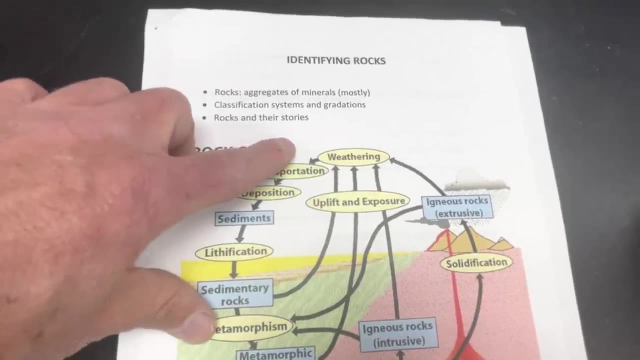 sediments can then get buried deep enough that they are compressed and cemented together- that's what we call lithification- to form a sedimentary rock. so sedimentary rock would be rocks that have weathered, or material that's weathered out of rocks and been compacted could be fossils as well. 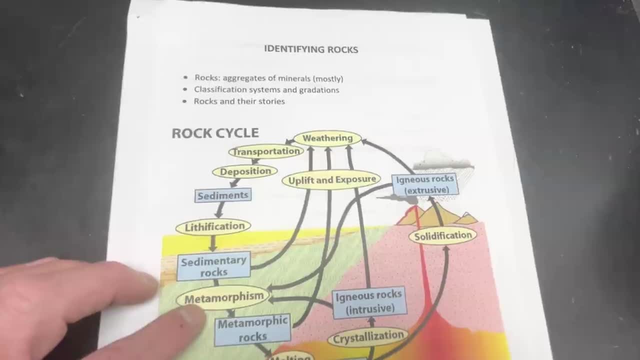 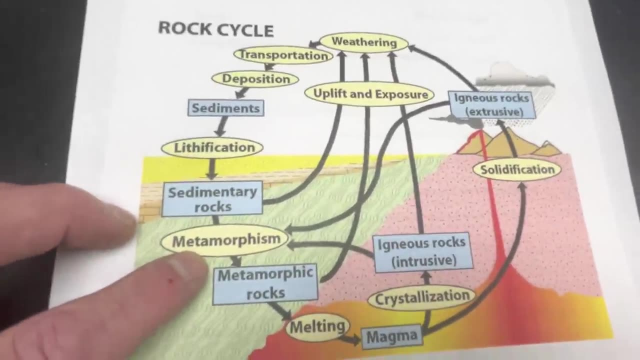 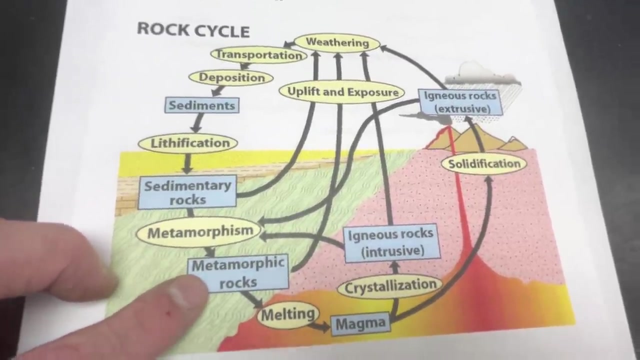 organic material any rock can be. if it's buried deep enough, the temperatures and pressures will be high enough. that will have a change in the rock, a solid state change, and that's what we call metamorphism. heat and pressure have changed the rocks into some new type of rock that we call metamorphic rocks. if 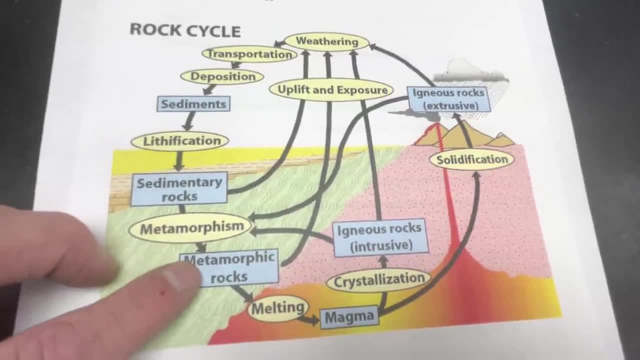 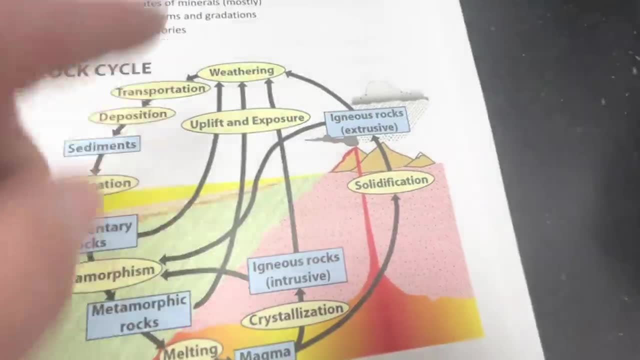 we keep heating the rocks up beyond this metamorphic realm here we may eventually start melting the rocks again and then we're back to magma. so realize, yes, it's one nice big circle. but also people with metamorphism are actually going to have to realize and notice that 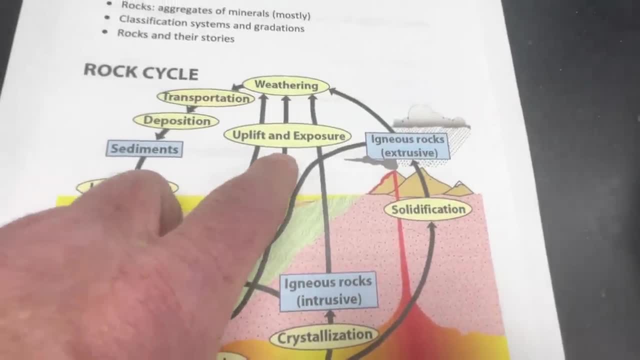 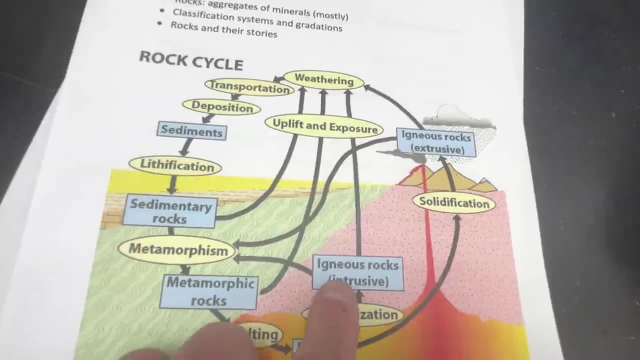 there's lots of little shortcuts. metamorphic rocks might be pushed up by mountain-building events. they might be uplifted, exposed, they become weathered. then they can turn back into sedimentary rocks at any point in the game. a rock might be buried deep enough that it becomes metamorphose, and so there's all. 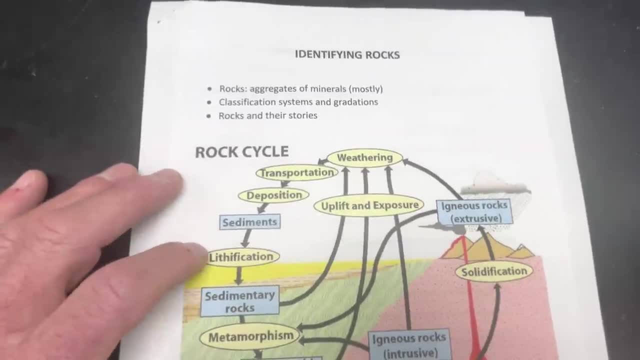 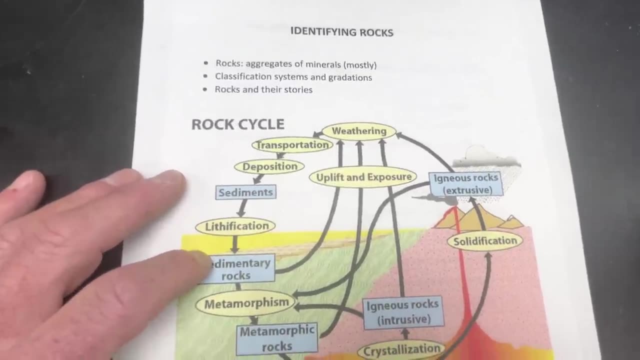 environment and those become sediments. those sediments can then get buried deep enough that they are compressed and cemented together- that's what we call lithification- to form a sedimentary rock. so sedimentary rock would be rocks that have weathered, or material that's weathered out of rocks. 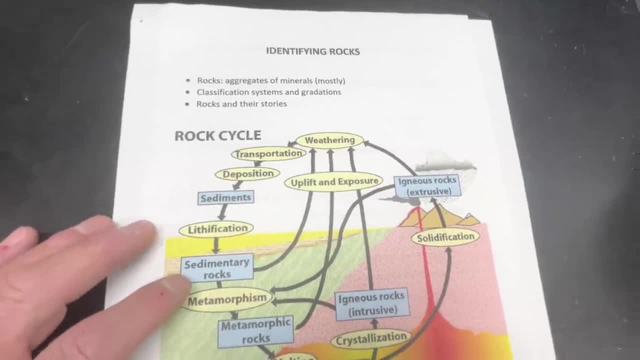 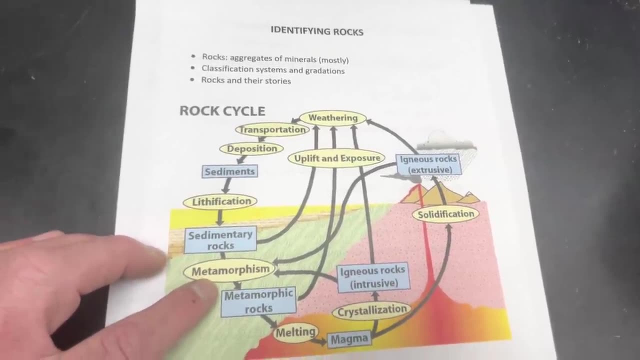 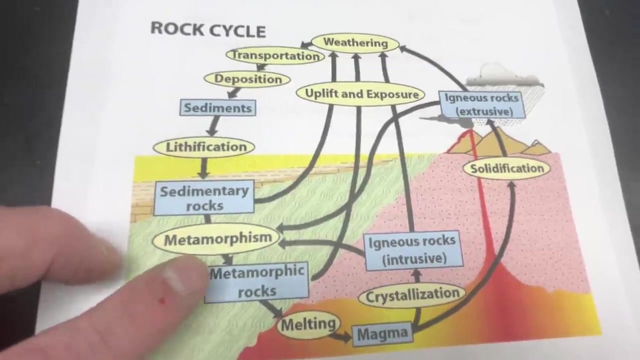 and been compacted, could be fossils as well organic material, um any rock can be. if it's buried deep enough, the temperatures and pressures will be high enough that we'll have a change in the rock, a solid state change, and that's what we call metamorphism. heat and pressure have changed the rocks into some. 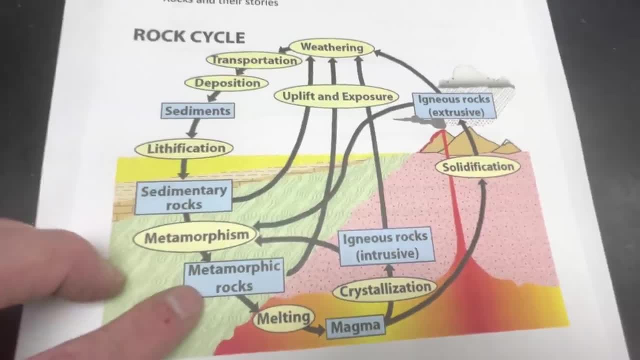 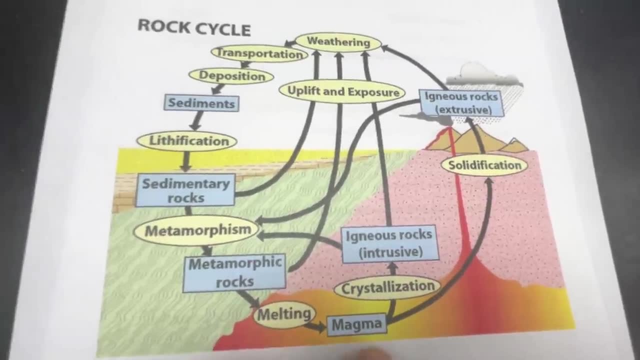 new type of rock that we call metamorphic rocks. if we keep heating the rocks up beyond this metamorphic realm here, we may eventually start melting the rocks again and then we're back to magma. so realize, yes, it's one nice big circle, but if we keep heating the rocks up, we're going to 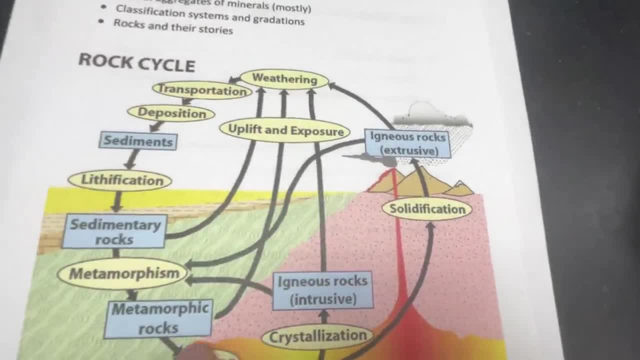 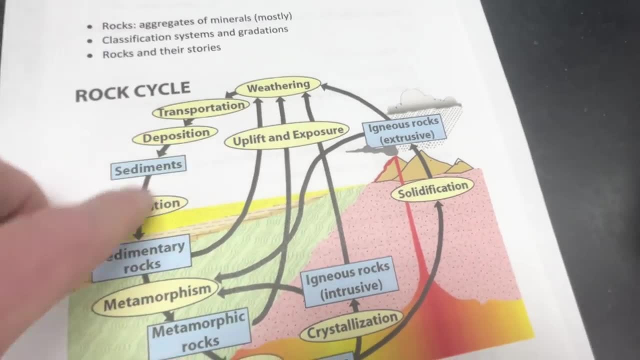 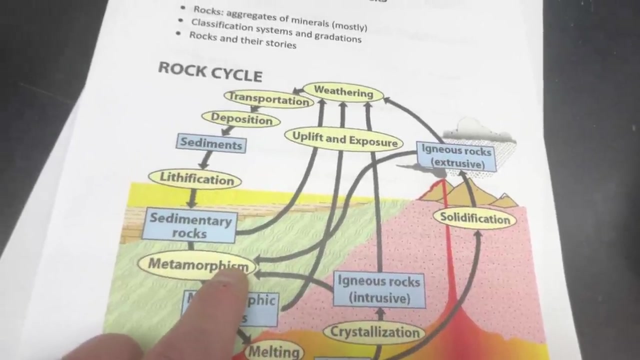 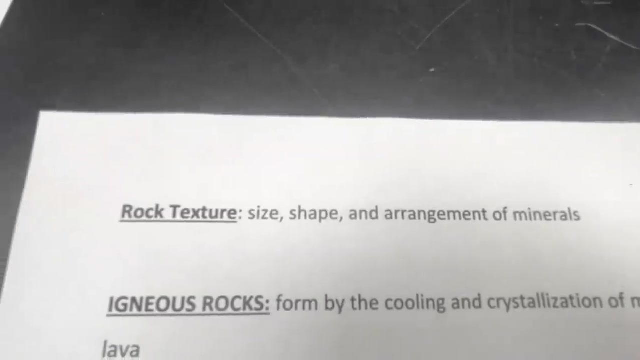 start melting the rocks again, and then we're back to magma. so realize, yes, it's one nice big circle. but also realize and notice that there's lots of little shortcuts. metamorphic rocks might be pushed up by mountain building events. they might be uplifted, exposed, they become weathered. then they can turn back into sedimentary rocks at any point in the game. a rock might be buried deep enough that it becomes metamorphosed, and so there's all sorts of shortcuts there. so that's the rock cycle. um, so when we look at rocks, what do we? what are some of the main things we're looking for? well, we're looking at the texture of the rock. now, that's sometimes. that could be like a little bit of a. 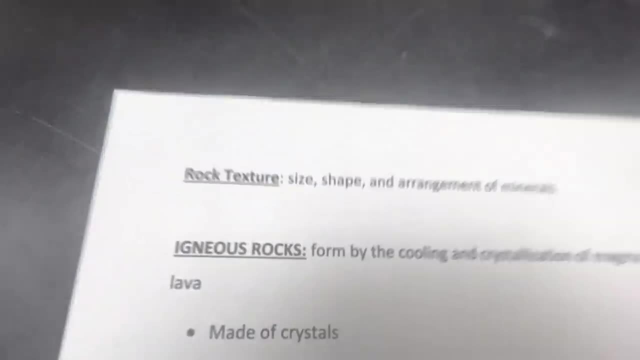 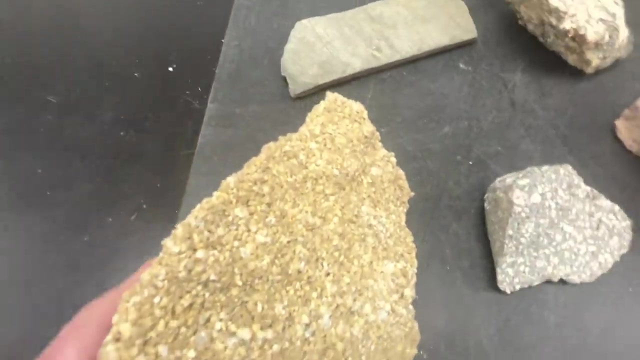 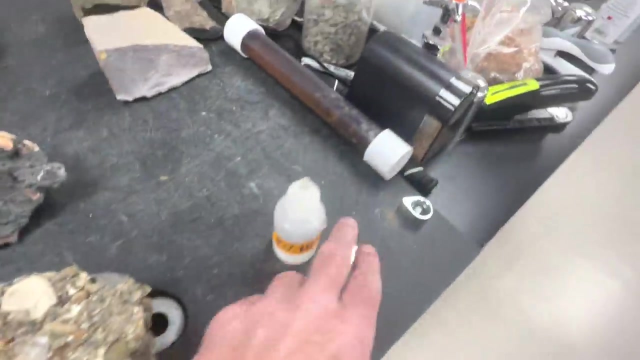 like how the rock feels to your hand, but, more importantly, it's going to be the shy size, shape, array and arrangement of the minerals, and so, for rocks that have larger particles, it might be pretty easy just to see- uh, with the naked eye, what's going on? um, i would recommend though, if you want, 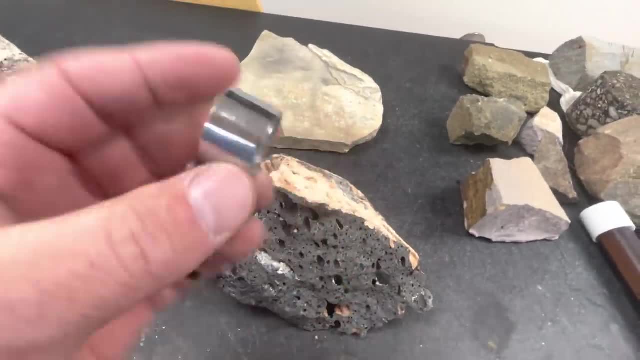 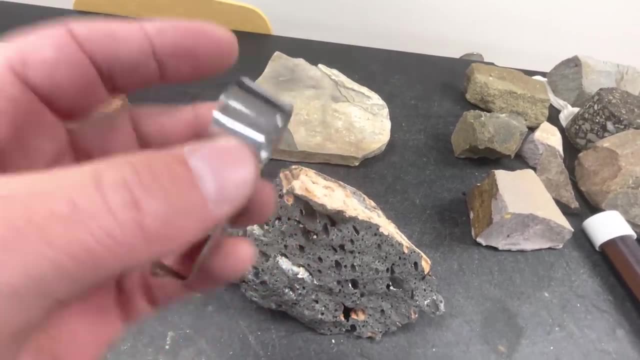 to get into this in some detail. you can get a hand lens, so just a simple loop or a little magnifying glass. a hand lens, uh, 10x, 15x or 20x would be good ones to get. 10x is kind of the one i prefer. um, that will allow you to see the particles a little bit. 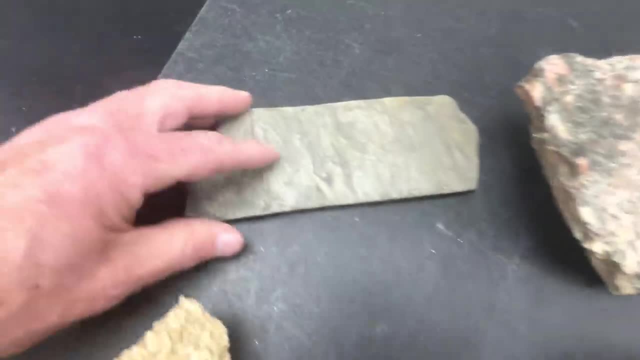 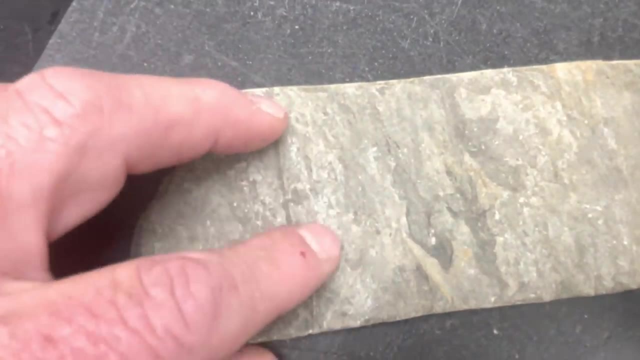 better because we get into these more. uh, fine grained rocks, maybe like this one here. uh, the particles are so small that it's a little hard to tell exactly what's going on, and so you might need some magnification to tell. but how big are the particles? are they all big? are they a mixture? 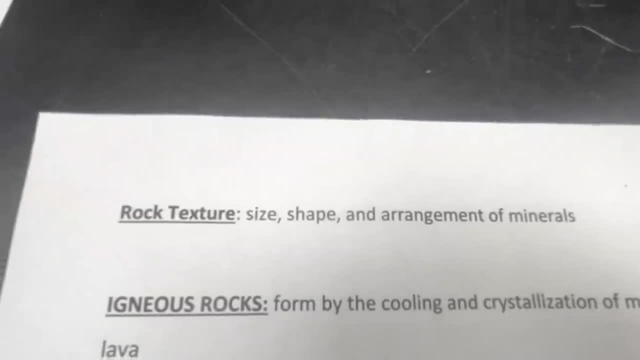 sorts of shortcuts there. so that's the rock cycle. so when we look at rocks, what do we? what are some of the main things we're looking for? well, we're looking at the texture of the rock. now that's sometimes that could be like how the rock feels to your hand. 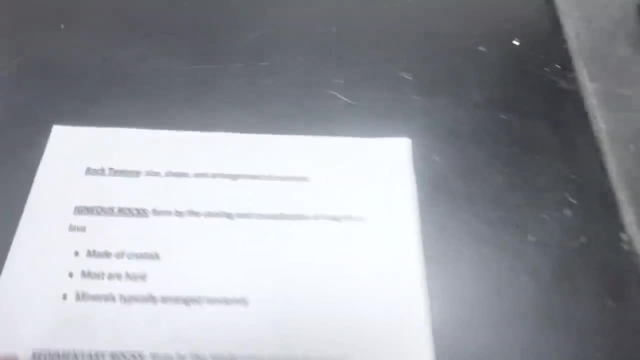 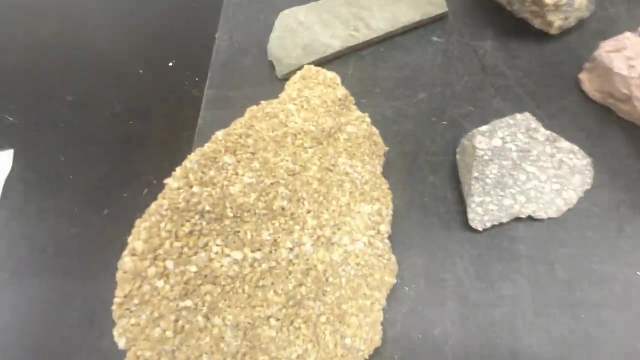 now, sometimes that could be like how the rock feels to your hand. sometimes that could be like how the rock feels to your hand hand. But more importantly, it's going to be the size, shape and arrangement of the minerals, And so, for rocks that have larger particles, it might be pretty easy just to see with the naked. 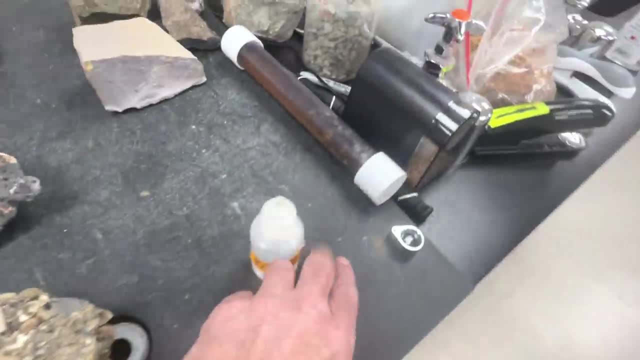 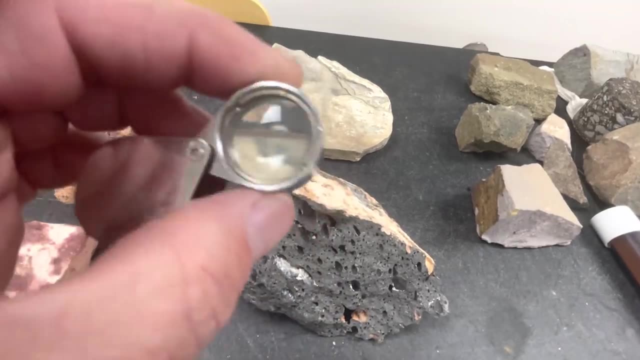 eye what's going on. I would recommend, though, if you want to get into this in some detail, you can get a hand lens, So just a simple loop or a little magnifying glass, a hand lens 10x, 15x or 20x. 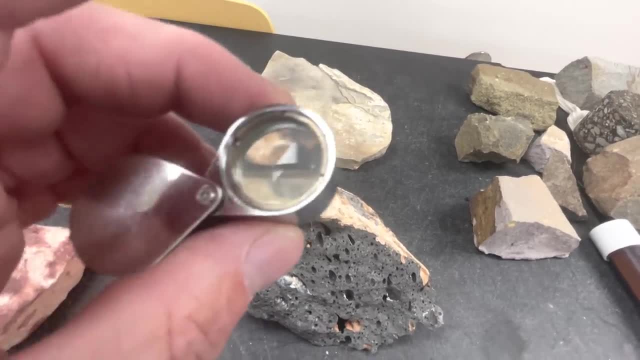 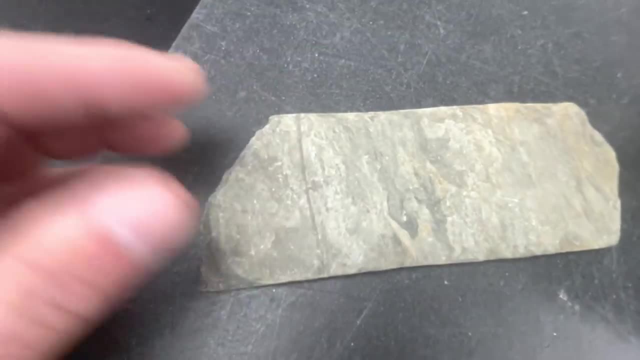 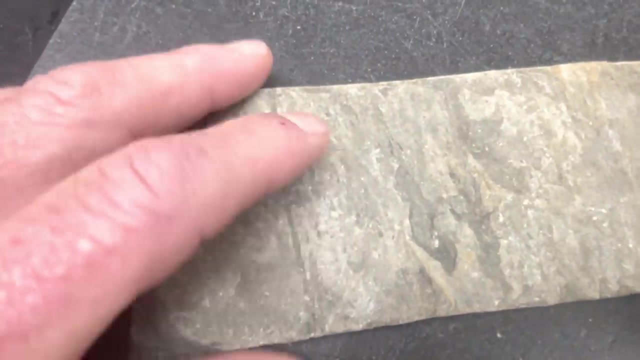 would be good ones to get. 10x is kind of the one I prefer. that will allow you to see the particles a little bit better, Because we get into these more fine-grained rocks, maybe like this one here. the particles are so small that it's a little hard to tell exactly what's going on, And so you might. 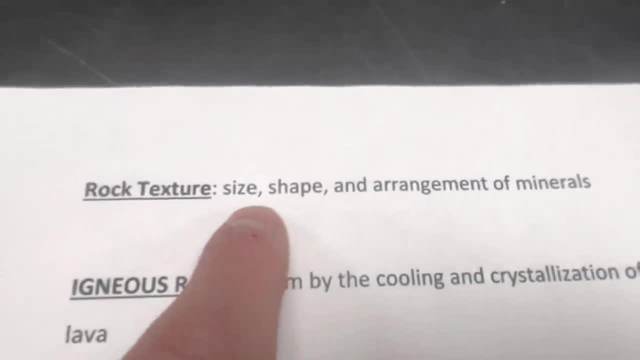 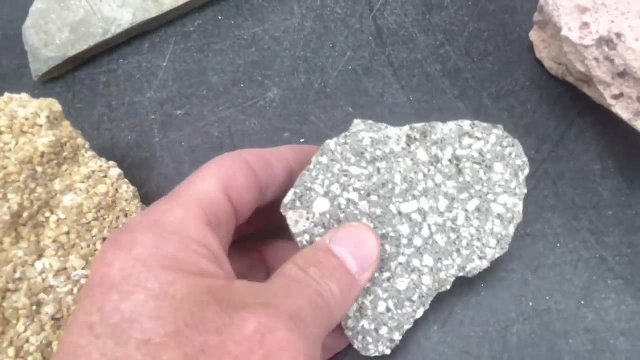 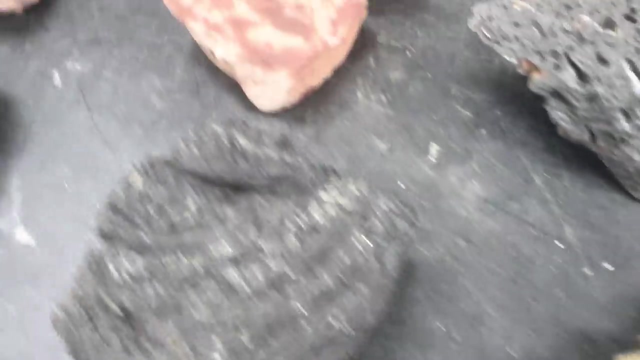 need some magnification to tell. But how big are the particles? Are they all big? Are they a mixture of big and small? We can see this rock here has a mixture of large and small particles, As does this rock over here. You can kind of see it with relation to my hand. Other rocks might. 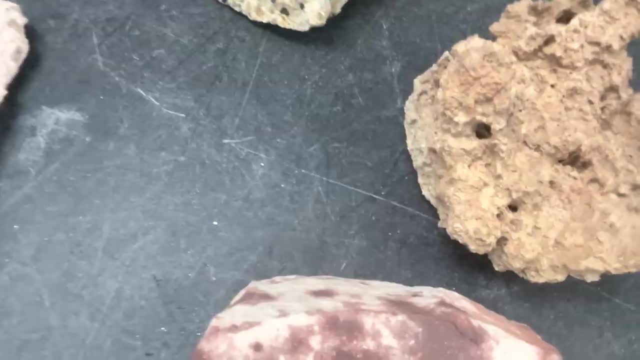 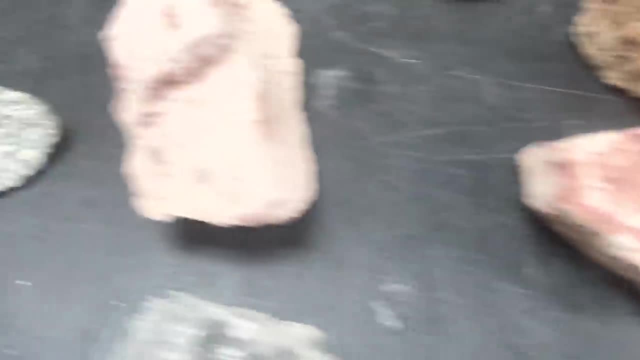 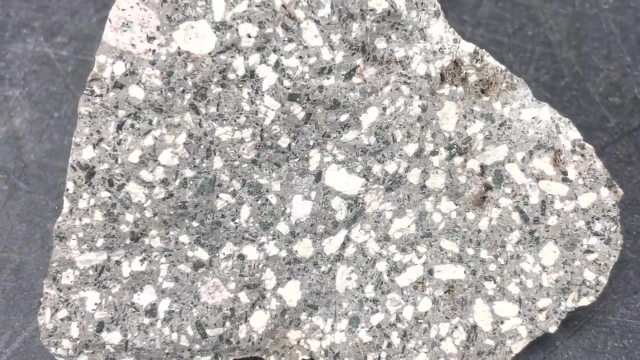 have generally all small particles. We want to look at the shape of those particles. Are they kind of rounded, maybe, in shape? If we look back at this one here, we can see a lot of these particles are somewhat angular in shape. So there's a different shape of the minerals that 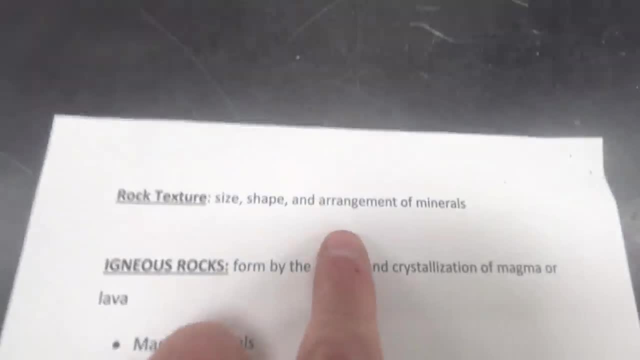 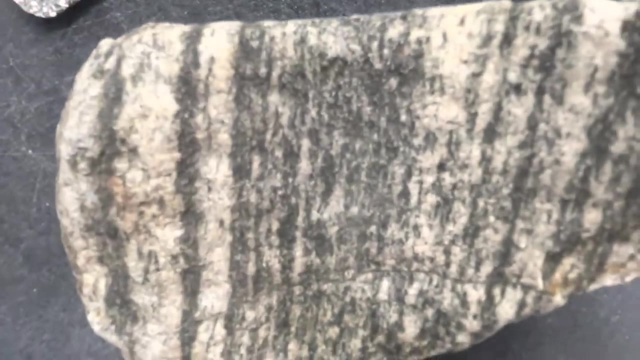 make up that rock there. And then we want to look also at how the minerals are arranged. So back to our metamorphic gneiss Here. they're arranged in nice lines So we can see there's definitely a fabric or an orientation. 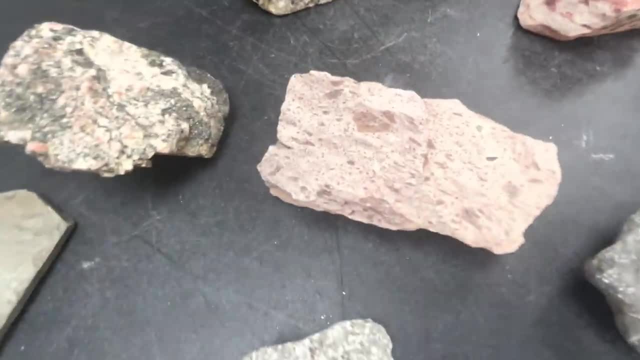 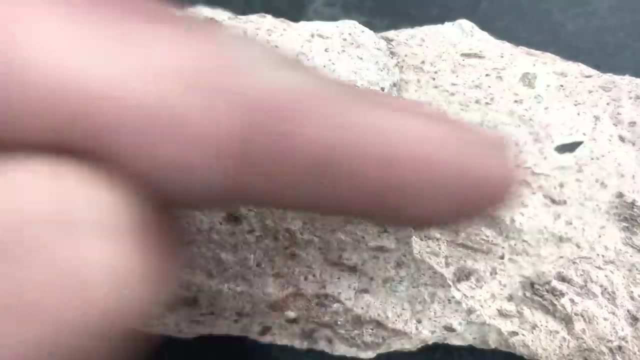 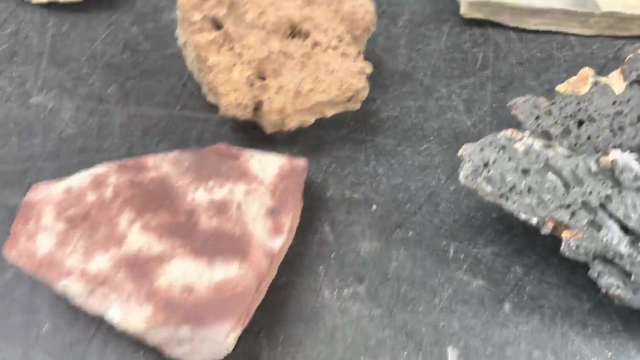 a preferred orientation of the minerals running through there. Even in this rock here we can crudely see that there's kind of a linear arrangement of the minerals this way, But it's not nearly as pronounced as some of these other ones we've looked at, And then sometimes it might. 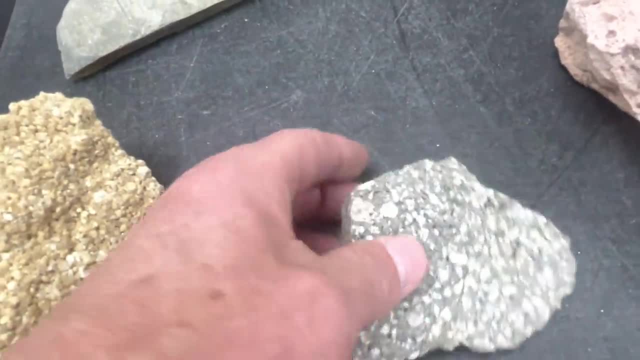 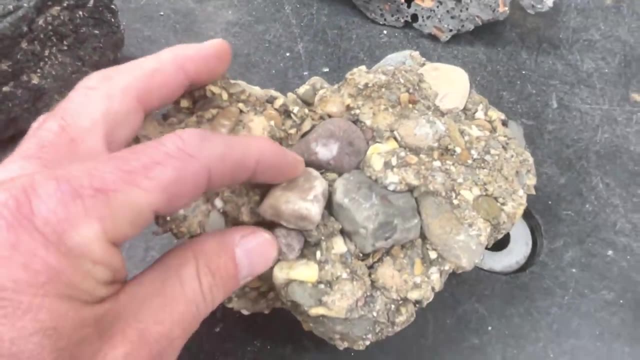 of big and small. we can see this rock here has a mixture of large and small particles, as does this rock here has a mixture of large and small particles, as does this rock here has a mixture of this rock over here. you can kind of see it with relation to my hand. other rocks might have. 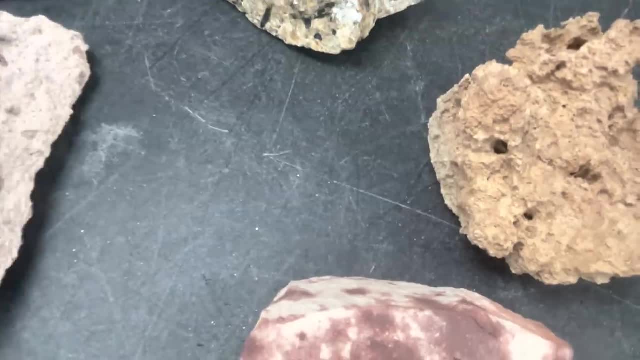 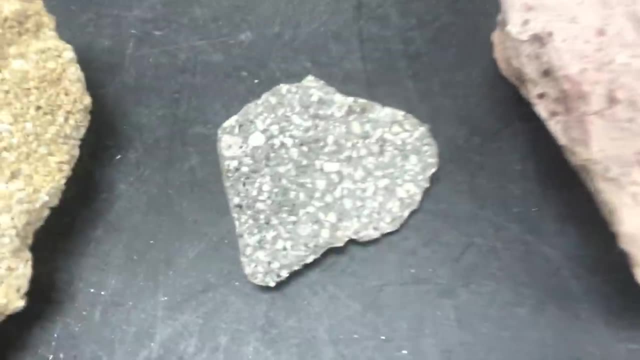 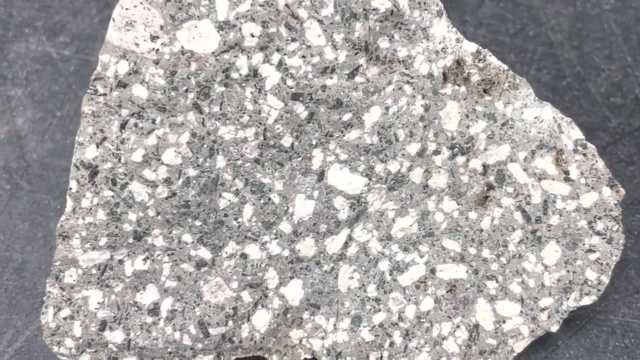 generally all small particles. we want to look at the shape of those particles. are they kind of rounded, maybe, in shape? if we look back at this one here, we can see a lot of these particles are somewhat angular in shape. so there's a different shape of the minerals that make up that rock there. 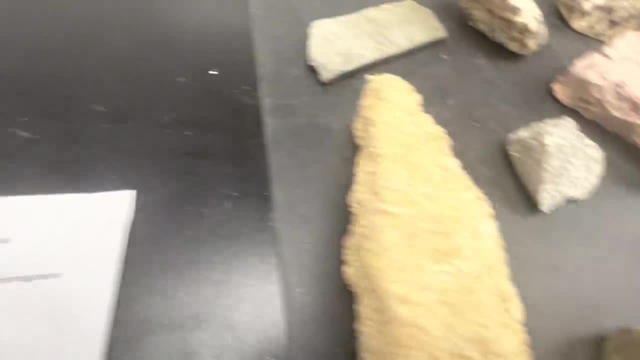 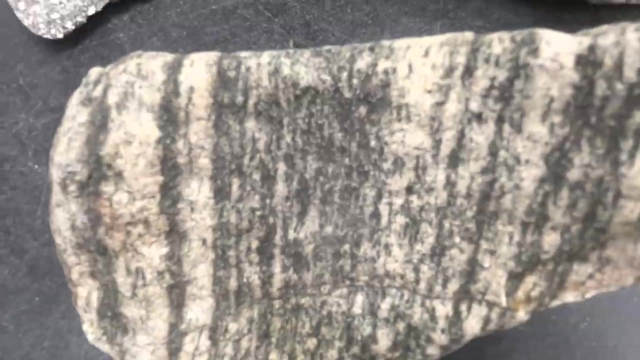 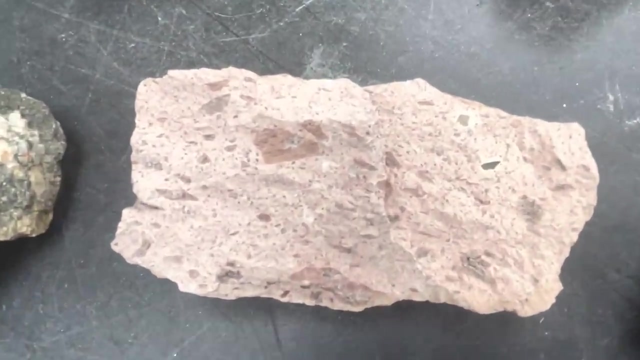 and then we want to look also at how the minerals are arranged. so back to our metamorphic nice. here they're arranged in nice uh lines, so we can see there's definitely a fabric or an orientation, a preferred orientation, the minerals running through there, uh, even in this rock here we can crudely see that there's kind of a linear 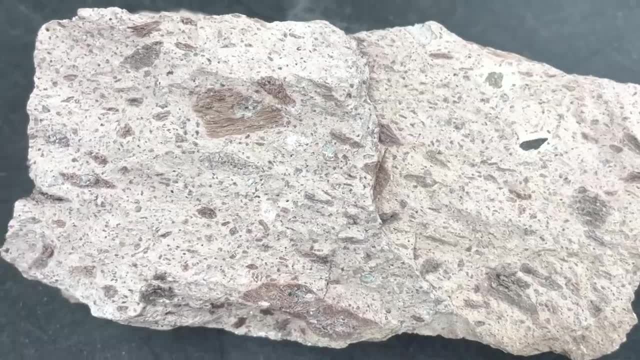 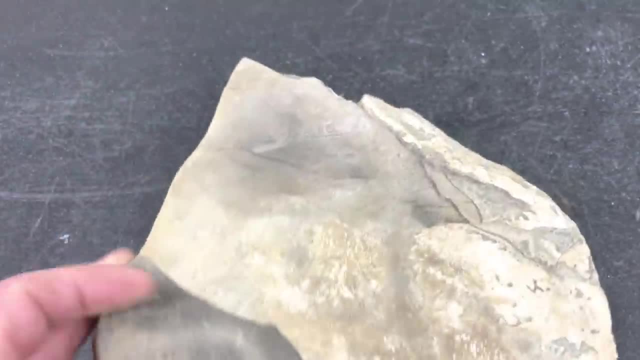 arrangement of the minerals this way, but it's not nearly as pronounced as some of these other ones we've looked at um, and then sometimes it might just be how the rock presents itself. this rock is presenting itself as kind of a flat sheet, and if i look on the end there i can actually see. 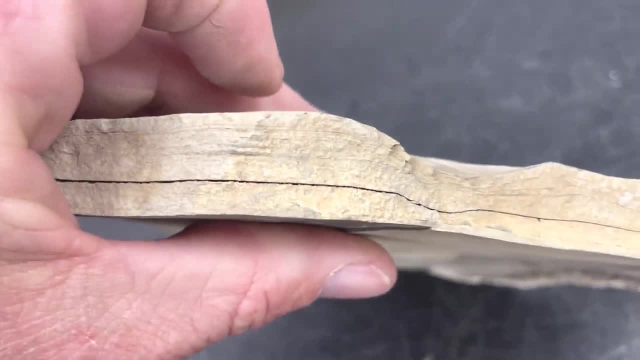 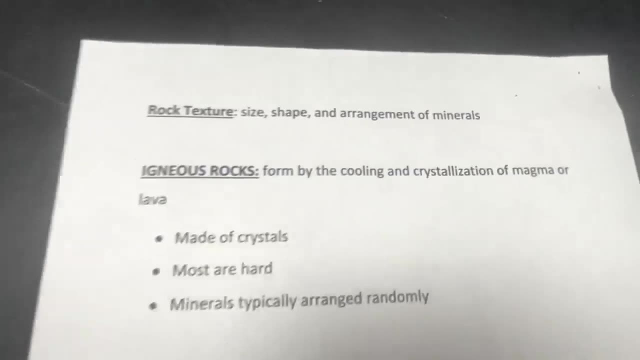 uh, some little thin lines running parallel to this planar fabric. so how are the minerals arranged? um so briefly, i don't want to- we'll spend more time on these later. but igneous rocks: these are the rocks formed by cooling and crystallization of magma or lava. 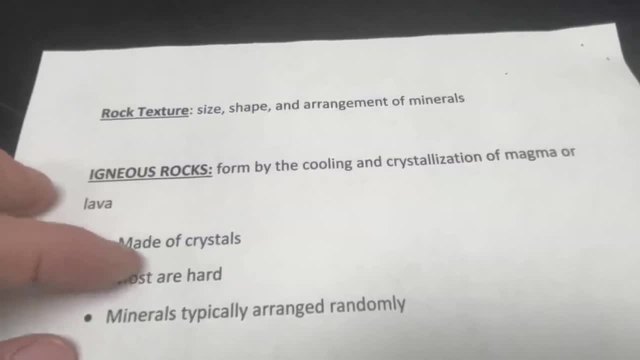 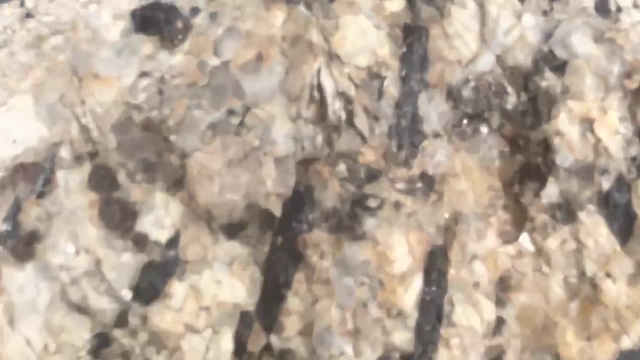 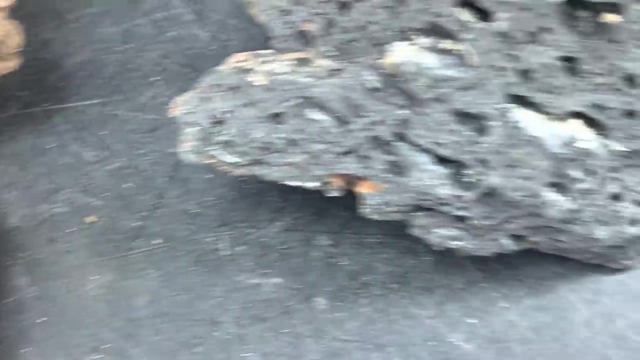 usually it's made out of crystals. they might be big crystals that you can see, as is the case over here with uh this rock. here you can actually see uh the individual minerals in here, or they might be quite small. so if i come over here to this igneous rock, actually you can see some of the minerals in. 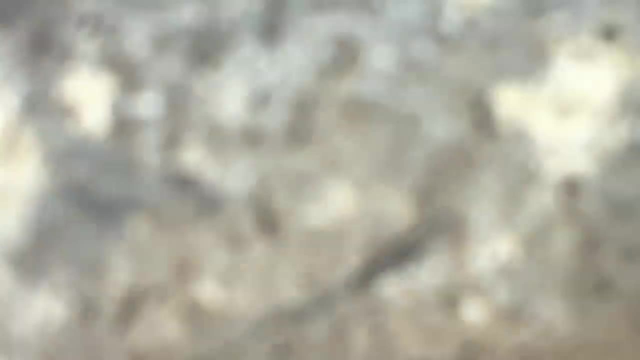 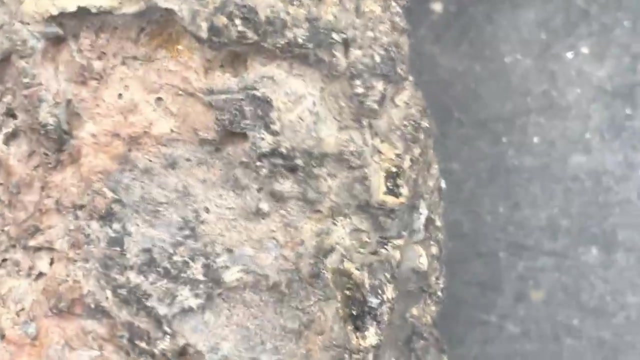 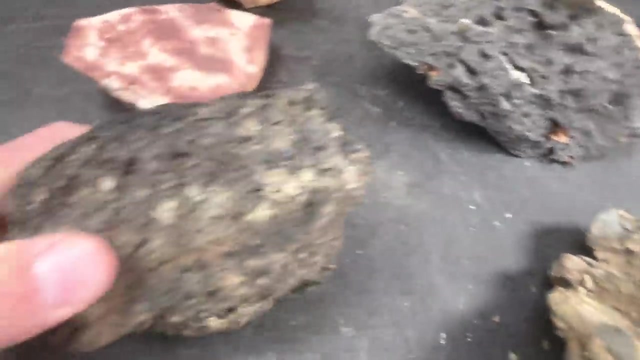 here, um, but other samples. here's maybe a better one. let's get that in focus. there we go um. the minerals aren't as obvious. remember, too, that one of the most important things you can do, uh, when you're looking at a rock, it's really hot and you're looking for something that's right up to the 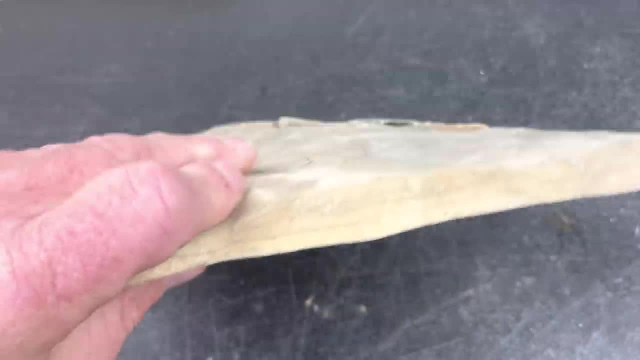 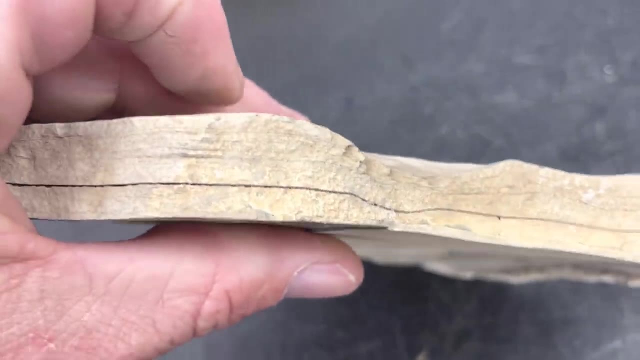 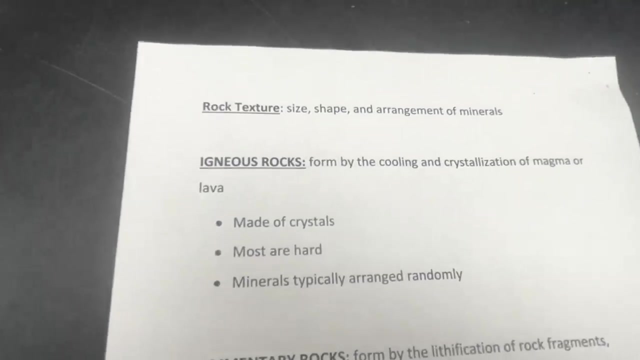 be that the rock presents itself. This rock is presenting itself as kind of a flat sheet, And if I look on the end there, I can actually see some little thin lines running parallel to this plane or fabric. So how are the minerals arranged? So briefly, I don't want to. we'll spend more time on. 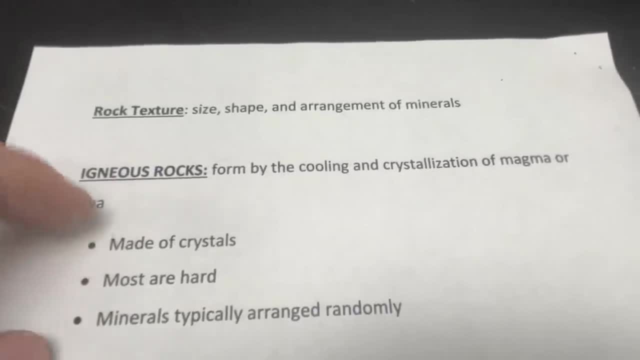 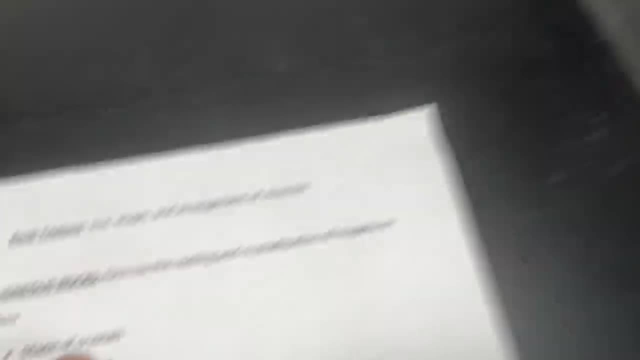 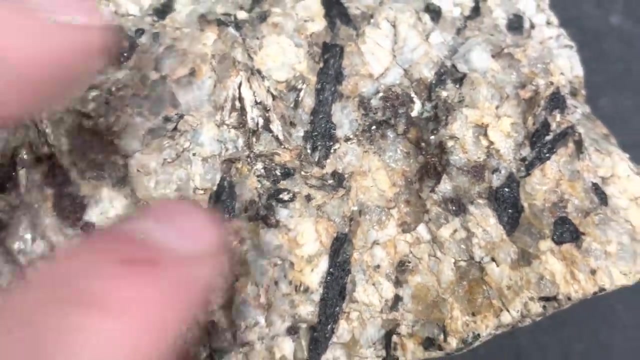 these later, But igneous rocks. these are the rocks formed by cooling and crystallization of magma or lava. Usually it's made out of crystals. They might be big crystals that you can see, as is the case over here with this rock. here You can actually see the individual minerals in here. Or 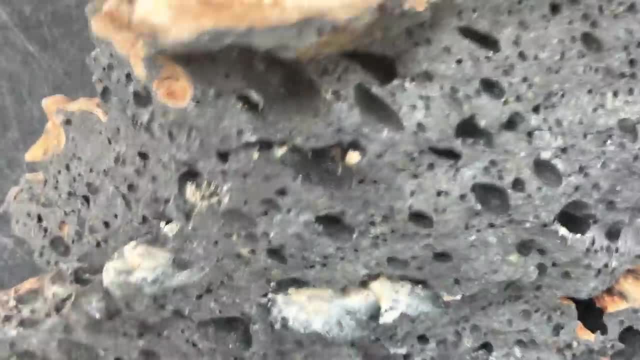 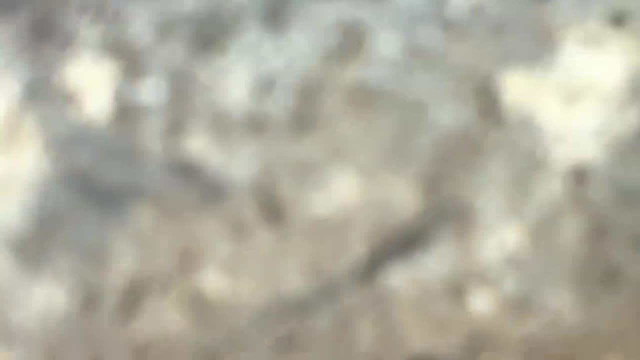 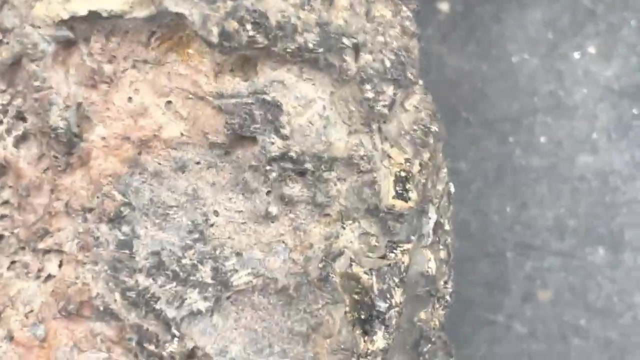 they might be quite small. So if I come over here to this igneous rock- actually you can see some of the minerals in here, But other samples here's maybe a better one. Let's get that in focus. There we go. The minerals aren't as obvious. Remember, too, that one of the most important things you 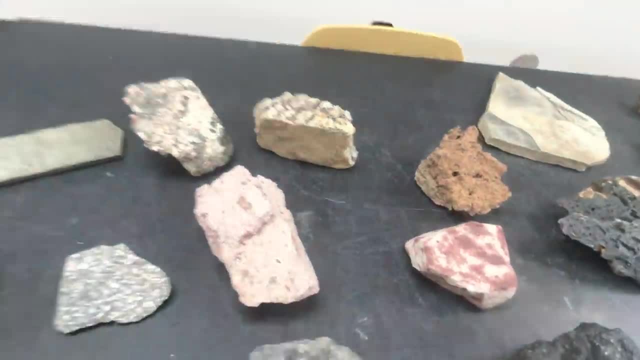 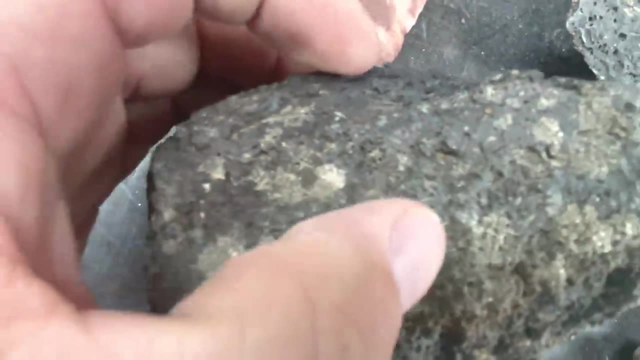 can do when you're trying to identify a rock is: break a freshener. You can break a freshener, but you can also break a fresh surface. So this surface here is pretty weathered. It's got maybe lichen growth on it or it's discolored. So we want to make sure we're looking at a fresh surface. I 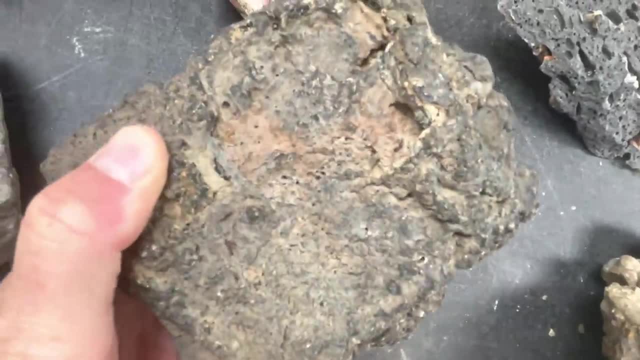 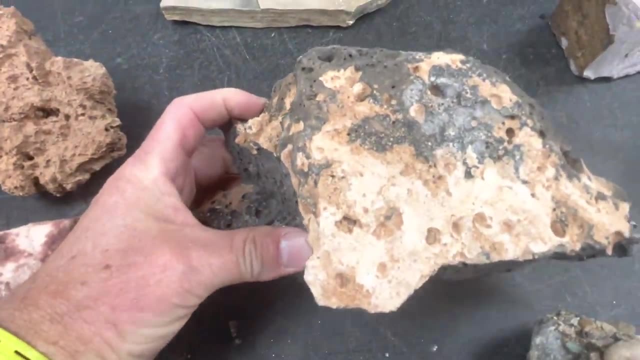 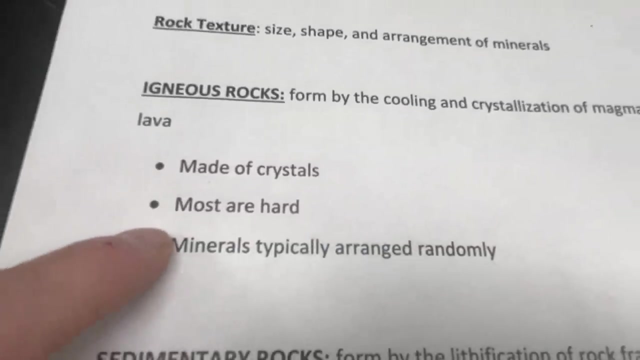 picked this one up and apparently didn't whack it with a hammer, So it does not have much of a fresh surface on it, As opposed to this one where you can see it's a nice clean face there. When you look at the top side, there it's much more kind of weathered. So, yeah, a lot of the igneous rocks are. 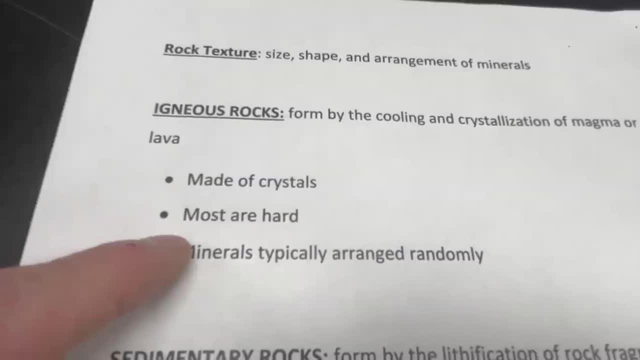 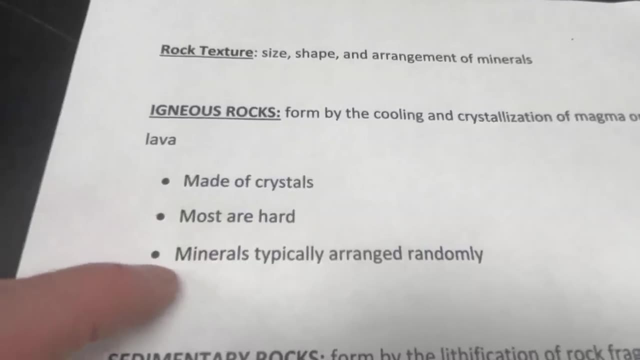 not always, but generally they're harder. So if you're looking in a stream or a beach where the rocks have been kind of tumbled a little bit, it's a good place for igneous rocks or certain types of igneous rocks to form, And most igneous rocks. they have sort of a random arrangement of the minerals. 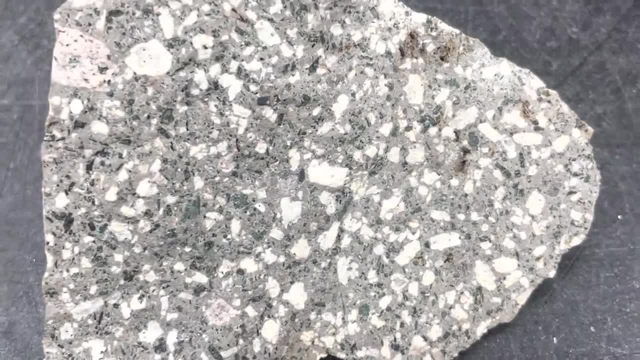 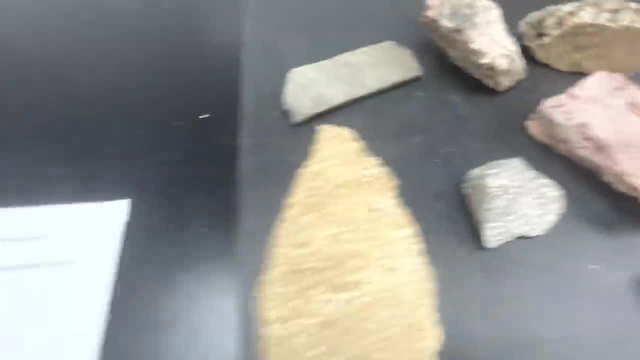 So again kind of back to this rock here. If you look at the crystals in there, they're pretty randomly arranged. There doesn't seem to be a preferential orientation to any of those particles there. Moving on to the sedimentary rocks, 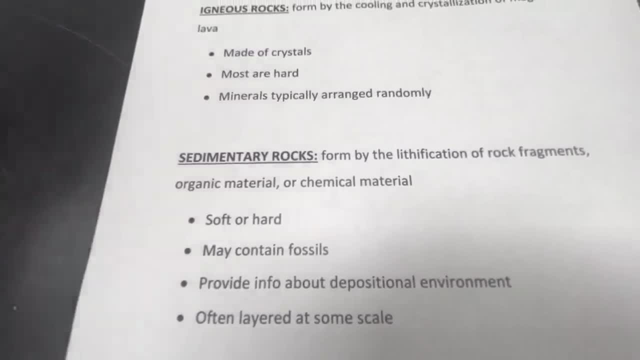 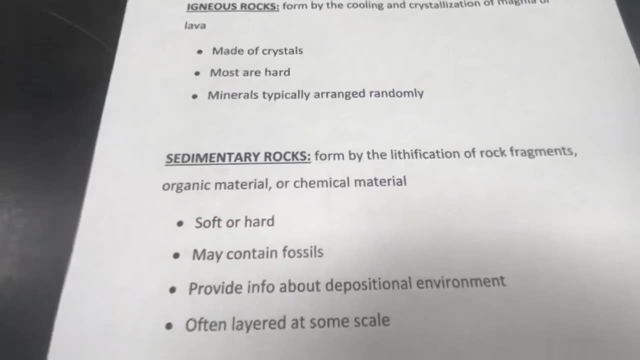 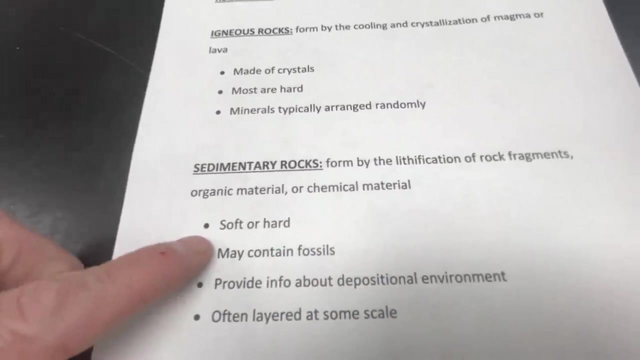 These are rocks that form when we have weathered rock fragments, grains, or what we sometimes call clasts. Could be organic material, so like shells, or plant material or other types of fossils, or sometimes even chemical material that precipitates. These can be soft or hard. There's some. 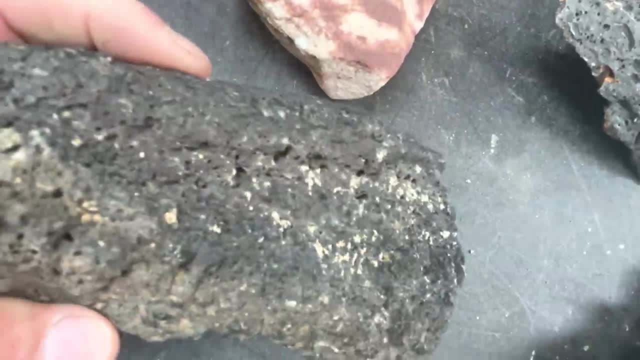 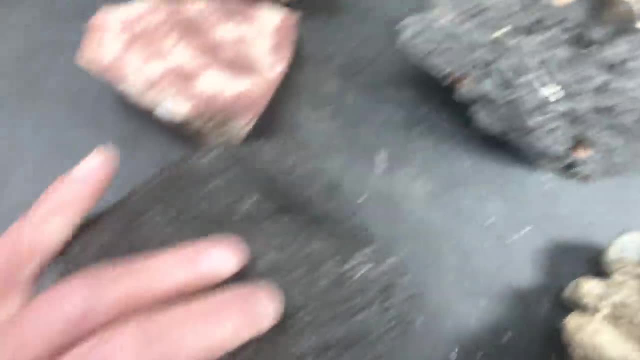 surface. it's pretty hard to find it. so this surface here is pretty weathered. it's got maybe lichen growth on it or it's discolored, uh, so we want to make sure we're looking at a fresh surface. i picked this one up and apparently didn't whack it with a hammer, so it does not have much of a. 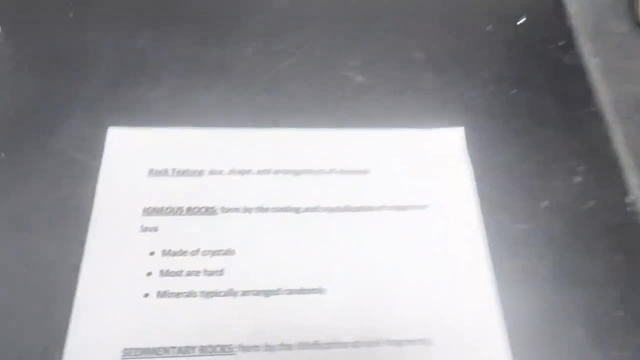 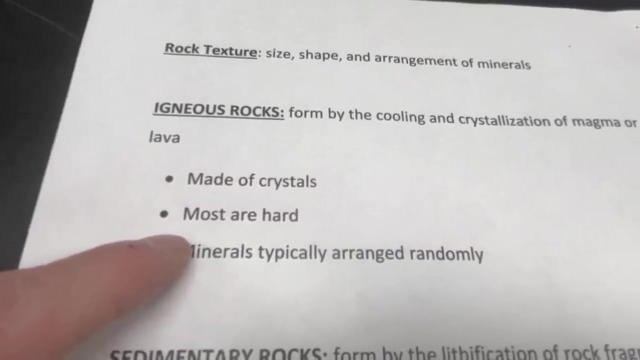 fresh surface on it, as opposed to this one, uh, where you can see it's a nice clean face there. when you look at the top side, there it's much more kind of weathered, um harder so if you're looking in a stream or a beach where the rocks have been kind of tumbled a little. 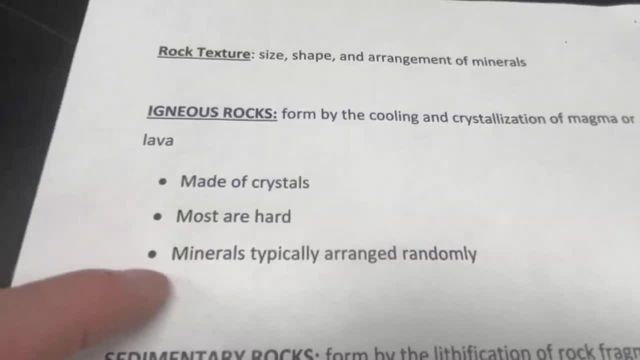 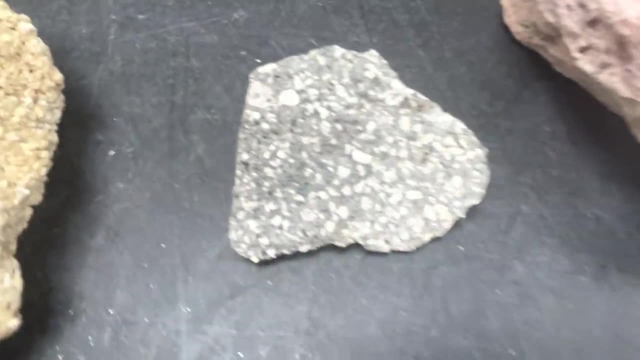 bit. it's a good place for igneous rocks or certain types of igneous rocks to form and most igneous rocks they have sort of a random arrangement of the minerals. so again kind of back to to this rock here. if you look at the, the crystals in there, they're pretty randomly arranged there, doesn't? 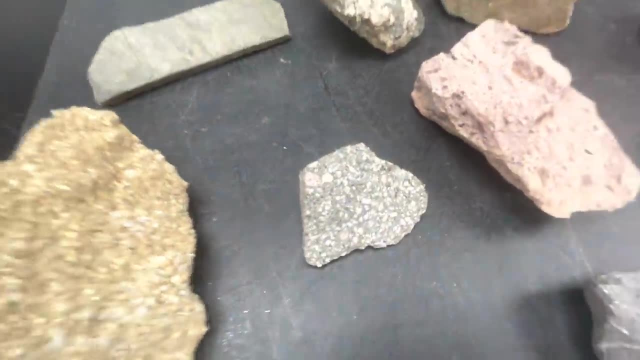 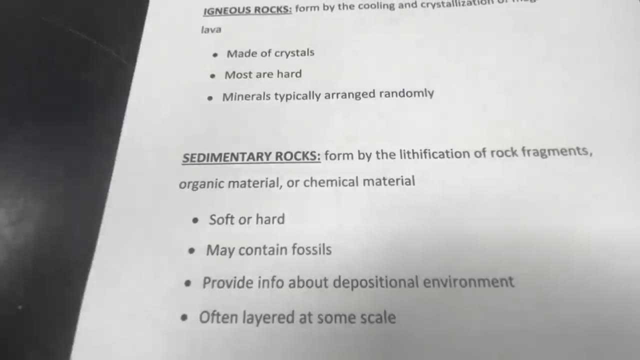 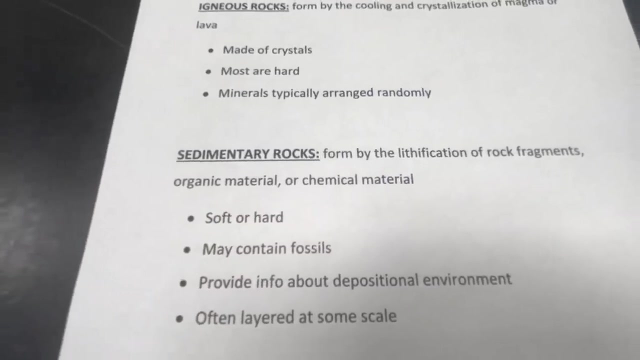 seem to be a preferential orientation to any of those particles there. moving on to the sedimentary rocks, these are rocks that form when we have weathered rock fragments, grains, what we sometimes call clasts- could be organic materials, so like shells or plant material or other types of fossils. 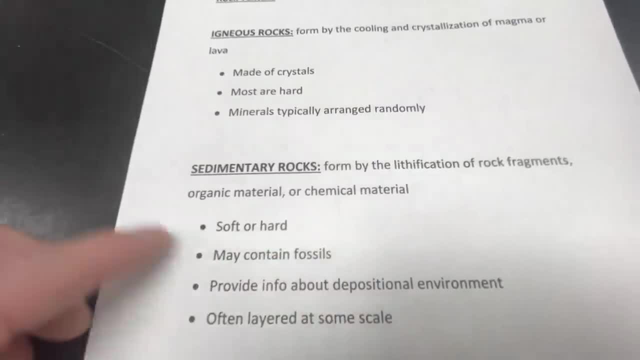 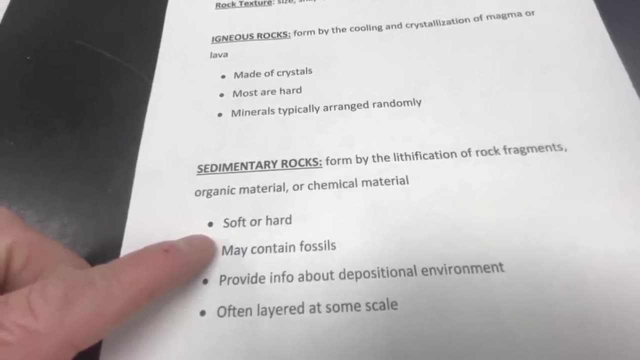 or sometimes even chemical material that it precipitates. these can be soft or hard. there's some sedimentary rocks that are quite hard, others that are quite soft. you can just kind of disaggregate them with your hand. almost these are the rocks that contain the fossils generally. so. 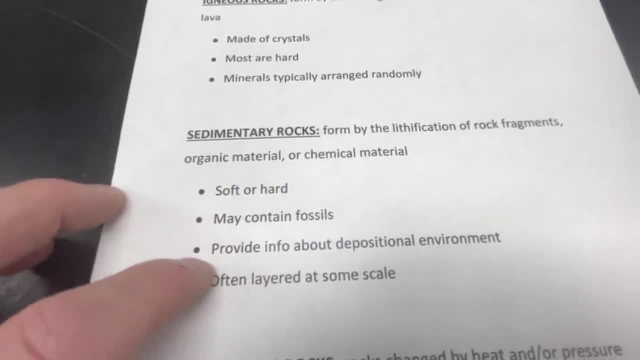 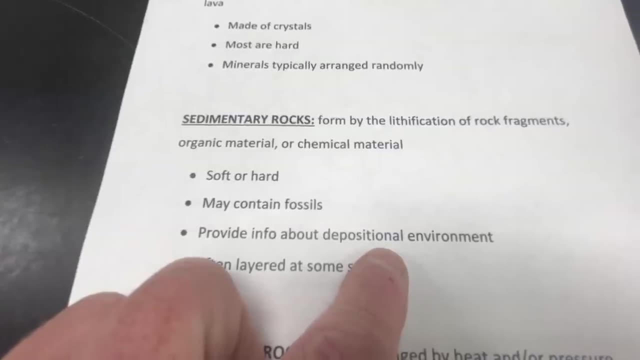 not all sedimentary rocks contain fossils, but many do. These give us information about what the environment was at the time it was deposited. It's what we call the depositional environment. So an example of that would be: if we have a sandstone, what are good places for sand to be deposited? Well, we 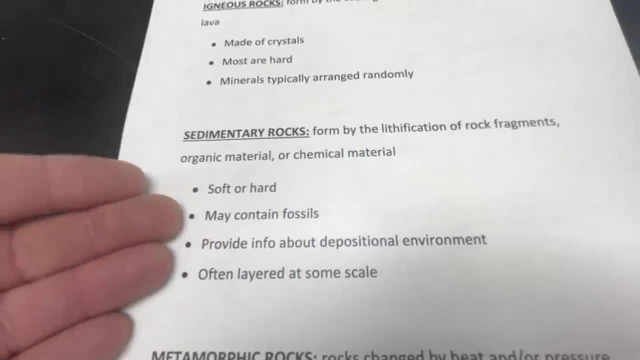 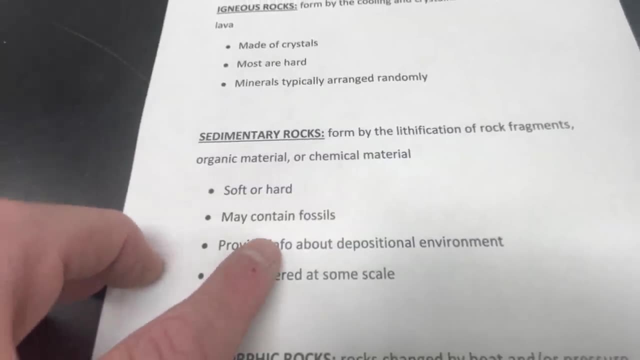 think of beaches, We think of, maybe, river systems like the shoreline of a river, We think of sand dunes. Those are all in depositional environments. So sediment rocks tell us what was going on at the surface, What was the climate like or the general environment. And a lot of sediment rocks. 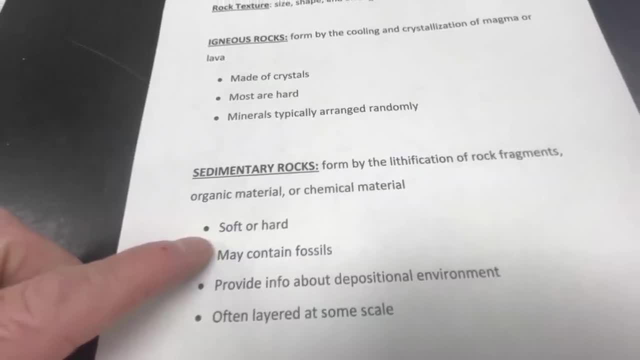 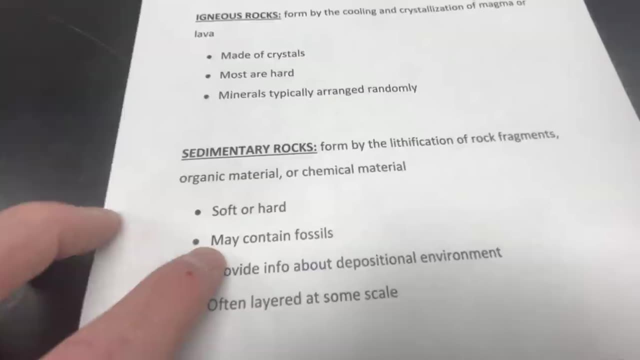 sedimentary rocks that are quite hard, others that are quite soft. You can just kind of disaggregate them with your hand. almost These are the rocks that contain the fossils generally, So not all sedimentary rocks. Some sedimentary rocks contain fossils, but many do. These give us information about what the 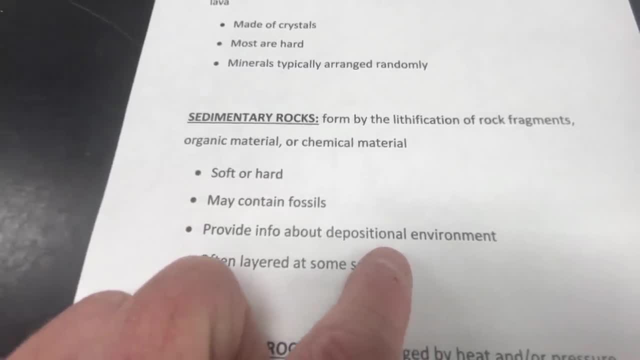 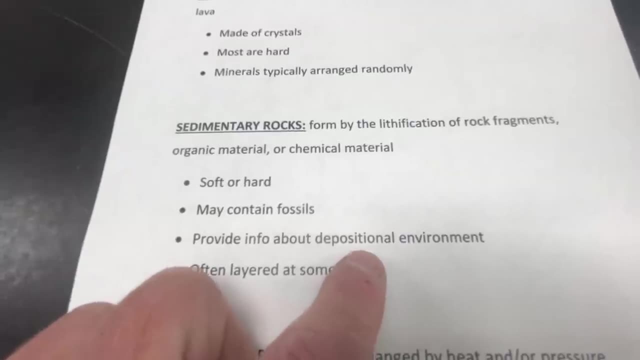 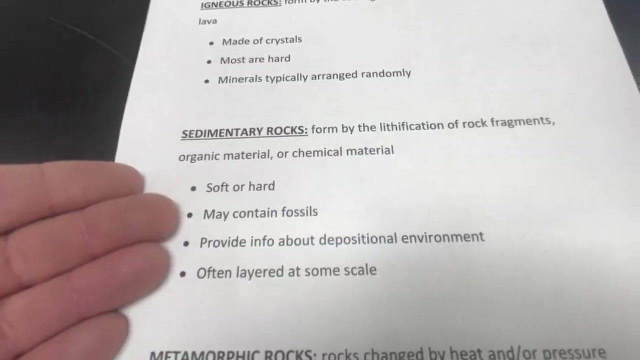 environment was at the time it was deposited. It's what we call the depositional environment. So an example of that would be: if we have a sandstone, what are good places for sand to be deposited? Well, we think of beaches. We think of, maybe, river systems, like the shoreline of a river. We think of 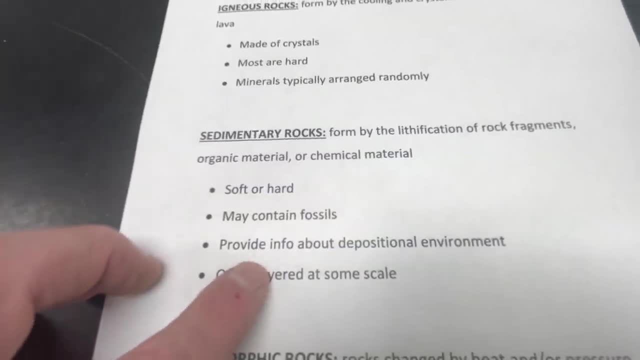 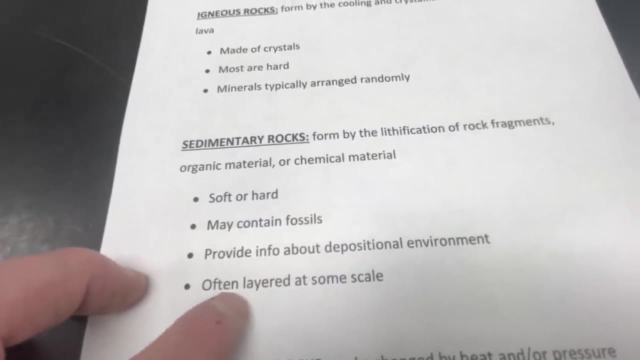 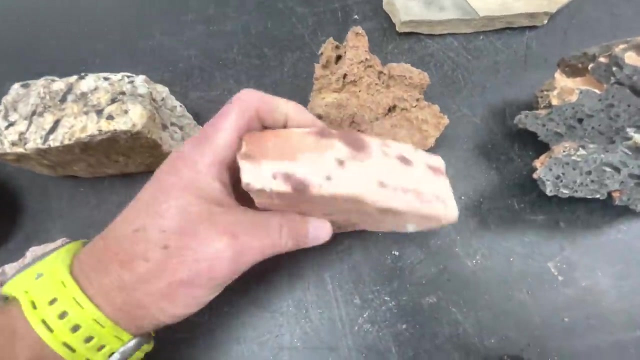 sand dunes. Those are all in depositional environments. So sedimentary rocks tell us what was going on at the surface. They tell us the climate-like or the general environment, And a lot of sedimentary rocks will have layering. Maybe they'll be layered, you know, at this level here. Let me see if I can get a good view of this one. 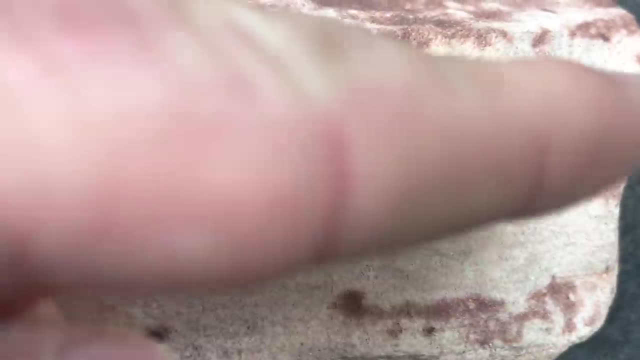 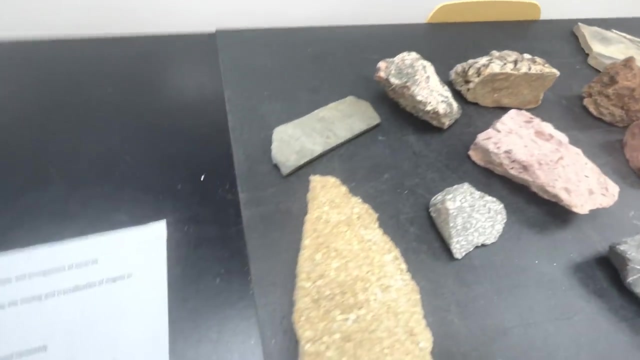 So if you kind of look at this one here, you can see there's some layers running this way, Maybe not at this scale, but maybe the whole outcrop scale. So maybe you look at a whole cliff face and you see some layering there. 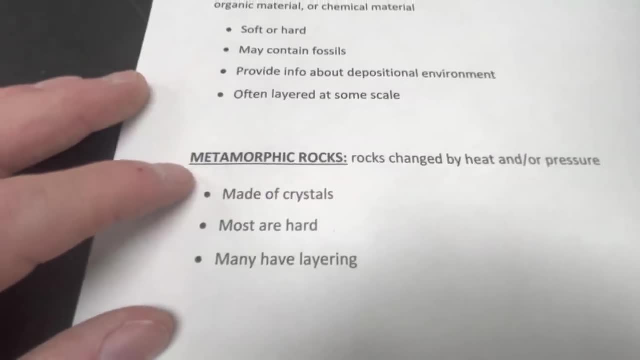 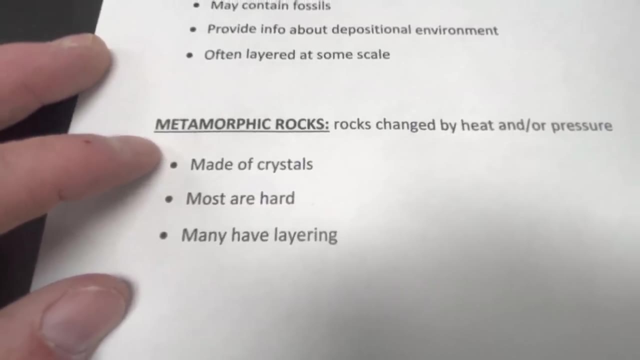 Moving on to the metamorphic rock. So these rocks get changed by heat or pressure or both. So when we have rocks that are kind of cooked or baked, put in the pressure cooker, if you will. it changes them into metamorphic rocks. 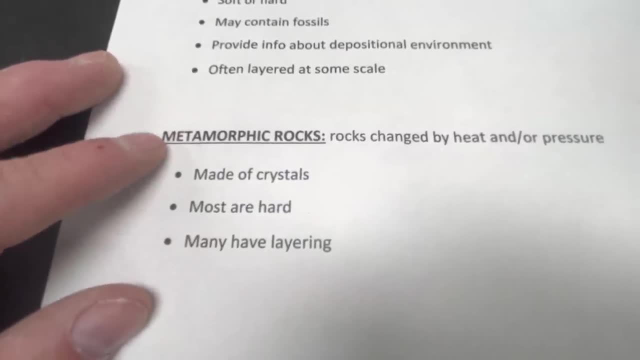 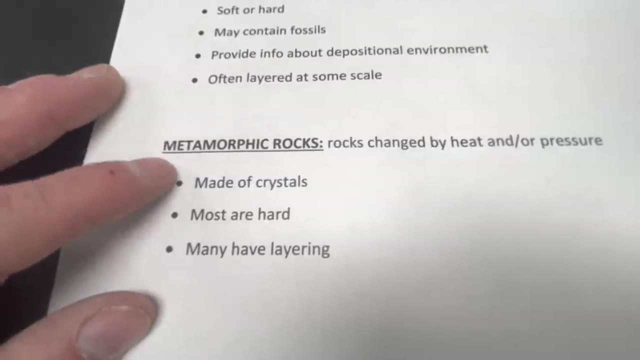 One big misnomer about metamorphic rocks is it does not involve melting. Remember, if you melt a rock, you are back to the igneous world. So metamorphism is a solid state change. We're changing one rock into another purely by adding heat, pressure and time. 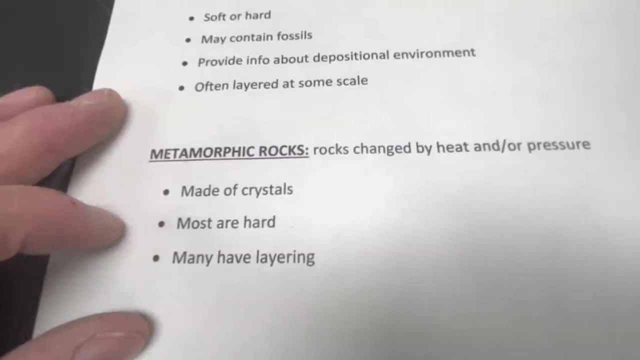 So metamorphic rocks, much like the igneous rocks, are going to be made out of metal. They're going to be made out of crystals. A lot of them are hard And some of them have layering, like we see here with this one or this one here. 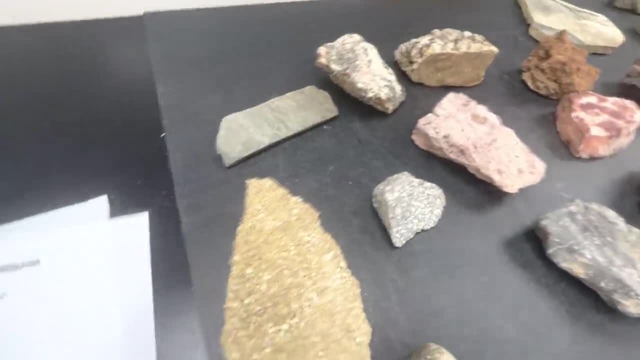 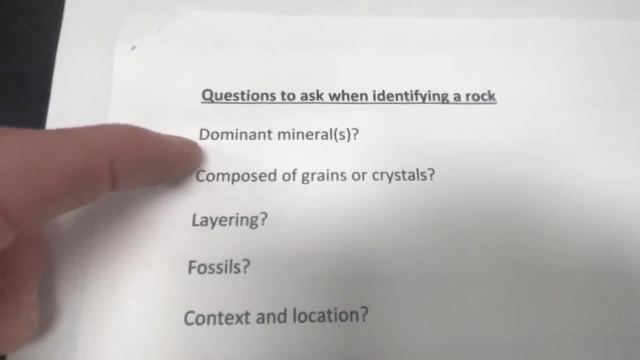 So let's look at these real quickly And just a couple of questions we can think of when we're looking at a rock. So what is it made out of? We had a whole mineral series. I tried to cover most of the major minerals. 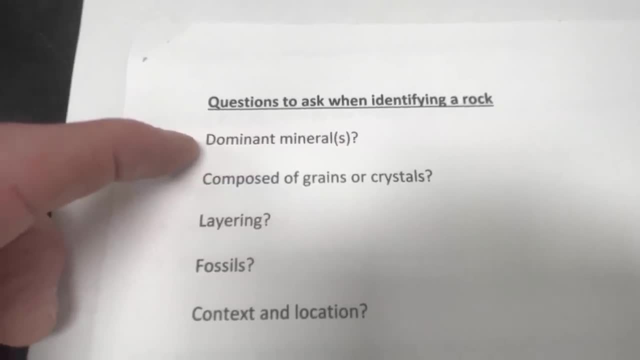 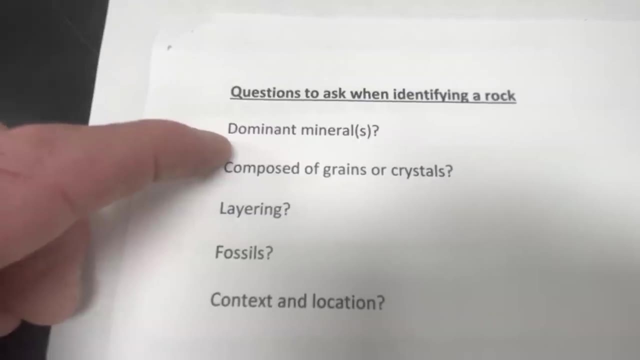 And as I look at these rocks next to me here, yeah, I think most of the minerals in most of these rocks are ones that we've covered in our mineral series, So these should be minerals that you can use, You can identify to some degree. 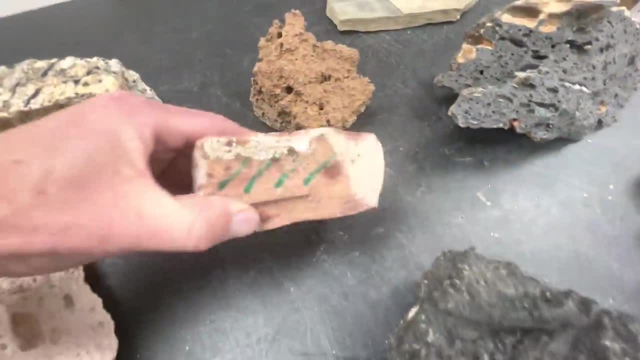 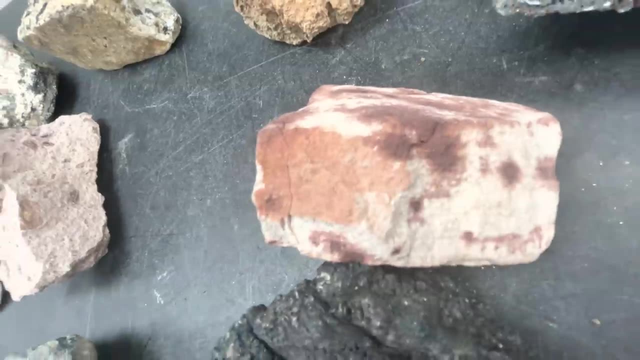 will have layering. Maybe they'll be layered. you know, at this level here Let me see if I can get a good view of this one. So if you kind of look at this one here, you can see there's some layers. 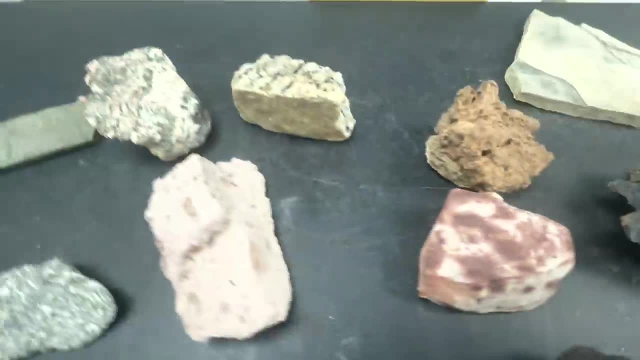 running this way, Maybe not at this scale, but maybe the whole outcrop scale. So maybe you look at a whole cliff face and you see some layering there Moving on to the metamorphic rock. So these are the layers that we're looking at. So these are the layers that we're looking at. So 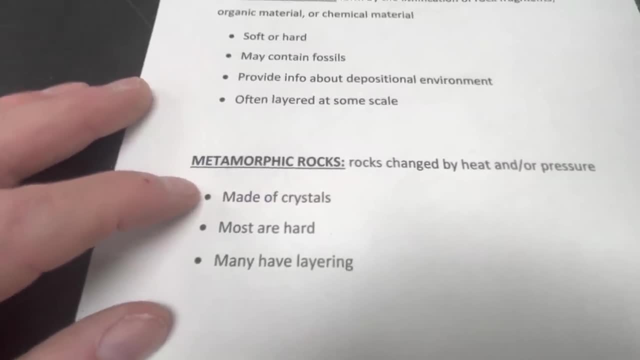 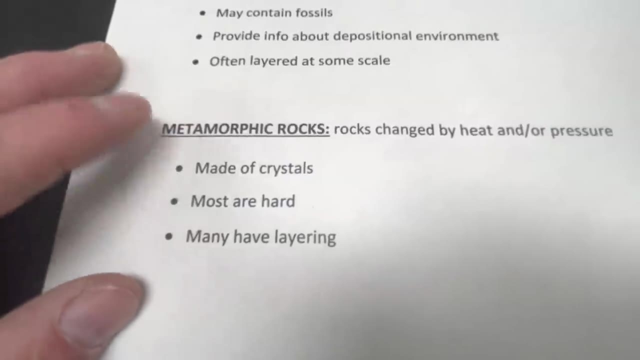 these rocks get changed by heat or pressure or both. So when we have rocks that are kind of cooked or baked, put in the pressure cooker, if you will. it changes them into metamorphic rocks. One big misnomer about metamorphic rocks is it does not involve melting, Remember, 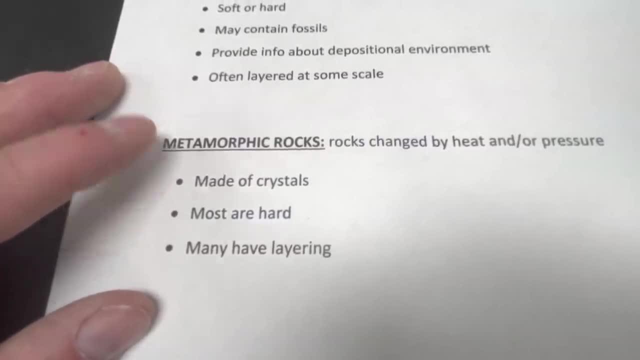 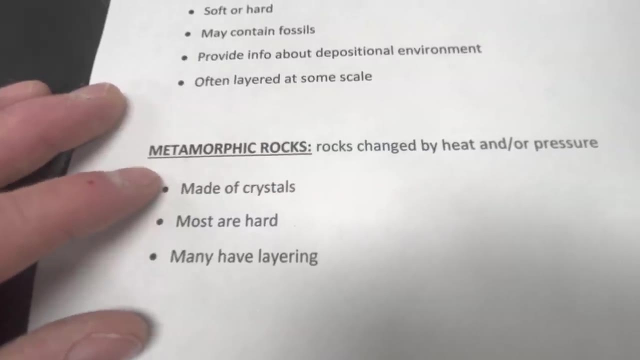 if you melt a rock, you are back to the igneous world. So metamorphism is a solid state change. We're changing one rock into another purely by adding heat, pressure and time. So metamorphic rocks, much like the igneous rocks, are going to be made out of metal. So we're going to be. 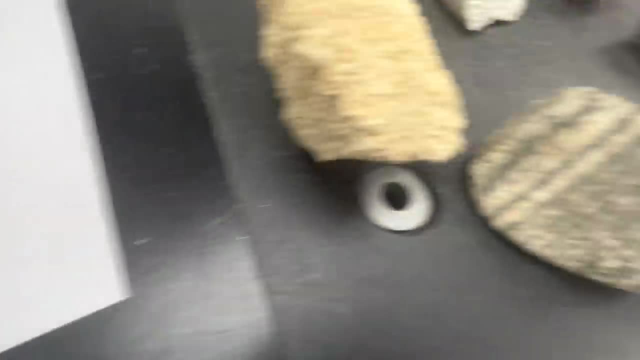 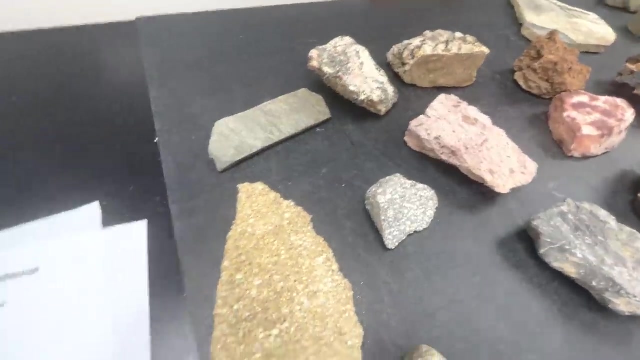 making them out of crystals. A lot of them are hard and some of them have layering, like we see here with this one or this one here. So let's look at these real quickly And just a couple questions we can think of when we're looking at a rock. So what is it made out of? We had a whole 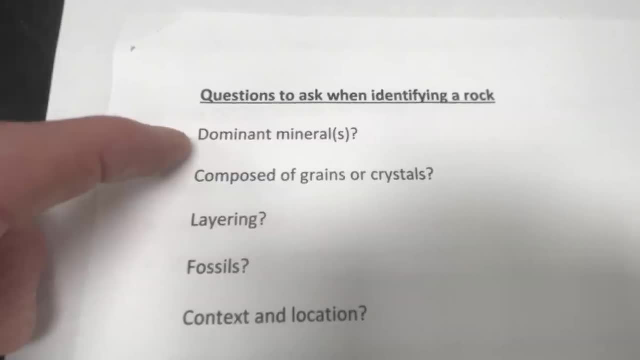 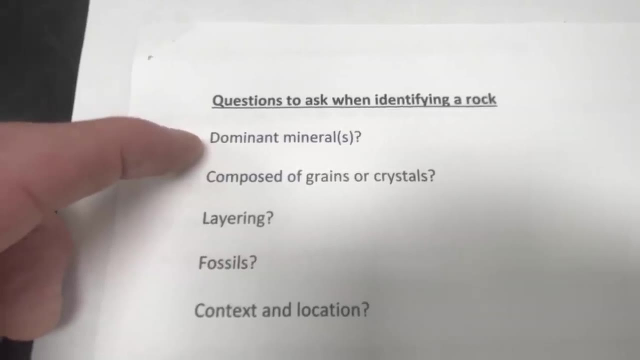 mineral series. I tried to cover most of the major minerals And, as I look at these rocks next to me here, yeah, I think most of the minerals in most of these rocks are ones that we've covered in our mineral series, So these should be minerals that you can. 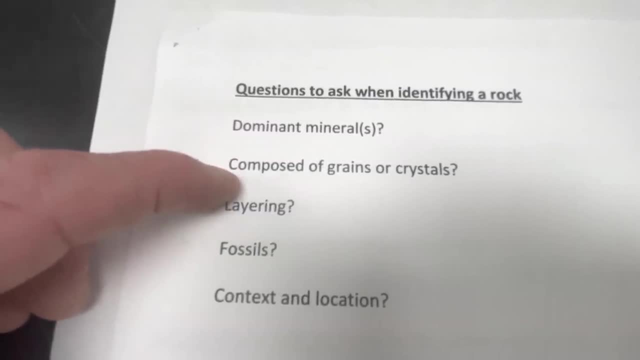 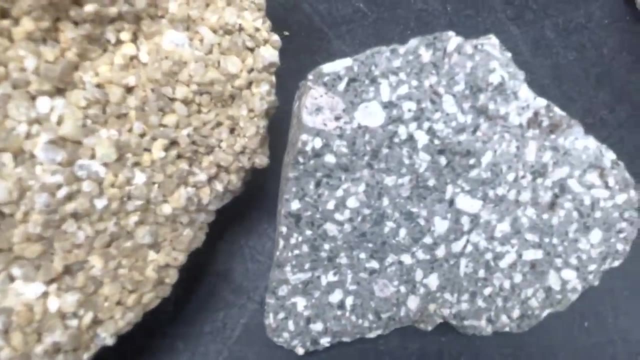 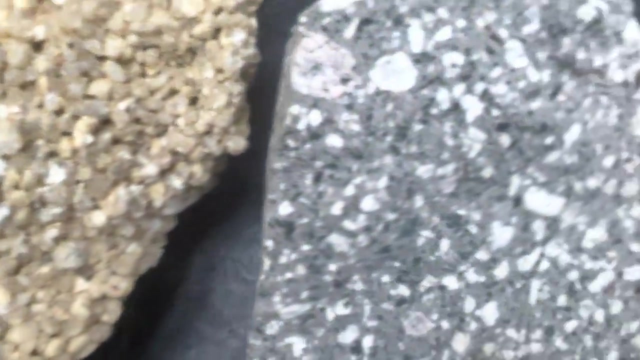 identify to some degree What's the rock made out of. Is it grains or is it crystals? So, for example, these two rocks have roughly similar sized particles in them, maybe about a centimeter or less, But we can see that when we look at this rock, that the particles are crystals. If I kind 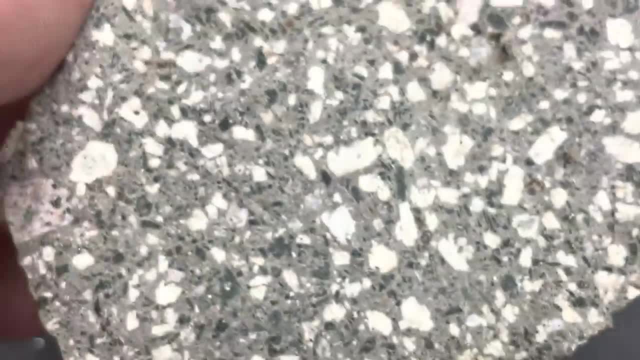 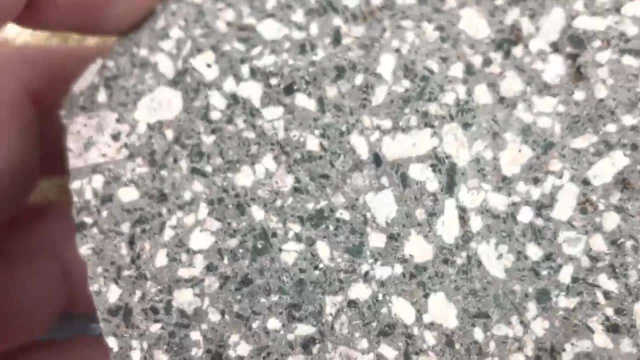 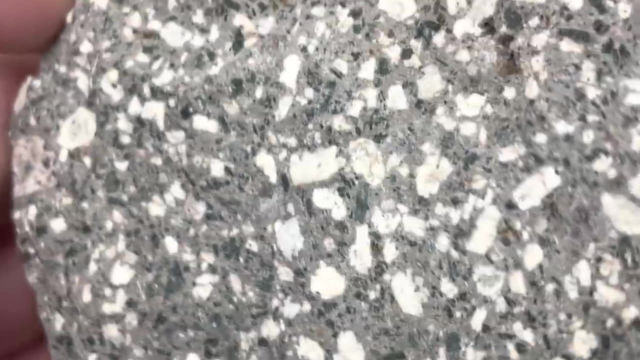 of rotate some of these in the light, sorry, trying to get all in focus here. I can see some particular And remember that the property of a mineral that will reflect light is cleavage planes, And so are you looking at crystals of minerals as we are here, Or are you looking at 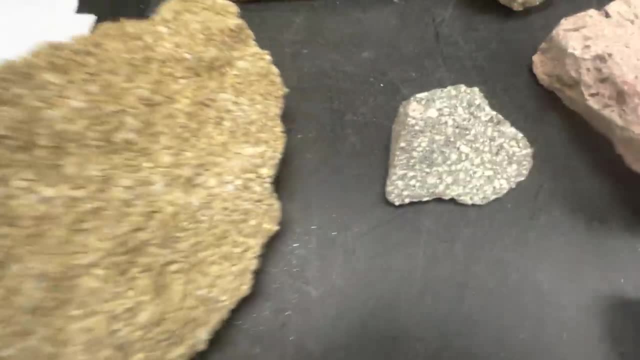 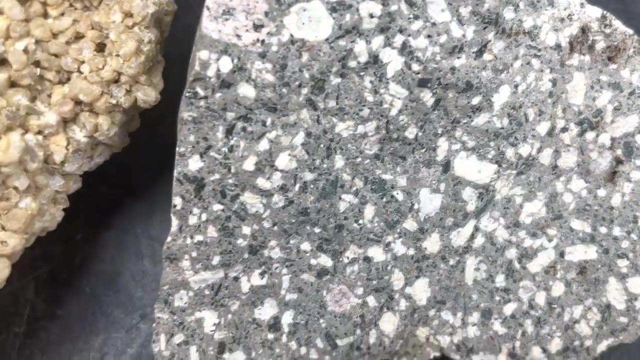 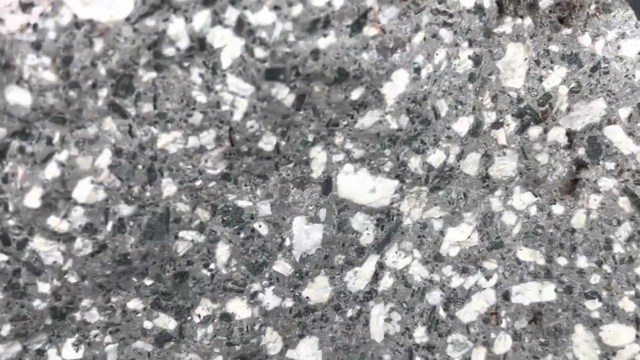 What's the rock made out of? Is it grains or is it crystals? So, for example, these two rocks have roughly similar sized particles in them, maybe about a centimeter or less, But we can see that, when we look at this rock, that the particles are crystals. 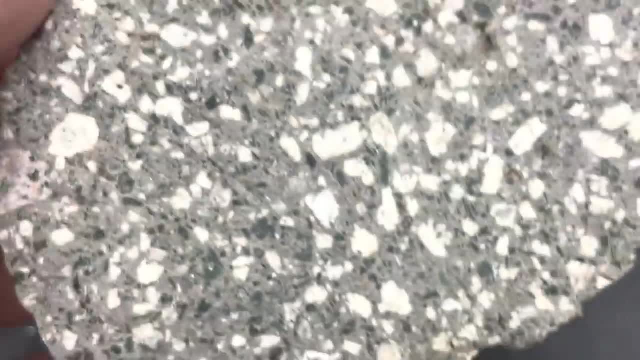 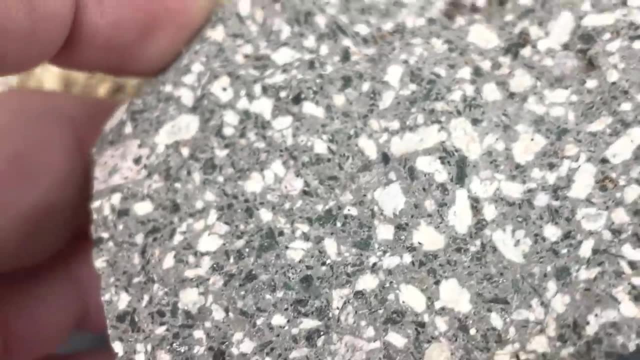 If I kind of rotate some of these in the light- sorry, trying to get all in focus here- I can see some reflections- And there's one right there. And remember that the property of a mineral that will reflect light is cleavage planes. 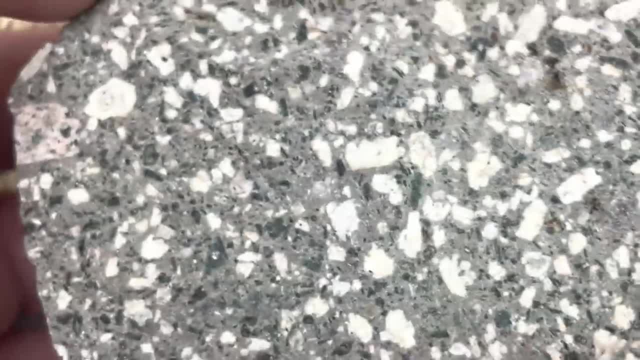 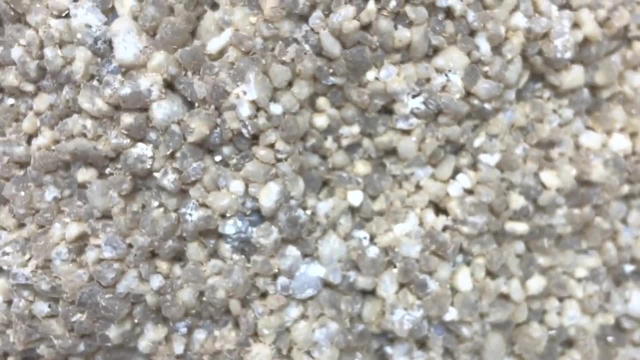 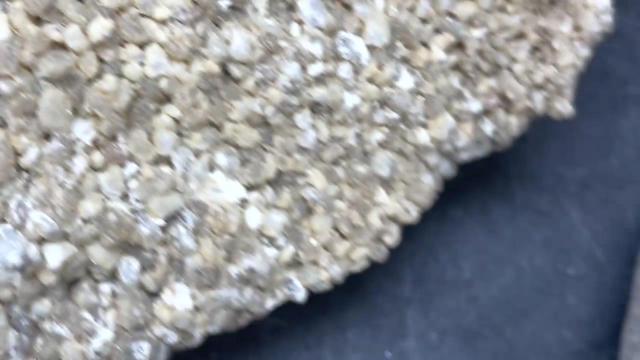 And so are you looking at crystals of minerals, as we are here, Or are you looking at grains, broken rock fragments that have just been glued together, as we have with this kind of pebbly sandstone, I suppose? So that would be a big criteria there is: what is, what is your rock actually made out of in terms of particles? 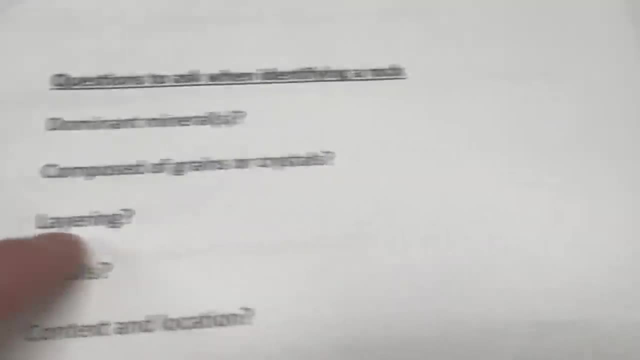 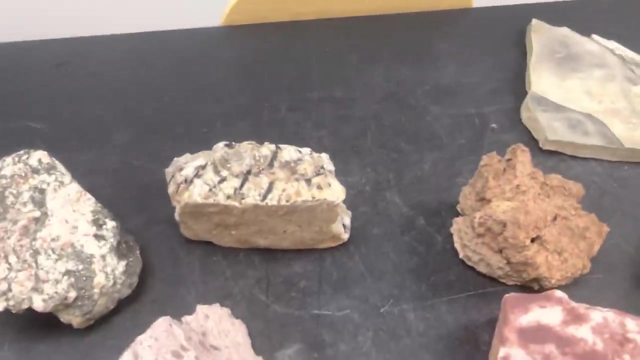 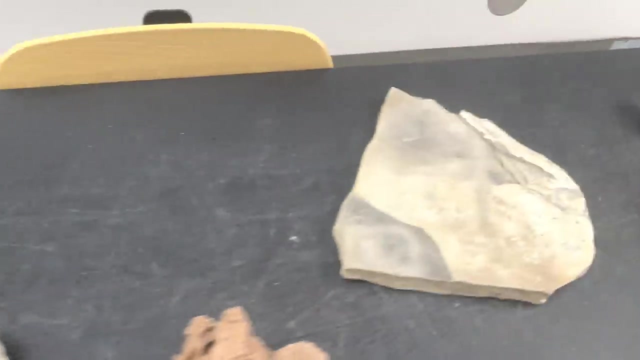 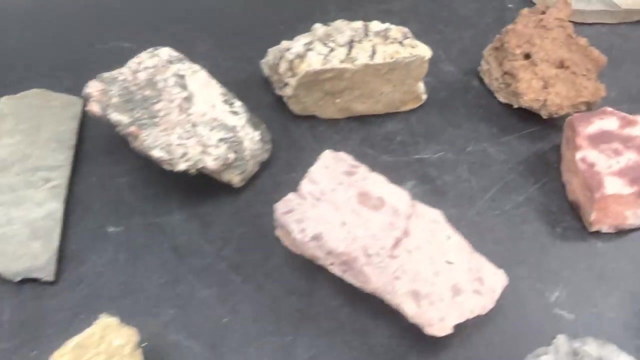 Does it have layering? If your rock has some layering to it, it's going to generally be a sedimentary or a metamorphic rock. A lot of times I just look at the way the rock presents itself right. So if it's just breaking off the slope into sheets like this or maybe something like this, that could be a big clue as to what kind of rock it is generally. 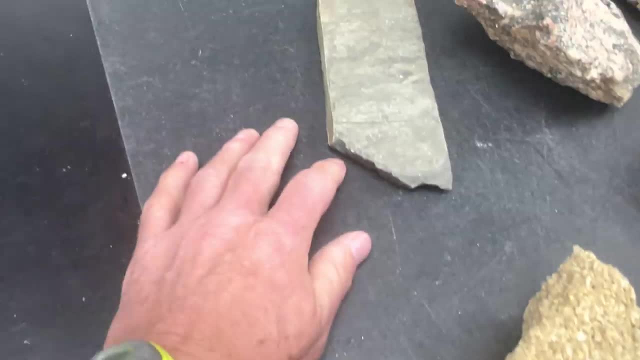 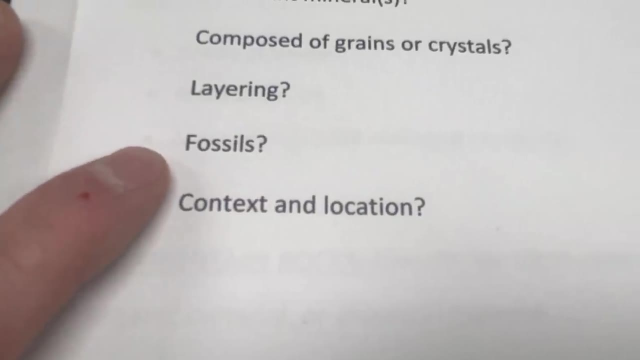 So there is a layering. And how thick are those layers? Are they really thin like these sheets here, Or is there? Is it more massive? Is it on like the tens of feet kind of scale fossils? What fossils do you have in the rock? 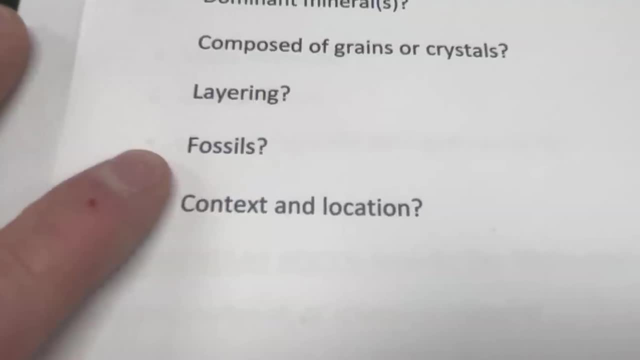 Because if you do, it's pretty much going to be sedimentary. There's a few instances, like an igneous rock, like tough, where you can get fossils in there. Sometimes some low grade metamorphic rocks preserve fossils, but they're often deformed. 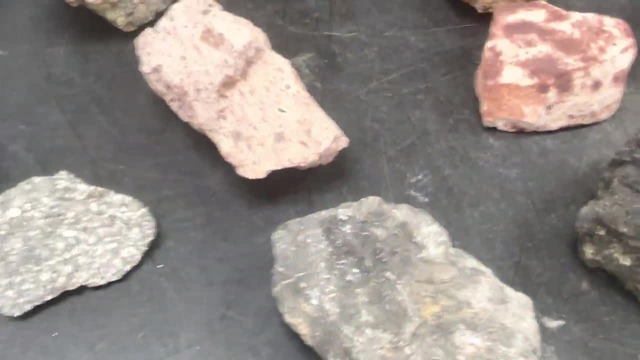 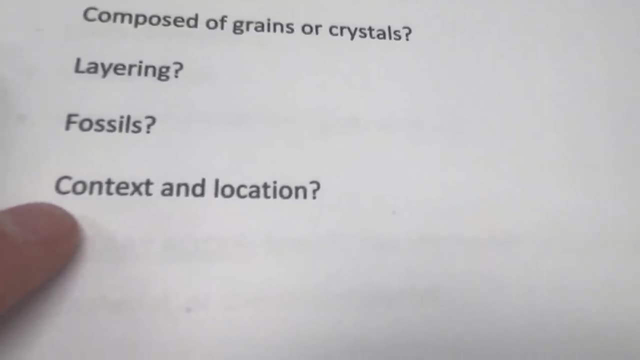 But fossils in your rock will indicate usually that you've got some sort of sedimentary rock. And then the last thing here is context and location. So where did you find it? Was it just like sitting on the shore, like next to the sidewalk on the shore, next to the trail? 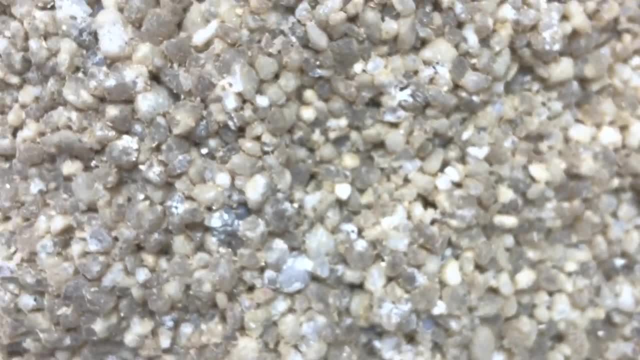 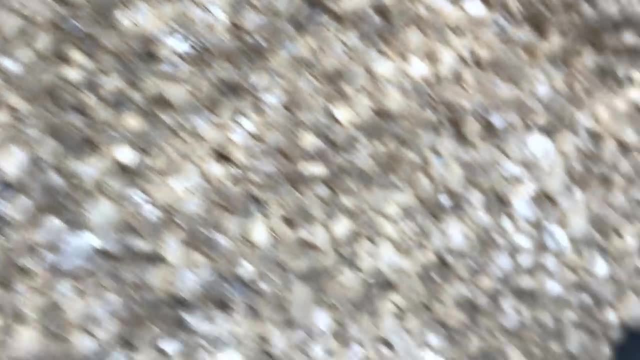 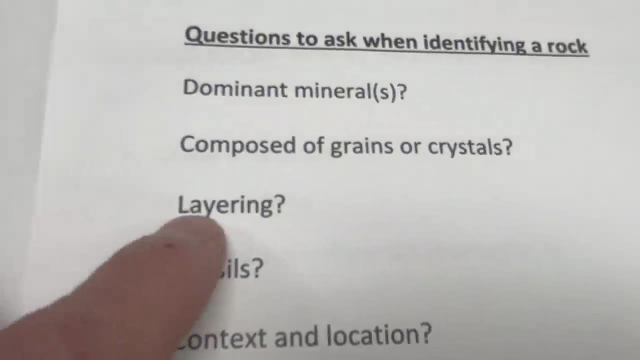 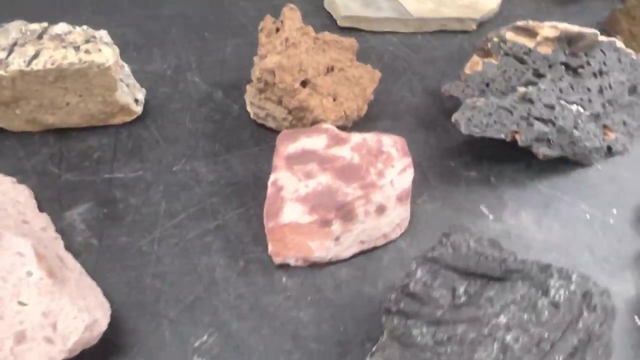 grains, broken rock fragments that have just been glued together, as we have with this kind of pebbly sandstone, I suppose. So that would be a big criteria. there is: what is your rock actually made out of in terms of particles? So if you have layering, if your rock has some layering to it, it's going to generally be a sedimentary or a. 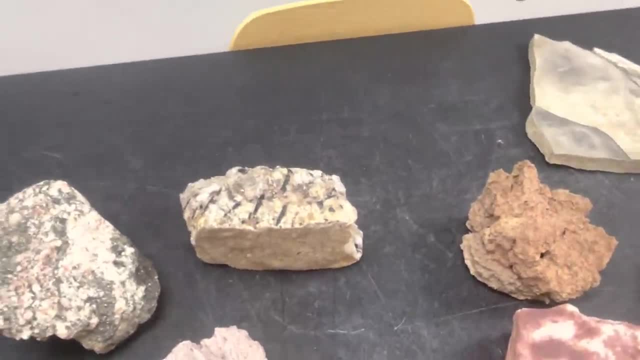 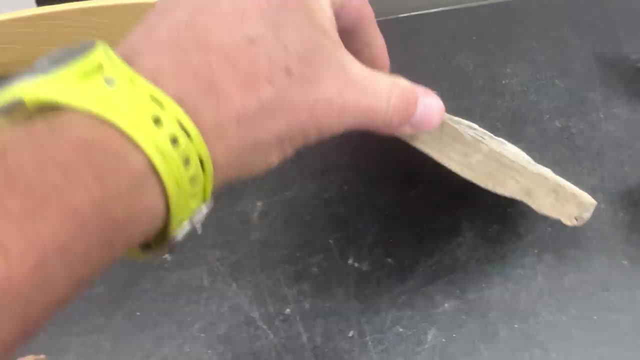 metamorphic rock. A lot of times I just look at the way the rock presents itself right. So if it's just breaking off the slope into sheets like this or maybe something like this, that could be a big clue as to what kind of 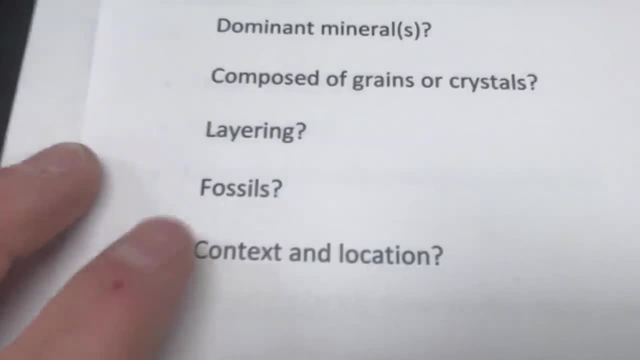 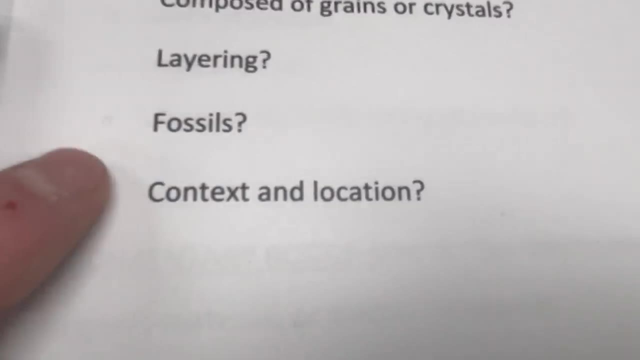 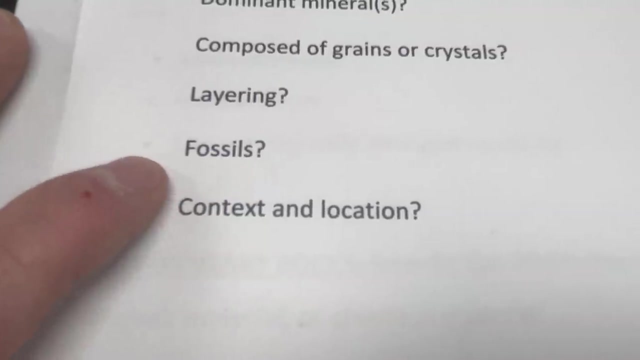 rock. it is generally So there is a layering. and how thick are those layers? Are they really thin like these sheets here, Or is it more massive? Is it on like the tens of feet kind of scale Fossils? what fossils do you have in the rock? Because if you do, it's pretty much going to be sedimentary. 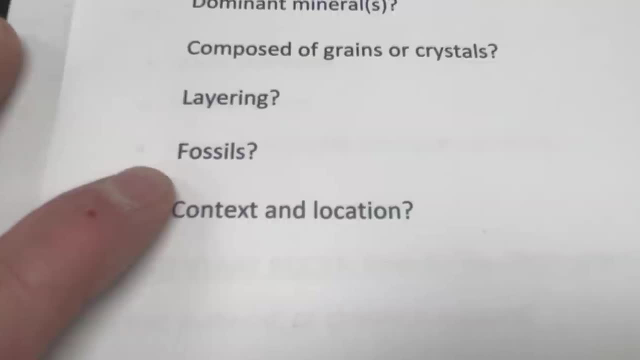 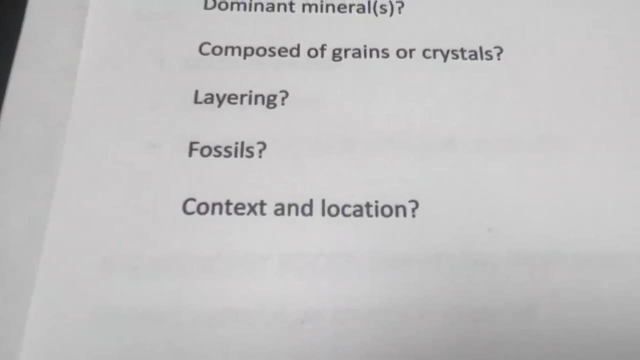 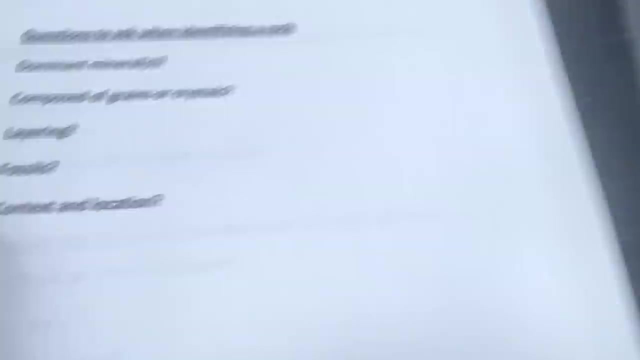 There's a few instances, like in igneous rock like Tuff, where you can get fossils in there. Sometimes some low-grade metamorphic rocks preserve fossils but they're often deformed. But fossils in your rock will indicate usually that you've got some sort of sedimentary rock. 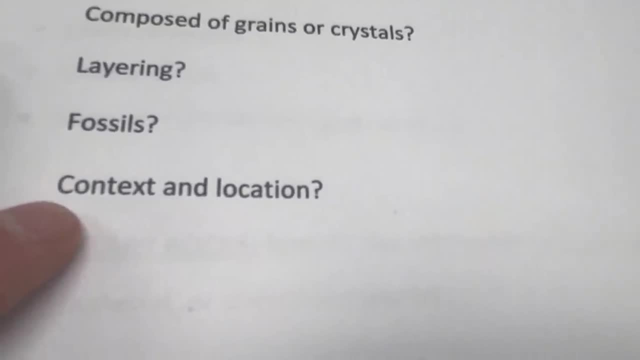 And then the last thing here is context And location. So where did you find it? Was it just like sitting on the shore, like next to the sidewalk, on the shore, next to the trail? Did you actually collect it from the base of the cliff? 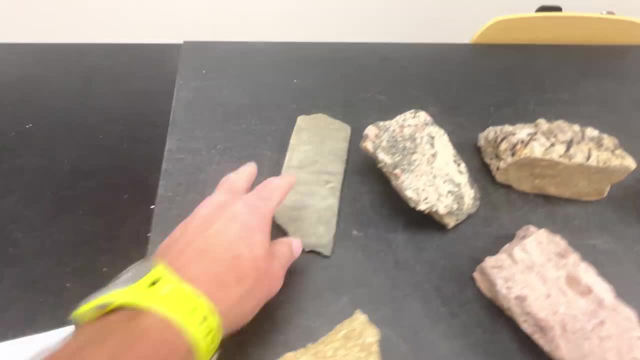 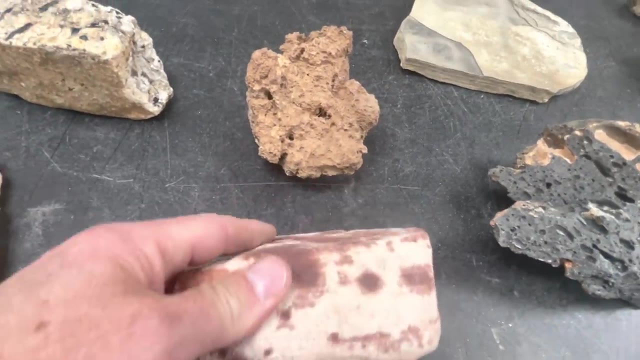 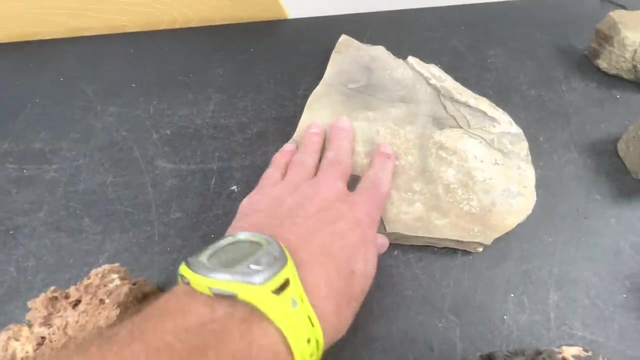 What kind of rocks were nearby? Maybe you have a flat rock like this or this and you don't know what it is, but you can see that it's occurring next to, let's say, a sandstone. And so if it's a sandstone and it's got, you've got this flat rock nearby. that's kind of fine grained. 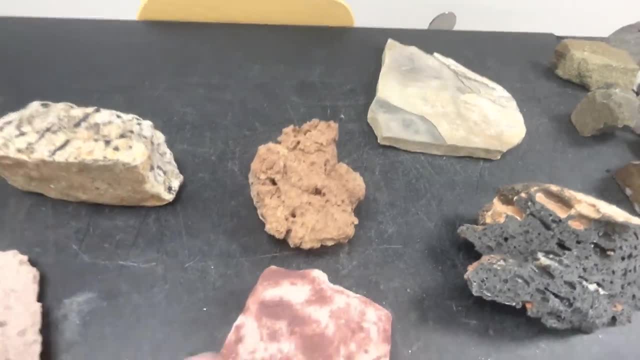 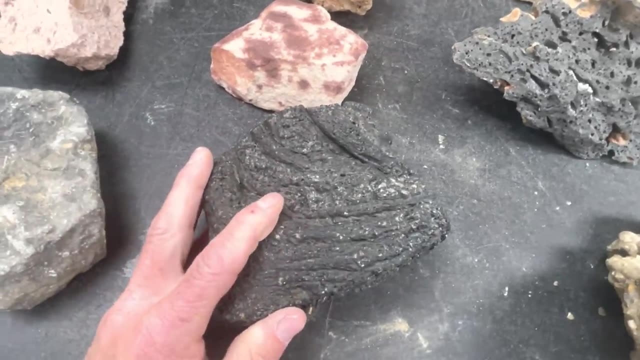 more likely than not, it's another sedimentary rock. It's another rock that makes sense in that type of environment. So think about the context and the location. Think about things like texture, right? So like, how is there any type of textures going on? 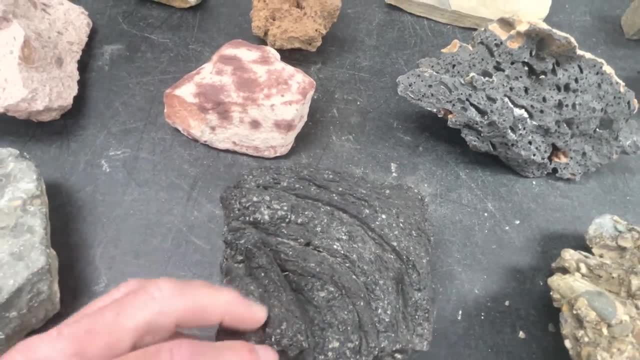 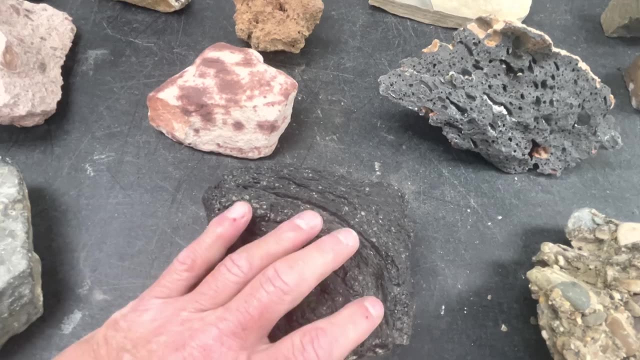 This has a flow texture to it. So this tells me that this material was either folded in this manner or maybe was somewhat plastic and elastic at some point in time- pliable if you will- And was able to sort of deform this way. 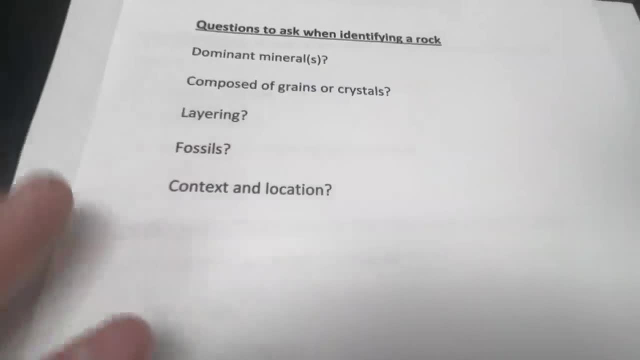 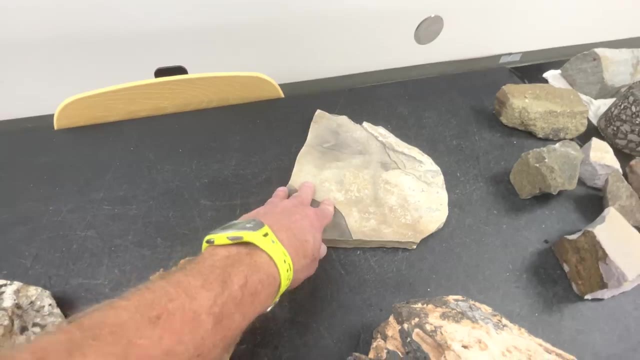 Did you actually collect it from the base of the cliff? What kind of rocks were nearby? Maybe you have a flat rock like this or this and you don't know what it is, but you can see that it's occurring next to, let's say, a sandstone. 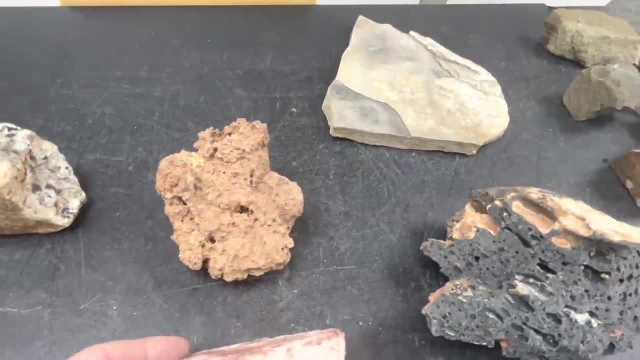 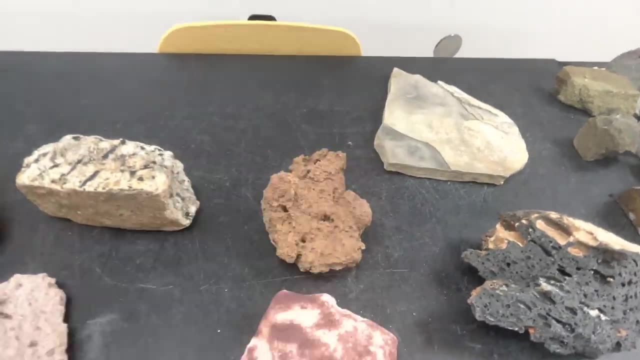 And so if it's a sandstone and it's got, you've got this flat rock nearby. That's kind of fine grained. More likely than not, it's another sedimentary rock. It's another rock that makes sense in that type of environment. 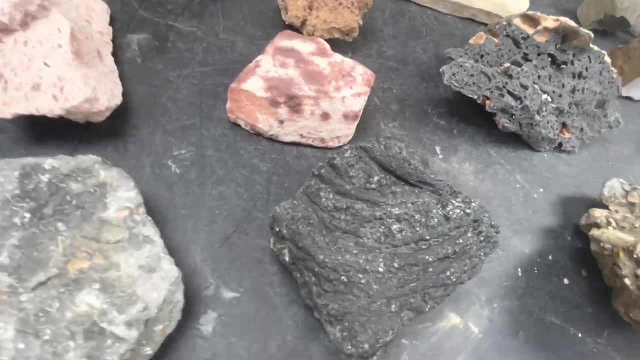 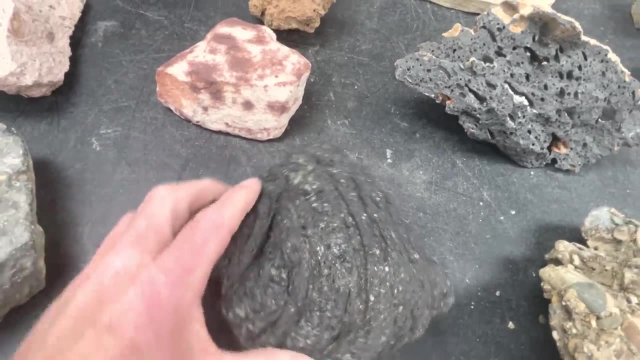 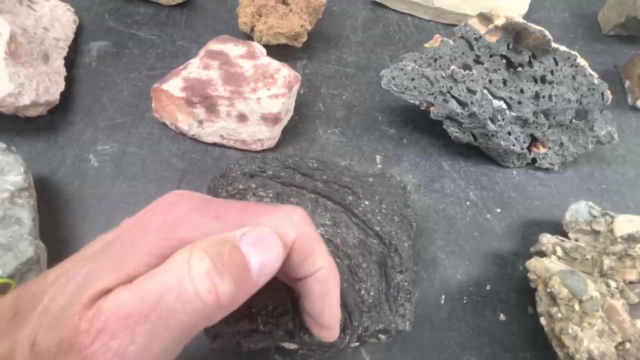 So think about the context and the location. Think about things like texture, Right. So like, how is there any type of textures going on? This has a flow texture to it. So this tells me that this material was either folded in this manner or maybe was somewhat plastic and elastic at some point. 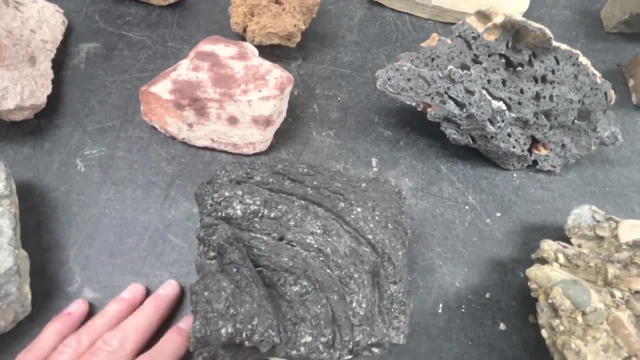 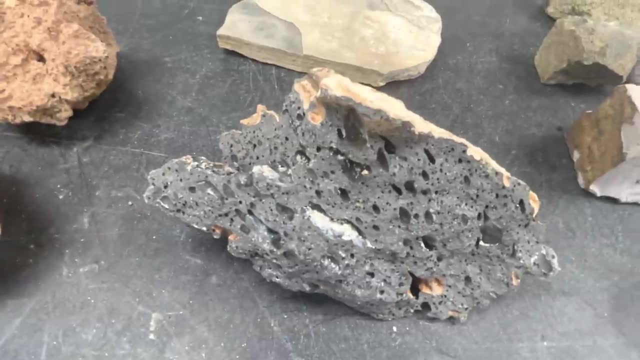 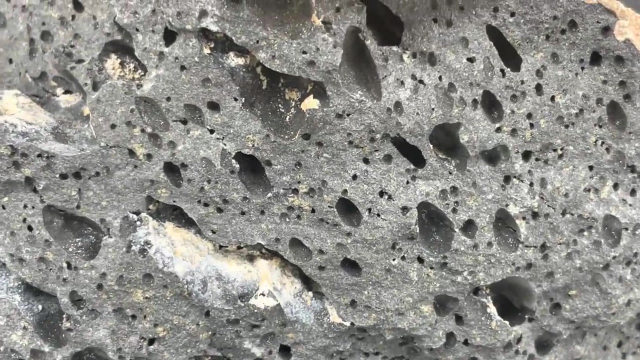 In time, pliable if you will, and was able to sort of deform this way. This is a piece of basalt with some some ropey pahoehue lines here. Holes in rocks- Another thing that people kind of focus on: just because we have holes in rocks doesn't mean that they're automatically gas bubbles, or what we call vesicles. 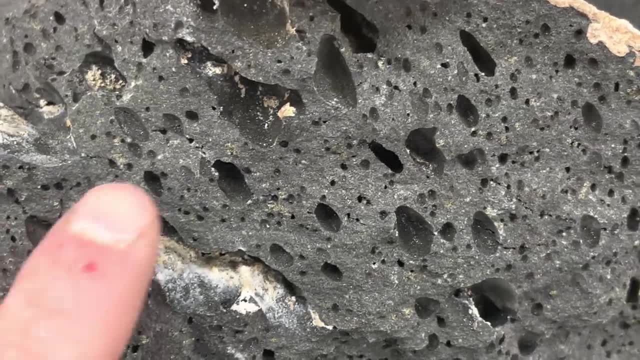 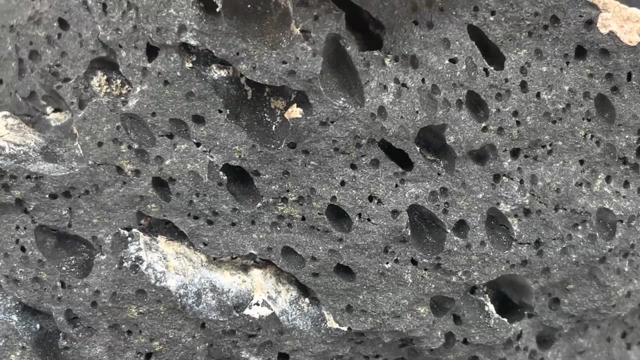 There's plenty of instances where organisms can make burrows in rocks, So that might be what's going on. Or it could be that the rock has some mineral. Some mineral has dissolved out of the rock, leaving some voids behind, So that's something to think about as well. 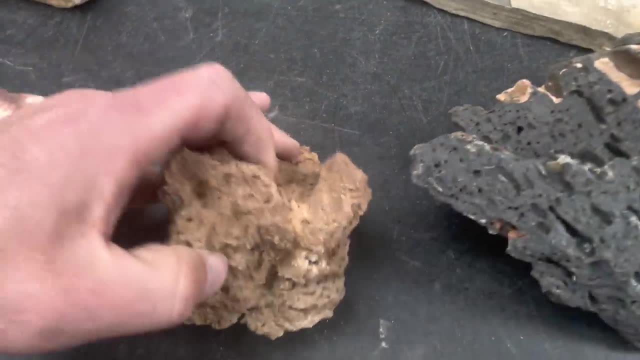 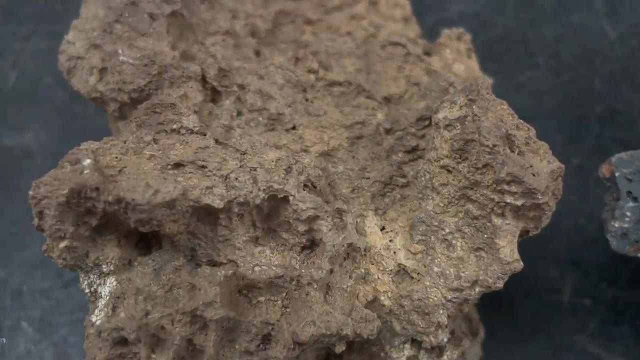 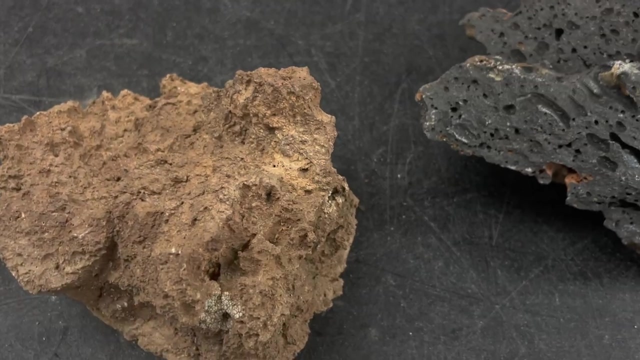 This would be a good example here. We've got holes in this rock as well. I can zoom in on this one if I can. There we go. This one's also kind of porous. Kind of looks like if you didn't know anything else about it. again, context is removed. 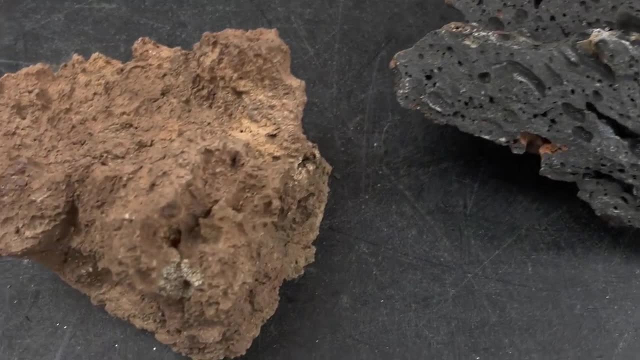 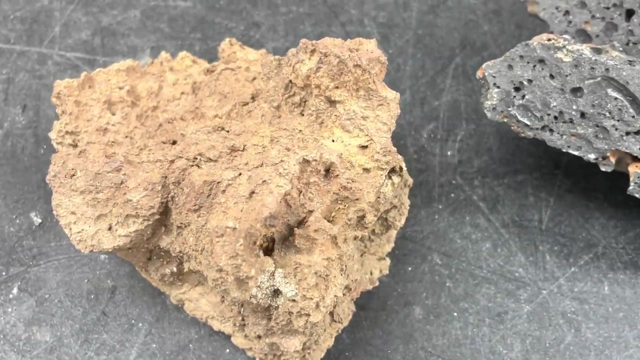 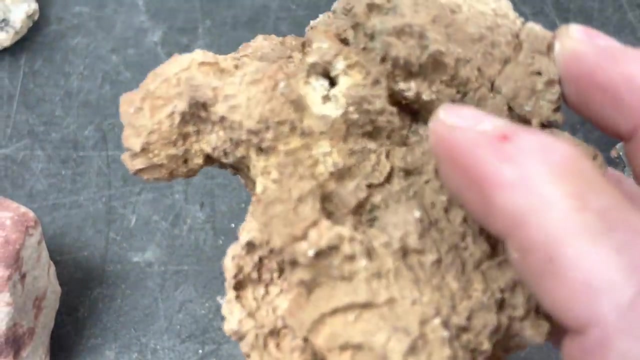 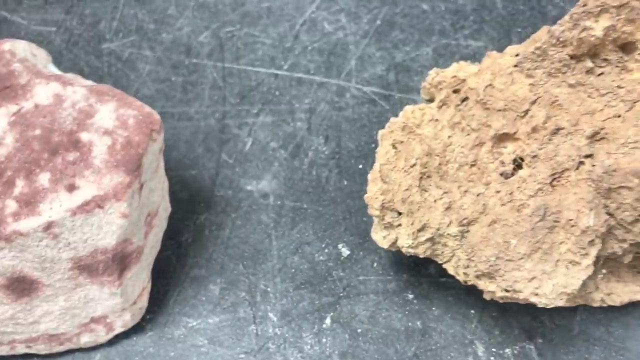 This is the hardest part of teaching geology in the classroom. I'm just handing these students these little samples, fist-sized samples of rocks, and there's no context. They're just looking at a rock all by itself. But in this case, here this rock, even though it's quite sharp and it does have some holes in it in places, the big key to give away this one is again looking at the mineral composition. 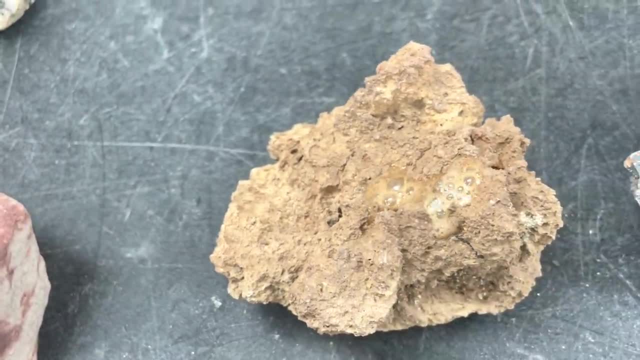 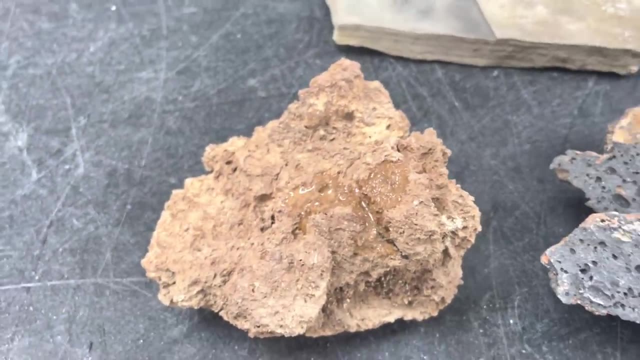 So if we hit it with acid or if you have vinegar at home, that will work too. This rock is totally made out of calcite, So it's a type of limestone. It's a type of limestone called tufa or travertine. 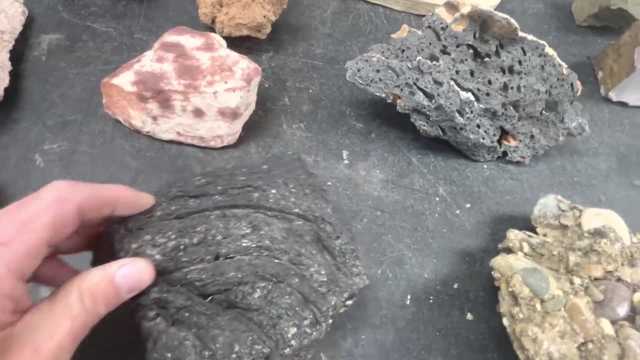 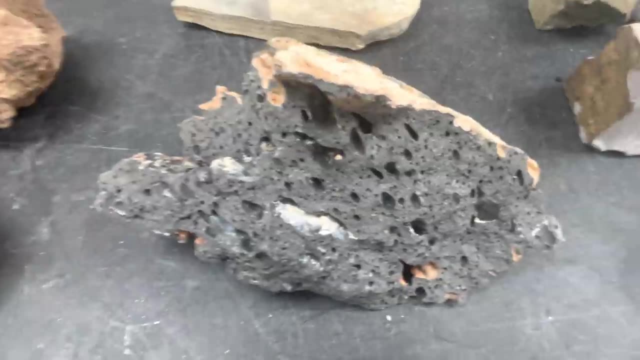 This is a piece of basalt with some some ropey pahoehoe lines here. Holes in rocks- Another thing that people kind of focus on: just because we have holes in rocks doesn't mean that they're automatically gas bubbles, or what we call vesicles. 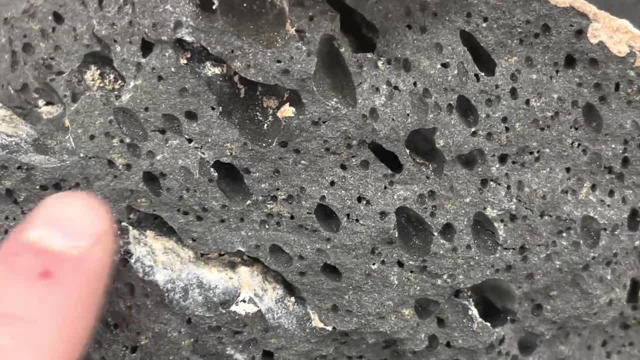 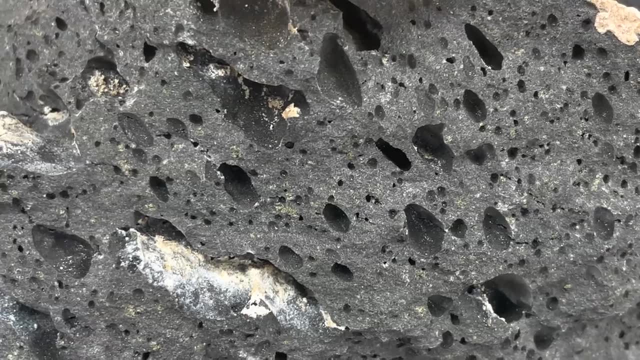 There's plenty of instances where organisms can make burrows in rocks, So that might be what's going on. Or it could be that the rock has some mineral has dissolved out of the rock, leaving some voids behind, So that's something to think about as well. 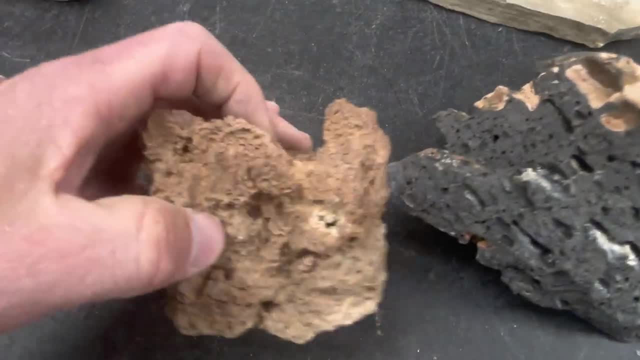 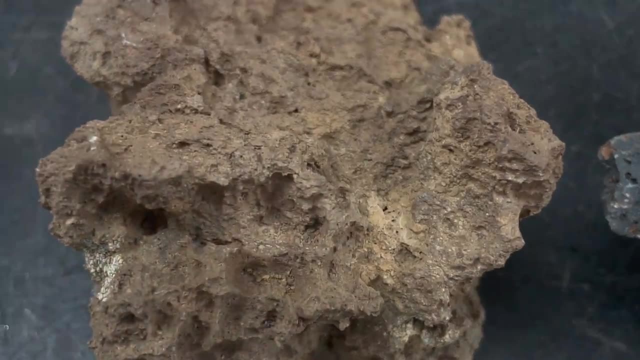 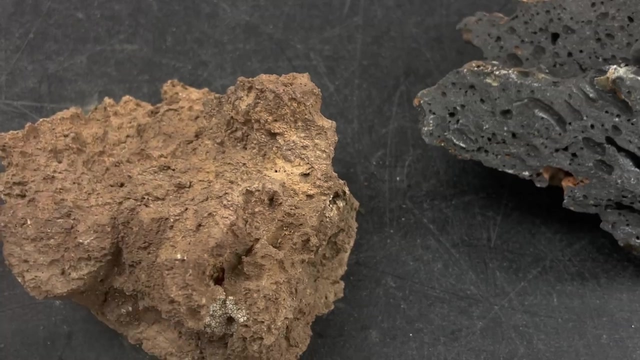 This would be a good example here. We've got holes in this rock as well. I can zoom in on this one if I can. There we go. This one's also kind of porous. Kind of looks like if you didn't know anything else about it. again, context is removed. 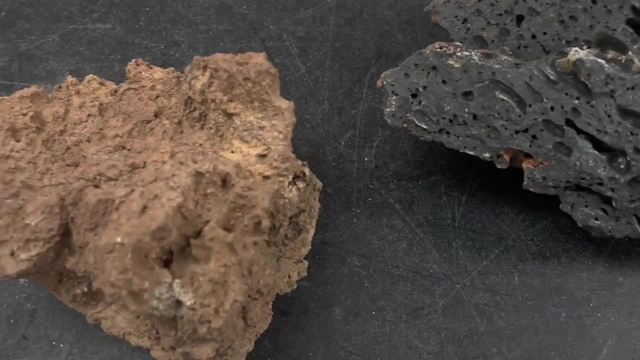 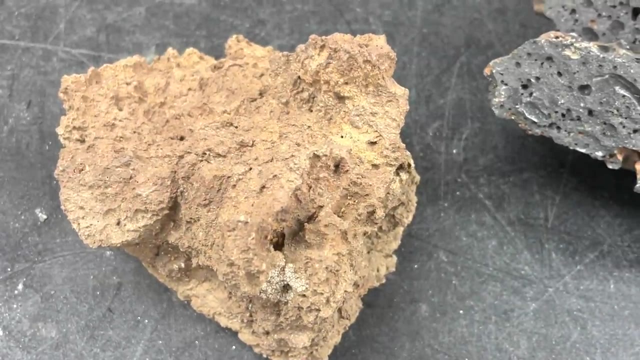 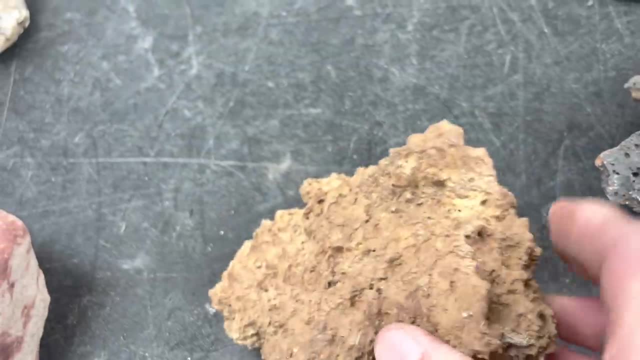 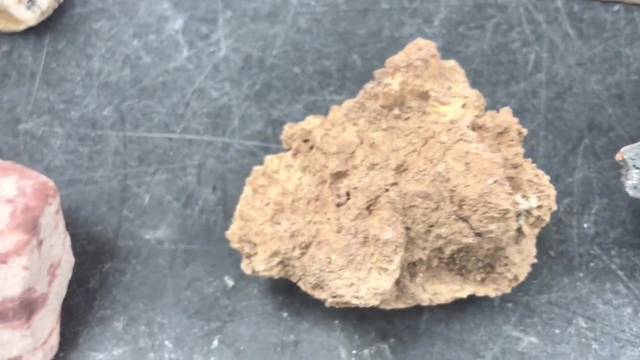 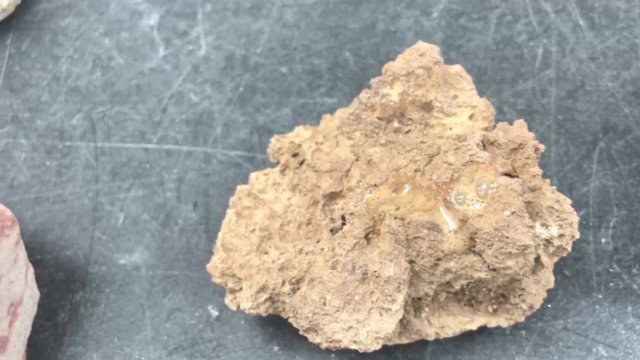 But in this case, here, this, this, this rock, even though it's quite sharp and it does have some holes in it in places, the big key to give away this one is again looking at the mineral composition. So if we hit it with acid or if you have vinegar at home, that will work too. 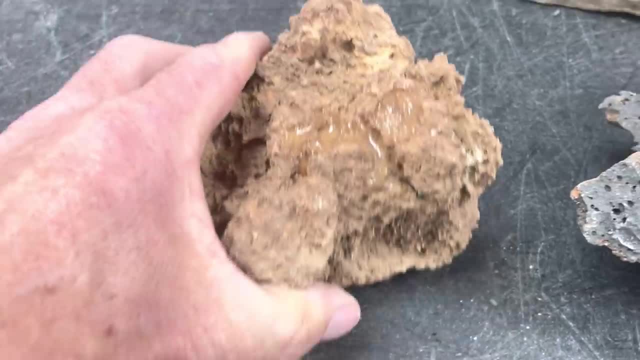 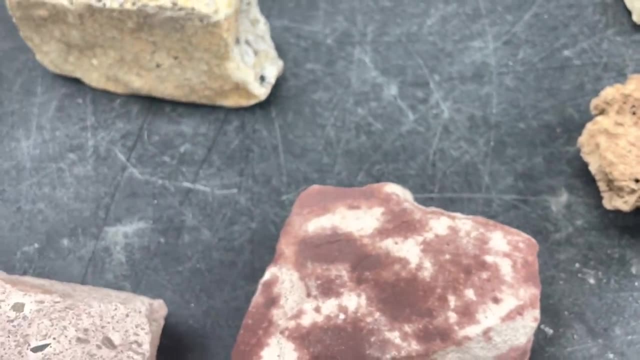 This rock is totally made out of calcite, So it's a type of limestone. It's a limestone type of limestone called tufa Travertine. We'll get to that later. Let's see what else. Yeah, Particles in the rock. 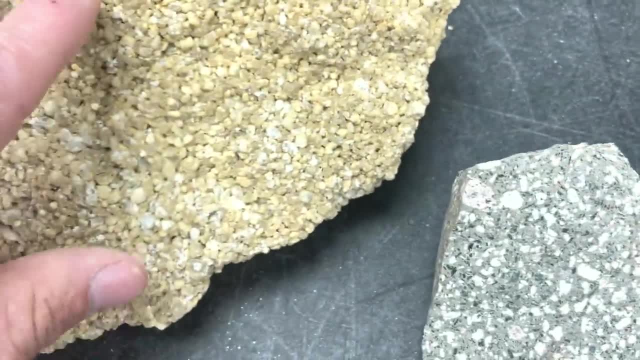 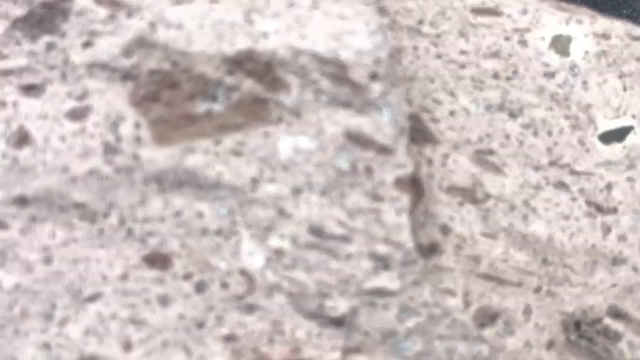 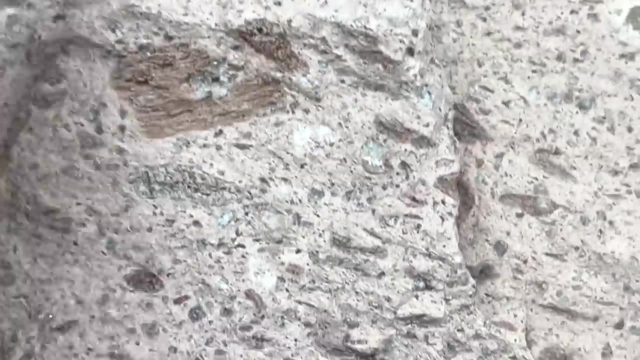 What are the particles? This is an interesting one. here We looked at these two grains and crystals. This rock is kind of interesting because if you look at it closely you'll see that it does have big particles in it, Angular particles. But as we kind of rotate it in the light, it looks like there's one there, maybe one over here. 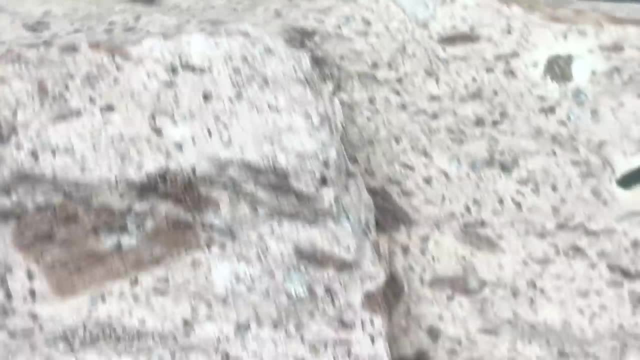 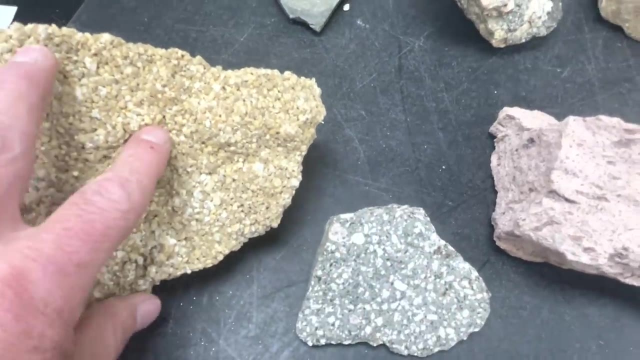 You can see some shiny little surface, And so there's crystals in here. So this is a rock that actually kind of has properties of both of these. It has crystals in it, but it also has some fragments or grains as well. This is a piece of tufa, volcanic tufa. 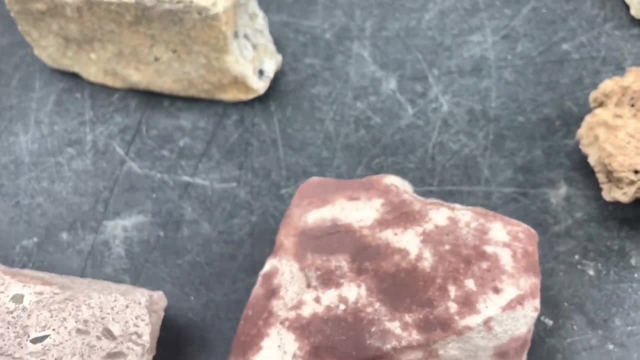 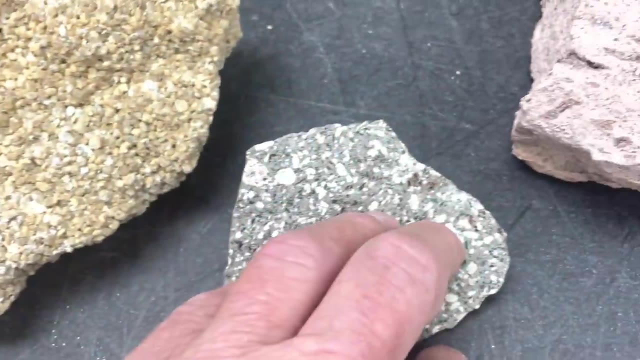 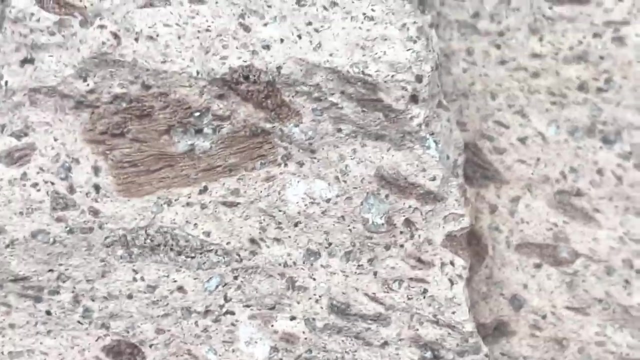 We'll get to that later. Let's see What else. Yeah, particles in the rock. What are the particles? This is an interesting one. here We looked at these two grains and crystals. This rock is kind of interesting because if you look at it closely you'll see that it does have big particles in it: angular particles. 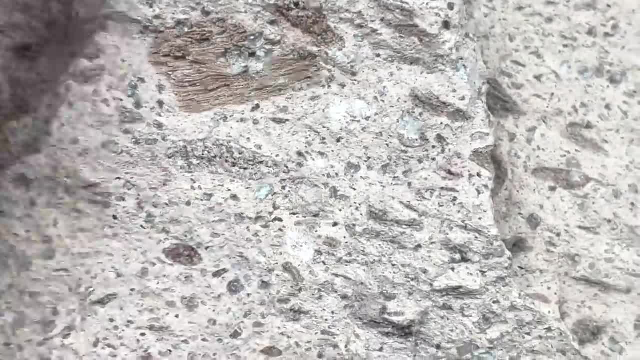 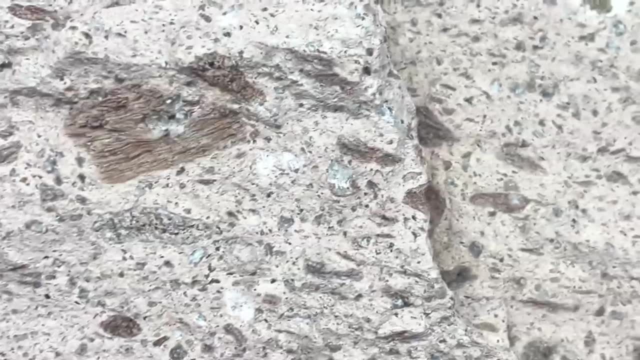 But as we kind of rotate it in the light, it looks like there's one there, Maybe one over here. You can see some shiny little surfaces as well, And so there's crystals in here. So this is a rock that actually kind of has properties of both of these. 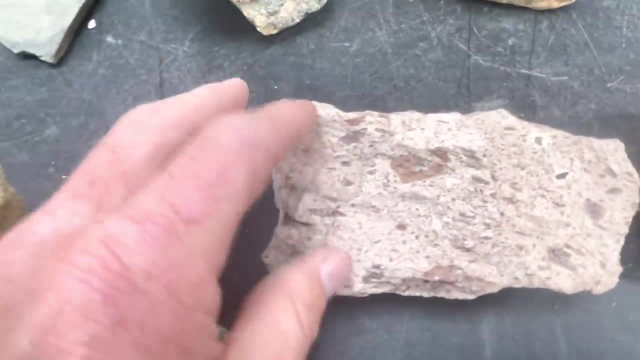 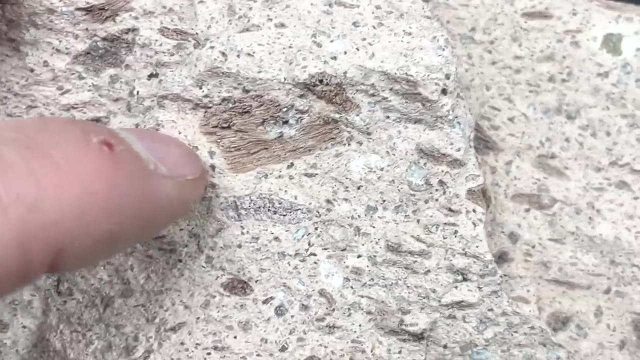 It has crystals in it, but it also has some fragments or grains as well. This is a piece of tufa, volcanic tufa, So it makes sense for it to have crystals, But it also in a big, powerful volcanic eruption. you might be ripping up other particles, volcanic particles or rocks. 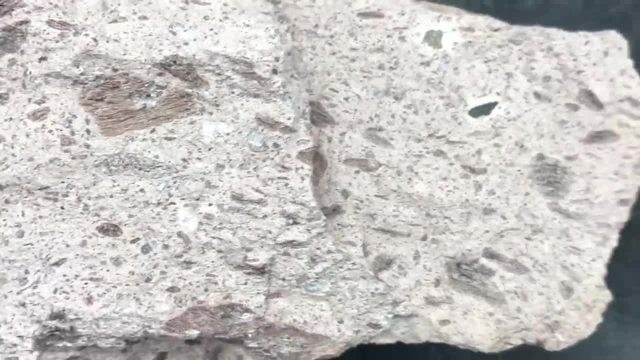 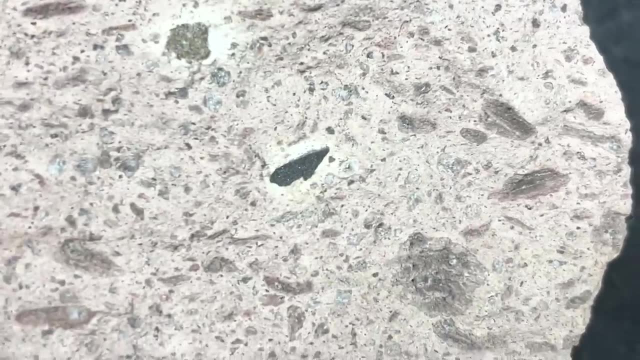 And those can get encased in there And those can get encased in it as well, And that's why we have these angular particles. Notice also here that we've got some particles that have kind of a halo around them. There's actually a discoloration around the particles themselves. 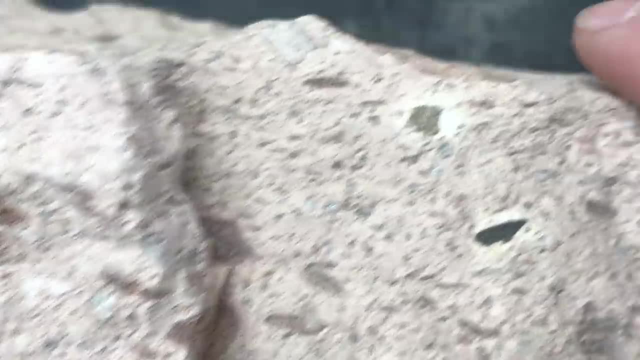 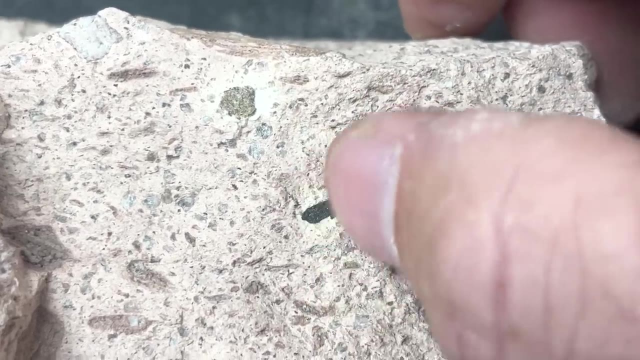 That suggests in this case, now that we kind of know this is a tufa and this is a volcanic rock- that these particles were maybe cooler, had a different temperature than the hot ash, And so there's kind of a thermal alteration effect going on around these. 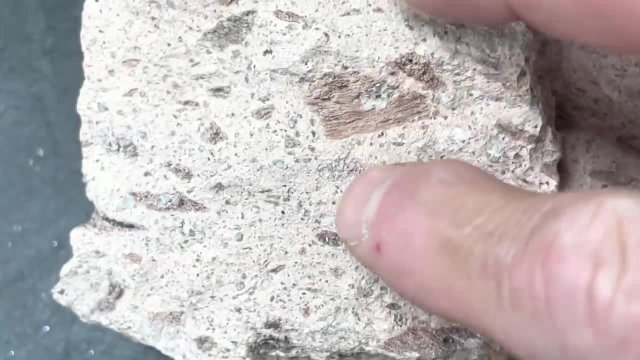 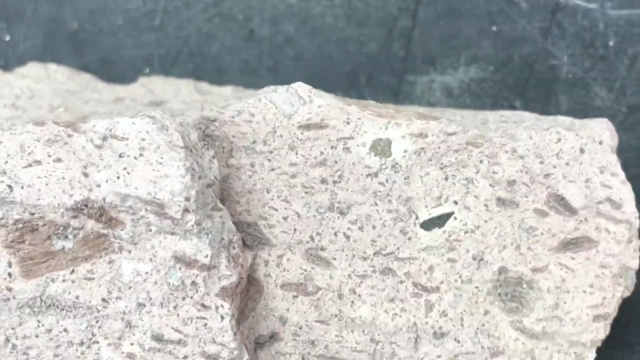 These little rock particles in there- Presumably the other particles- like that's a pumice- are particles that were already at high temperatures And so you don't see that little kind of thermal halo effect there. So yeah, big crystals. 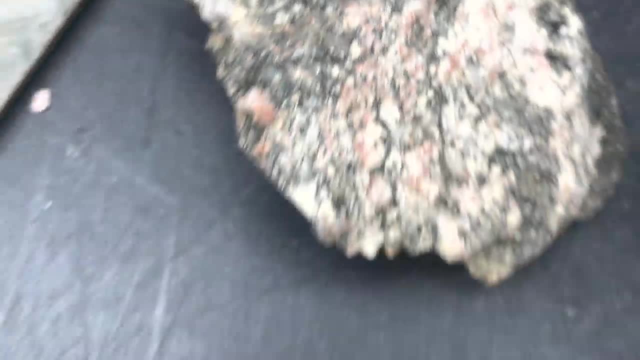 Yeah, again, is it made out of crystals? What do you see when you look at the rock? Those are all just good things there. I'm going to kind of wrap up. I might have went too far there. Oh, last one here. 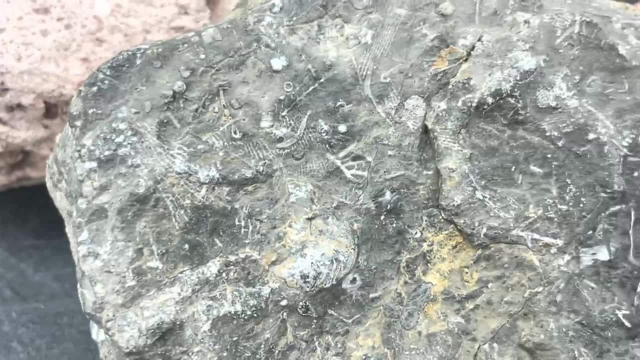 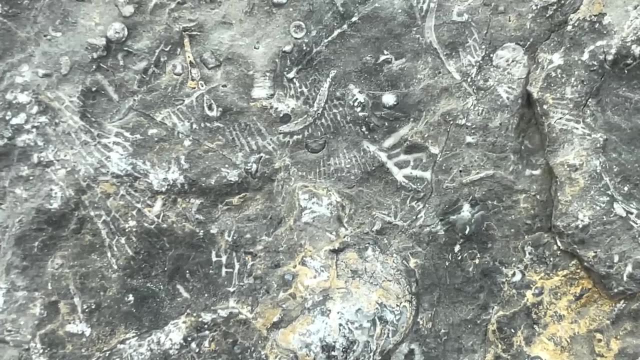 This one has, if we look at it closely. look for patterns. A lot of people think they have fossils just because there's an interesting shape or they're trying to project. you know, I've had people tell me that they think there's a fossilized snake eating a squid in the rock. 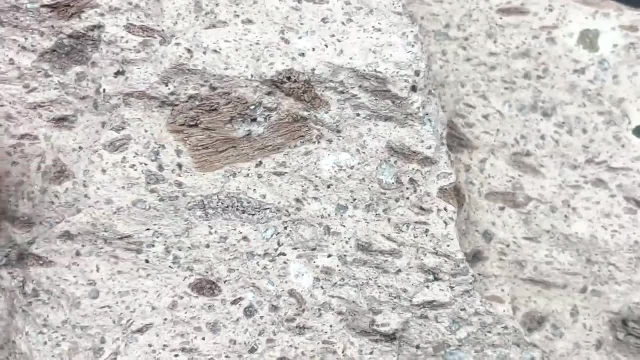 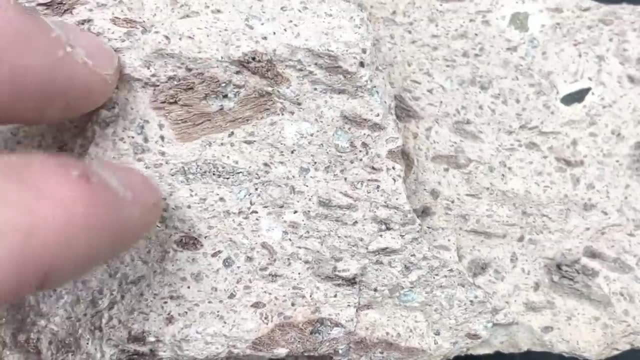 So it makes sense for it to have crystals, But it also in a big, powerful volcanic eruption you might be ripping up other particles- volcanic particles or rocks- And those can get encased in it as well, And that's why we have these angular particles. 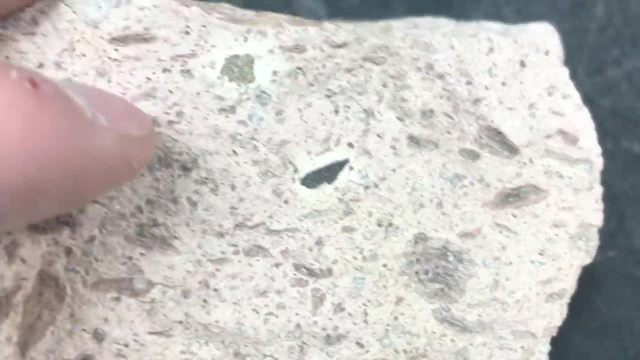 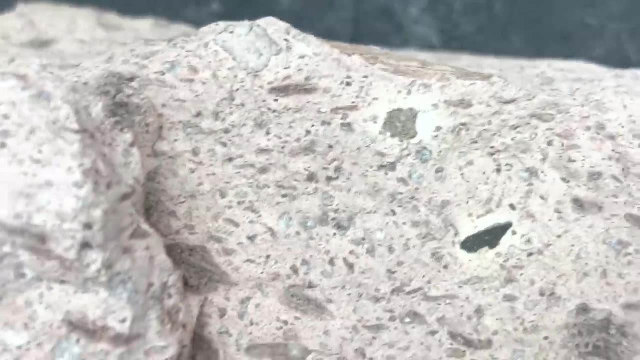 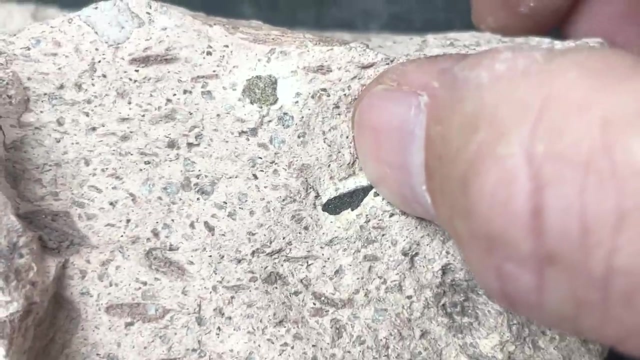 Notice also here that we've got some particles. They have kind of a halo around them. There's actually a discoloration around the particles themselves That suggests, in this case, now that we kind of know this is a tufa and this is a volcanic rock, that these particles were maybe cooler, had a different temperature than the hot ash. 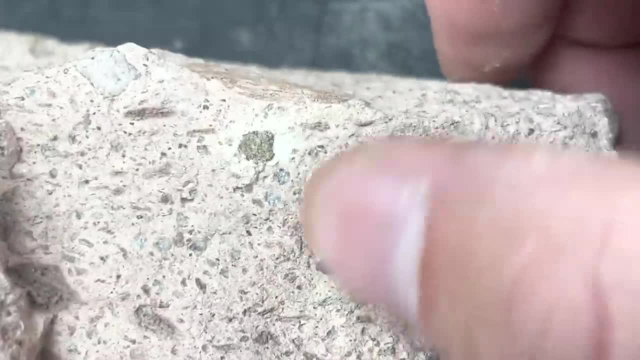 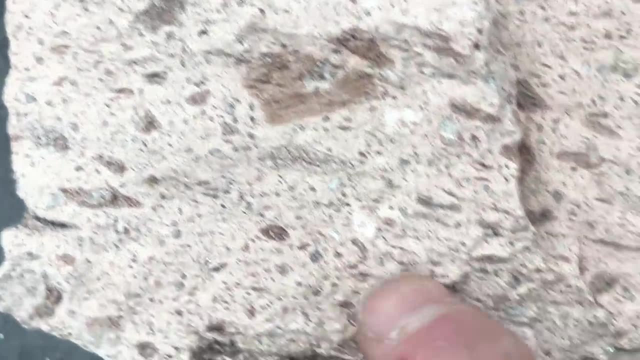 And so there's kind of a thermal alteration effect going on around these little rock particles in there. Presumably the other particles- like that's a pumice Right- Are particles that were already at high temperatures And so you don't see that little kind of thermal halo effect there. 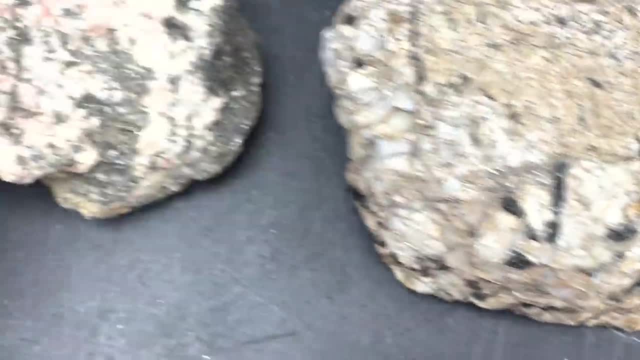 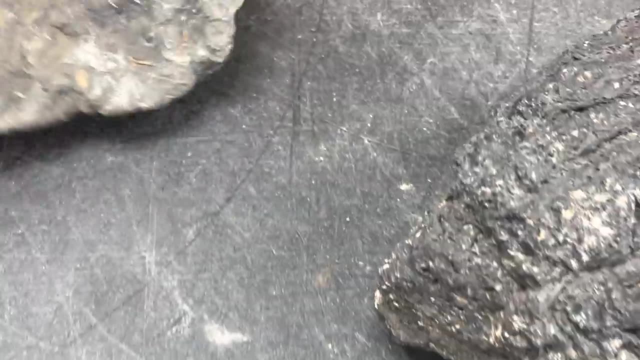 So yeah, big crystals, Yeah, again, is it made out of crystals? What do you see when you look at the rock? Those are all just good things there. I'm going to kind of wrap up. I might have went too far there. 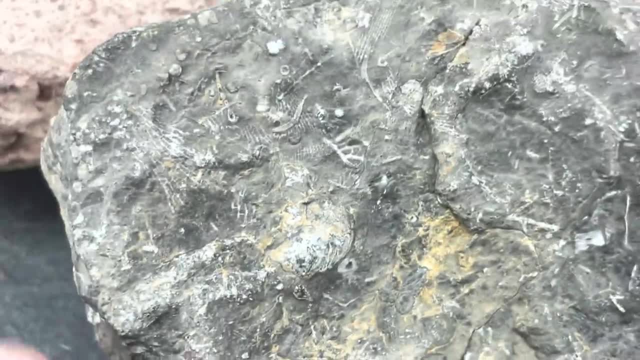 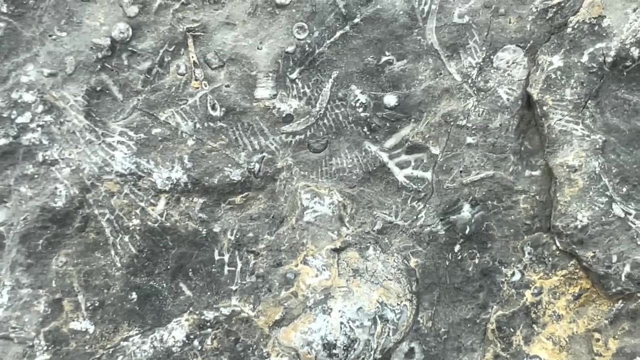 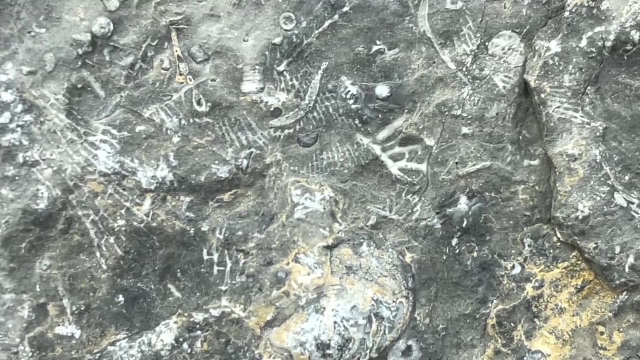 Oh, last one here. This one has, if we look at it closely, look for patterns. A lot of people think they have fossils just because there's an interesting shape Or they're trying to project. You know, I've had people tell me that they think there's a fossilized snake eating a squid in the rock and just all kinds of stuff that just doesn't even make sense. 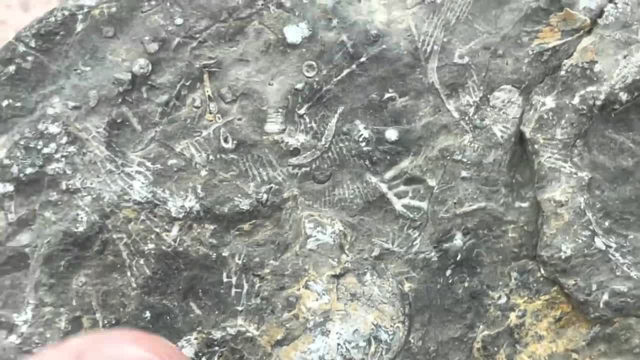 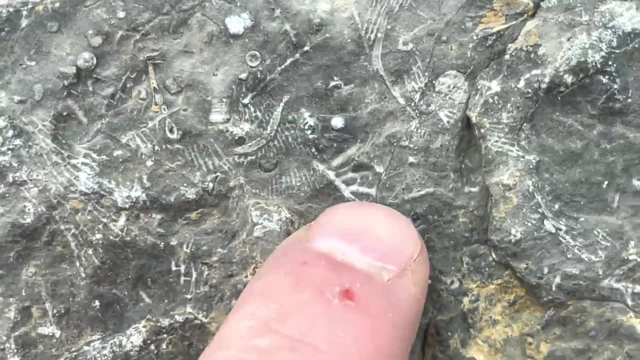 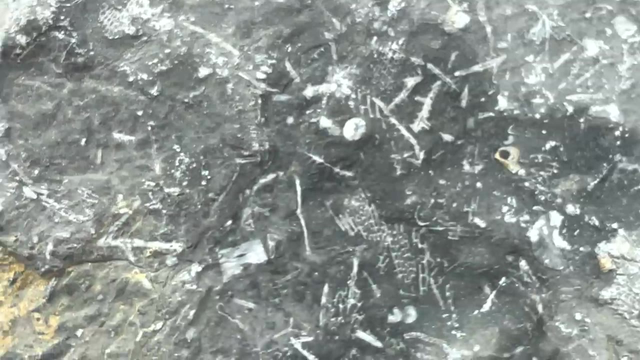 It might be good- And maybe we'll do another video series on these- is to look at some common fossils And so these little kind of cheerio looking things, these web shaped materials in here, these branching things Generally, if it looks, if you see geometric patterns and it looks organic, it very well could be a fossil. 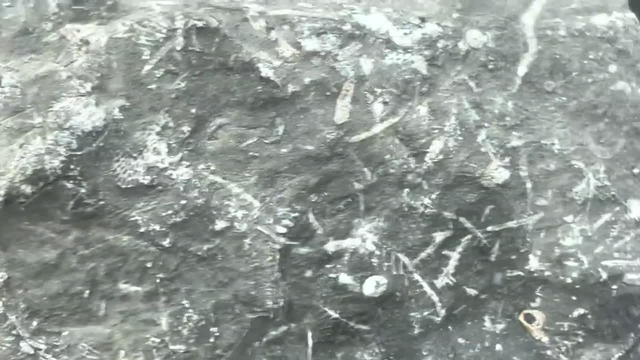 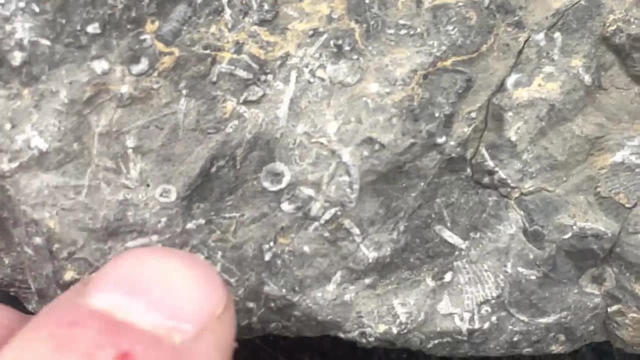 But I guess what I'm trying to say is, If you familiarize yourself with the different types of especially invertebrate fossils that can be found in rocks, that will help you identify the fossils that much better. This is a piece of limestone with crinoids. 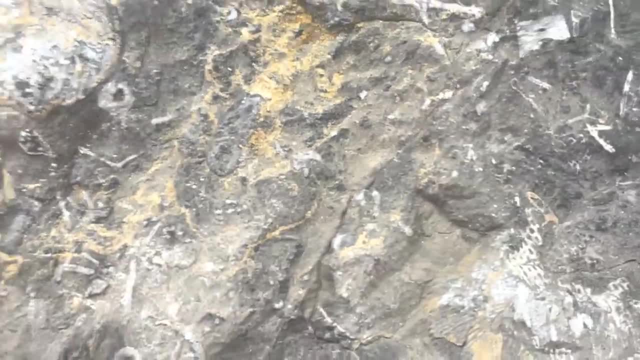 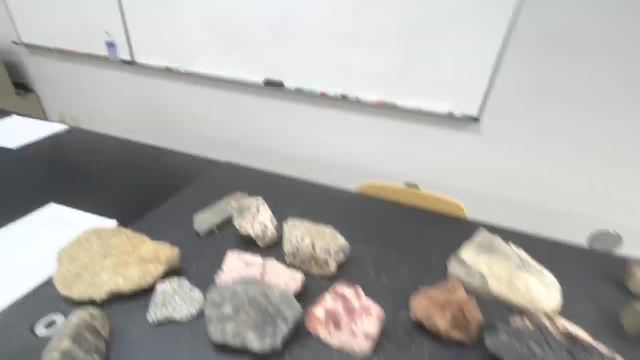 These are called bryozoans. Could be a little bit of coral material in here as well, And this is just a nice piece of of limestone here, So hopefully that was helpful. The idea was that would be a nice little primer, Nice little introduction.